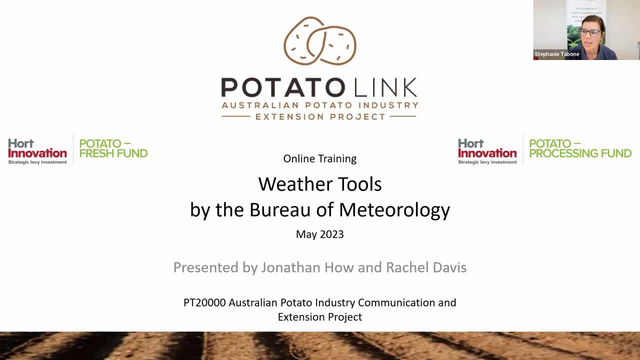 Jonathan has worked across multiple Bureau offices and teams in diverse roles, ranging from aviation, forecasting severe weather and, most recently, media and communications. Prior to the Bureau, Jonathan worked as an Economic Consultant with the Regulation and Policy Team at EY. Jonathan brings a genuine interest and passion to his new agriculture team as it seeks to help. 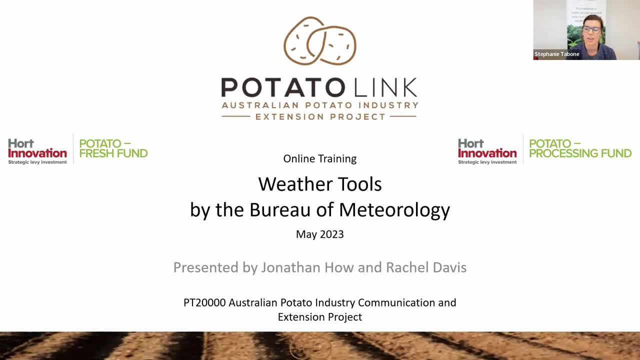 growers make critical farming management decisions in a changing climate. He holds a Bachelor of Science majoring in Meteorology and Mathematics, and also a Bachelor of Commerce majoring in Economics from Monash University and is also a Graduate Diploma in Meteorology. So we welcome Jonathan and his experience to our session today With us also Rachel Davis. 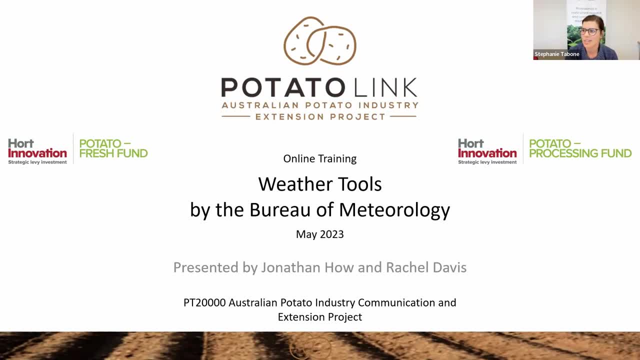 who is a Certified Practicing Agriculturalist with 20 years experience in horticulture and supply chains. She is currently the Agriculture Segment Lead at the Bureau of Meteorology to support Australia's horticulture, sugar and wine segments. Her experience in post-farm gate. 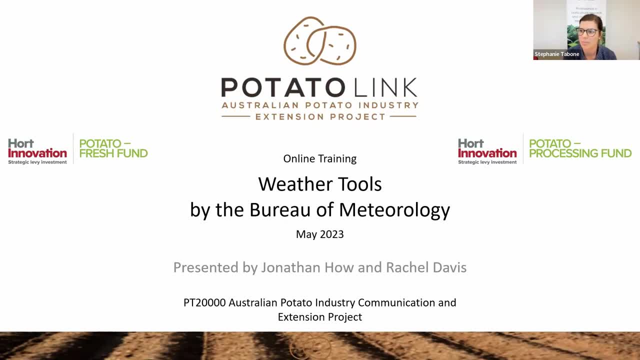 supplies is being utilised as she builds the Bureau's engagement and relationships across the sector to boost the Australian economy. Rachel's passions are environmental sustainability, sustainability and reducing food waste. She also holds a postgraduate degree in agribusiness from the University of Queensland and is also a Director of the International Fresh. 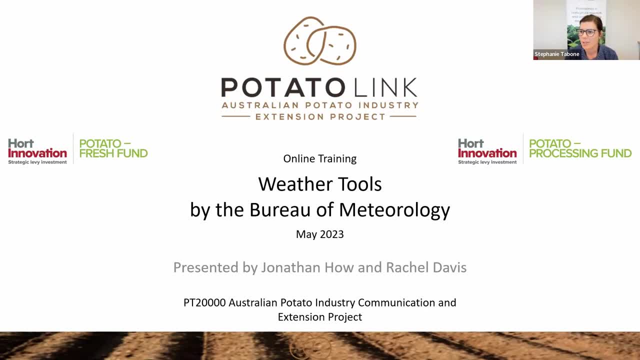 Produce Association. With us also on the line, we have Peter O'Brien, who is a valued member of the Potato Link team and the National Coordinator for the project, bringing also many years of experience working in horticulture and the potato industry. So welcome our guest. 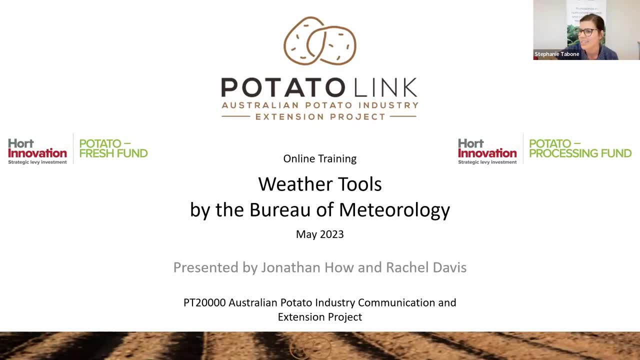 today and Peter O'Brien, And look forward to having the training session with you all. So I just wanted to give a brief introduction. The Bureau of Meteorology has an incredible source of weather data available and I think it would. it would be crazy not to utilise these resources that. 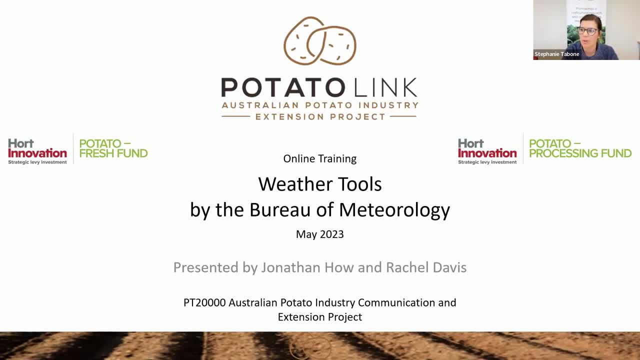 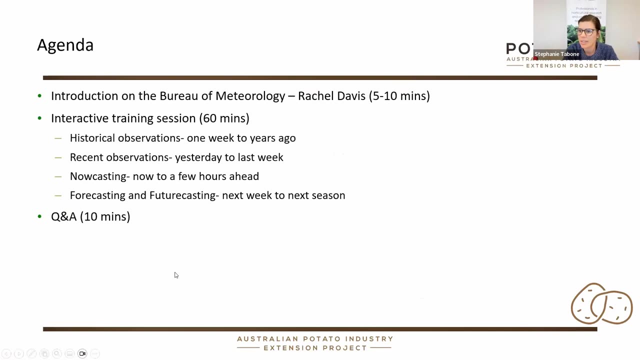 are free to people, And the goal today is to help growers and other industry representatives learn the most about what the Bureau has to offer, how you can navigate the resources available and where you might use them best in your operations. So in today's online training on our agenda, Rachel is going to provide a brief introduction. 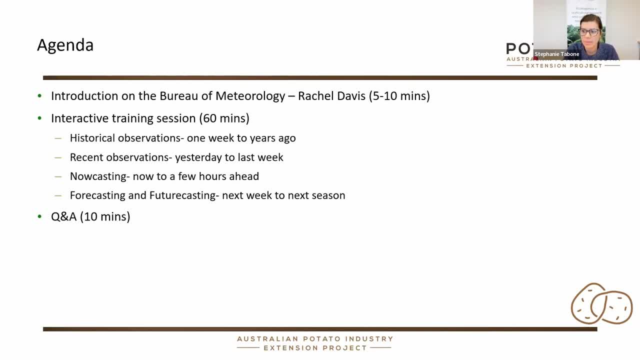 to the Bureau of Meteorology outlining some of their team's objectives and some other climate tools that we probably won't have time to cover today, but just for your awareness, so you can access them in future. And then we're going to jump straight into the training interactive session. 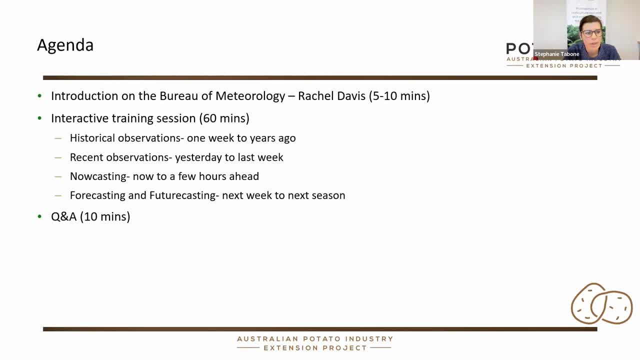 with Jonathan, And Jonathan is going to be covering a few different segments in which we'll hear more about shortly and also hear your input on which you'd like to hear most about during today's session. But essentially, looking at historical observations, what are the most recent observations? 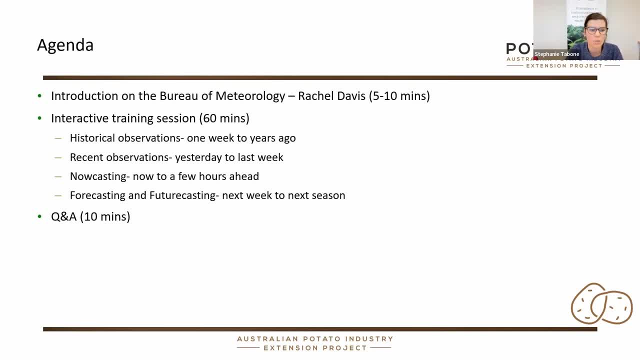 what is happening now in weather and then also tools for forecasting. It could be from a range of next week to next season, So that will cover the majority of our session and then we'll have a Q&A- more formal Q&A- at the end, but we will be taking questions after each of the different tools. 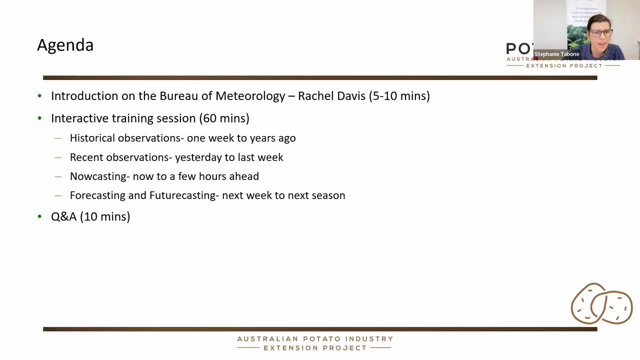 are covered. In terms of housekeeping, I mentioned before. we are recording this session. We will be sharing screens. You do have the ability to come off mute and turn your video on, so I mean, feel free to do so if you'd like to raise your hand for a question. Alternatively, it would be best to, I think. 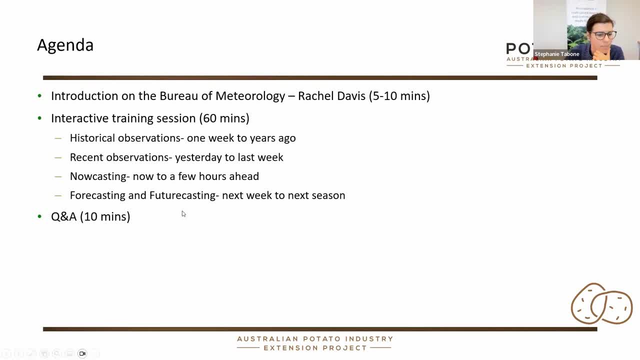 keep your camera off while Jonathan's presenting, just to keep everything streamlined and focused. And we also have a worksheet that we will paste a link in the chat for you now that you can follow along with, And the purpose of today is to try and keep it interactive, So you're welcome to try. 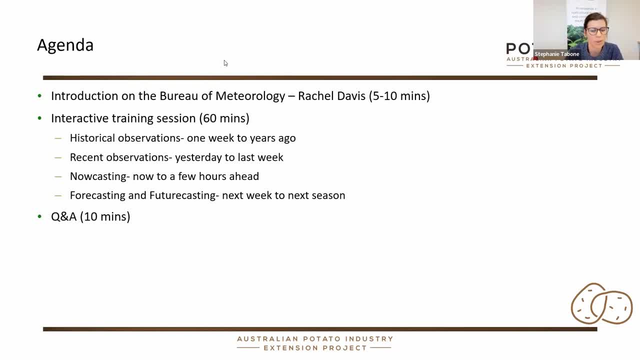 and follow along and access the tools as we go through it, or you're welcome just to follow Jonathan's screen and access it at a later time, as you have the worksheet as reference. So with that, I think that's most of the intro I'm going to hand over to Rachel, who's going to start the session. 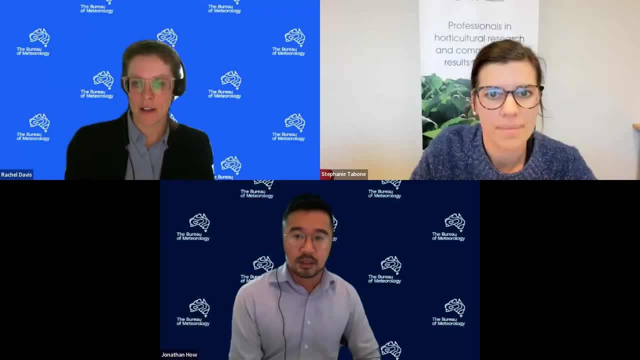 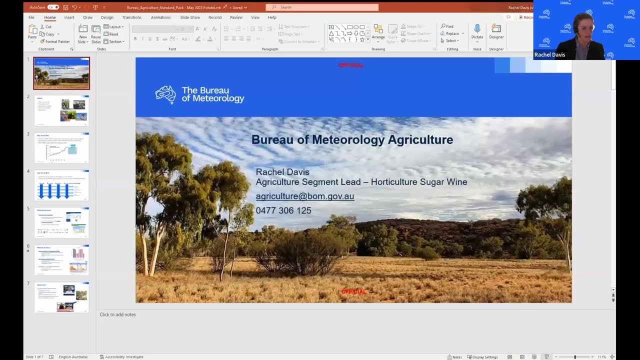 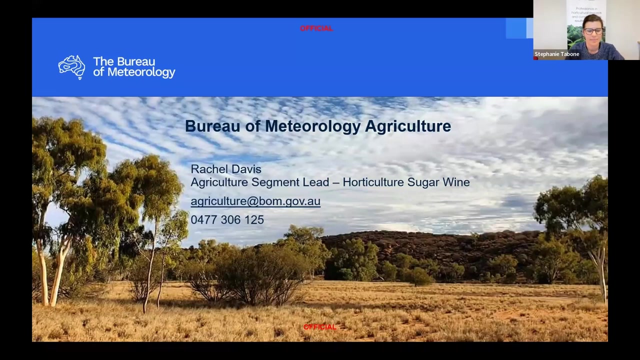 Thanks, Hi, Stephanie. Hello everyone, I'll just switch to sharing screens. Did I do that right? Does that come up right? Yes, great, Thank you. So I probably don't need to reintroduce myself. Steph already did a pretty good job of that. Just a big thank you for having us along today. I'm really looking. 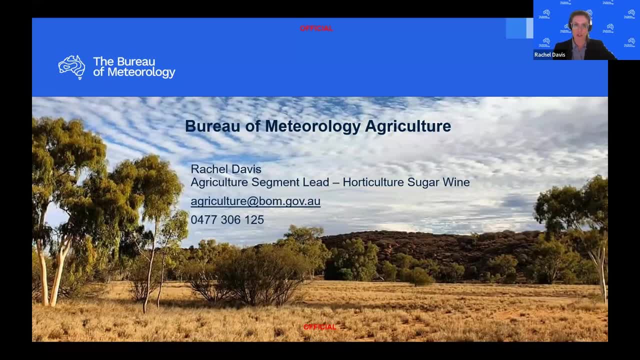 forward to the session, and in particular, obviously, Jono's session, for us to learn a little bit more. but I thought I'd start with a bit of an introduction to the Bureau of Meteorology and what we're doing here in the Agriculture and Water Program. So yeah, a little bit about. 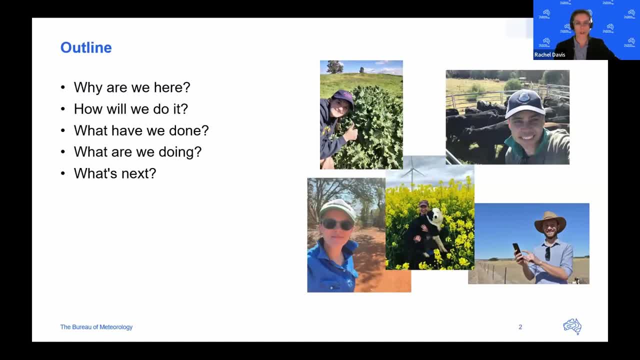 why we are here. you know what we're doing, how we'll do it. you know projects we've got going on and sort of what's next. So Jono doesn't feature here, but this is our team in agriculture. 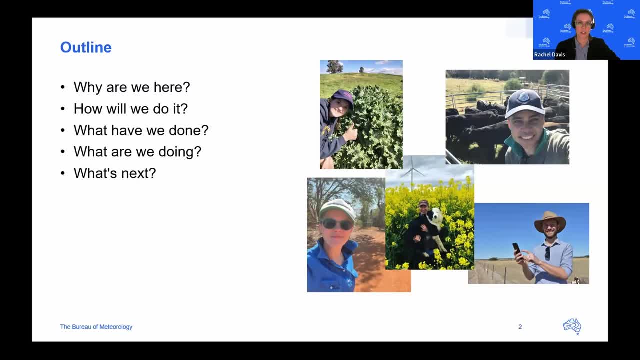 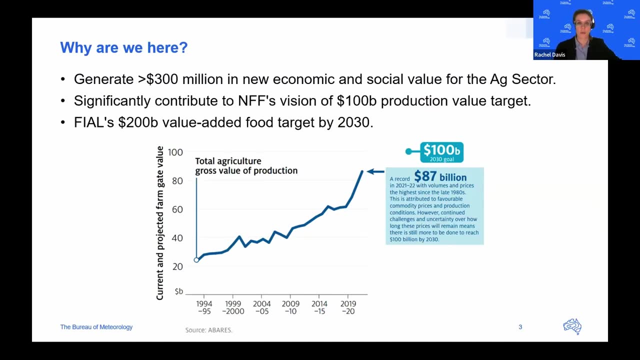 so we're the front door, I guess, to the Bureau experts And, yeah, it's our role to be the industry representatives. So the agriculture team is here to generate greater than $400 million in new economic value for the agriculture sector And this is also to significantly contribute to. 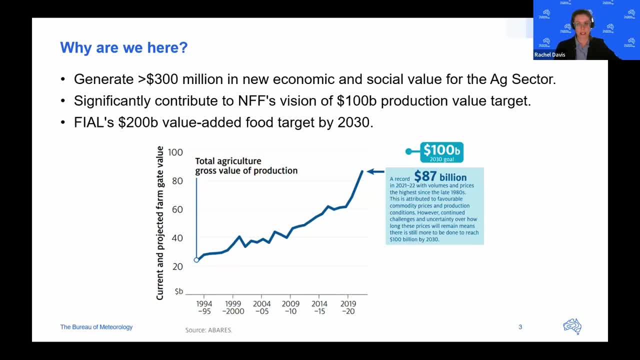 some you know industry targets and visions that have been set. So the $100 billion dollar production value target, which, all going well, we're on track for, and also there's a you know some food, food value added targets that feel set too. So how will we do it? So, as I mentioned, 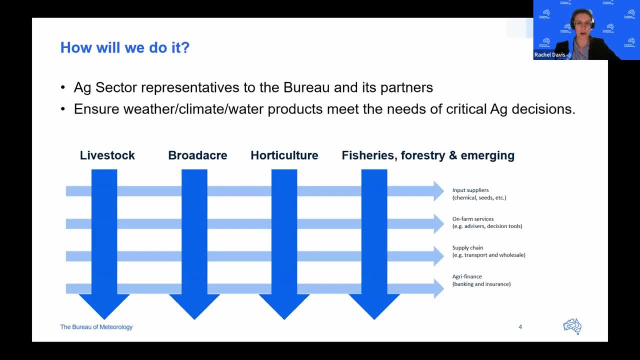 we've got a team of agriculture representatives and it's our role to ensure that the Bureau's weather, water, climate, products and services meet the needs for the agriculture industry and assist with key decisions that are being made. So we've tried to split, I guess, our team. 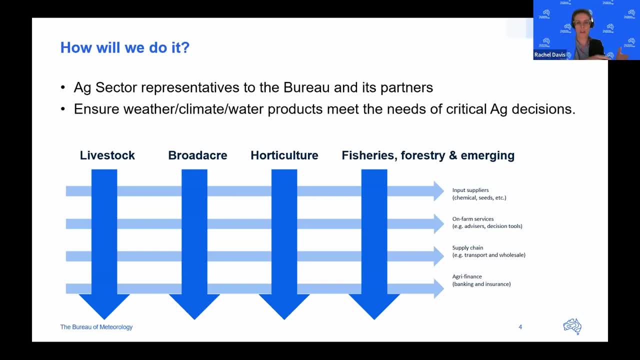 to try and cover all of agriculture, noting that it's not just production that can get value out of weather and climate tools. There's the whole supply chain that we really want to try and represent and, I guess, assist with understanding the tools. So yeah, 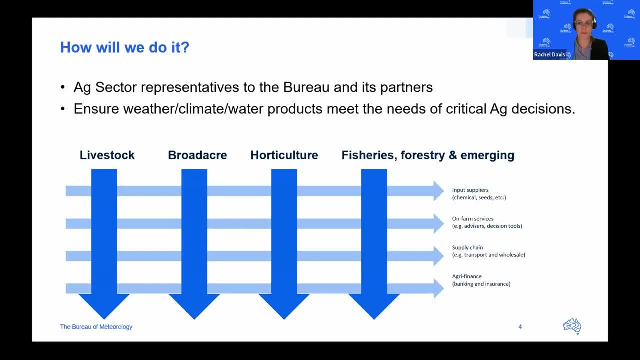 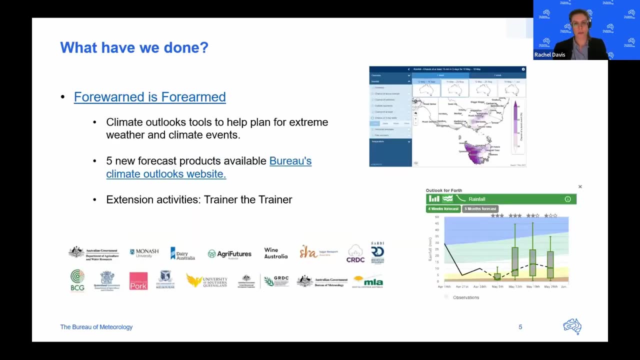 covering off livestock, broadacre, haul it, fisheries and emerging and also then, you know, secondary focuses. split between our teams trying to cover all those value add sectors are very important. So just a bit about what we've recently done. So we've done a lot, but I thought I'd just mention one project is the Forewarned is. 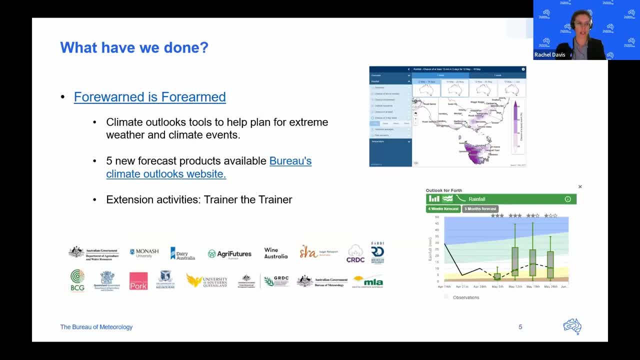 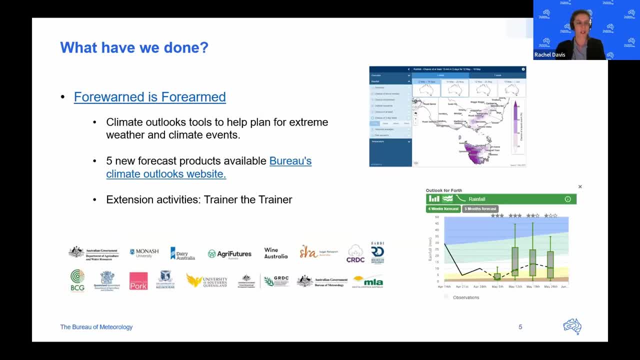 and the partners in those logos below. But so these five new forecast products essentially equipped farmers and agricultural value chains to proactively manage the impacts of extreme weather and climate events, And there's actually even a officially wrapped up last year. there's some extension activities going on at the moment that will be delivered next month with 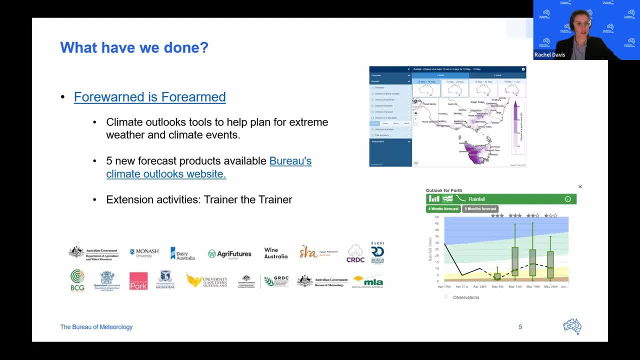 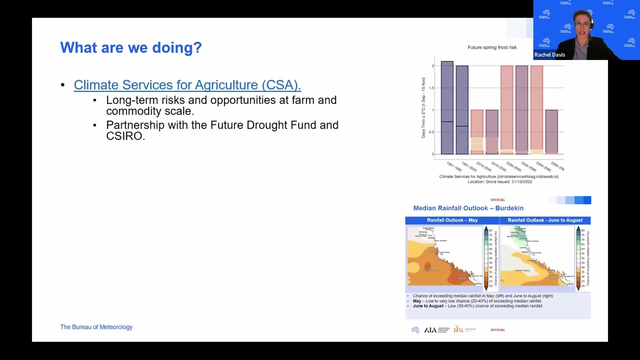 train the trainer extension activities. So Jonathan will actually be showcasing some of these new products in his interactive session. So yeah, just some tools wanted to mention out of a project that came about recently. So what are we doing now? So big project is the climate services for 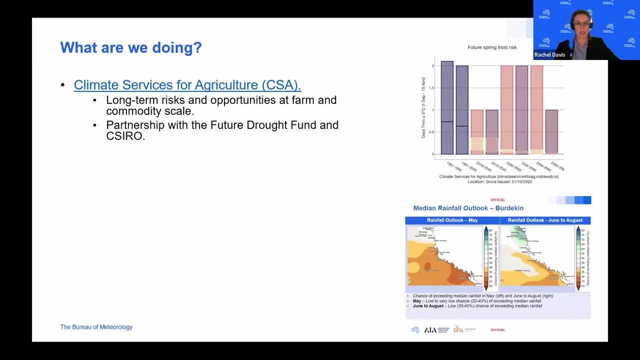 agriculture project. So we do have a separate team looking after that and I've included an image there on future spring frost risk and yeah, it looks at that platform- still in development phase but you can use it now. looks at long-term risks and opportunities at farm and commodity scale. 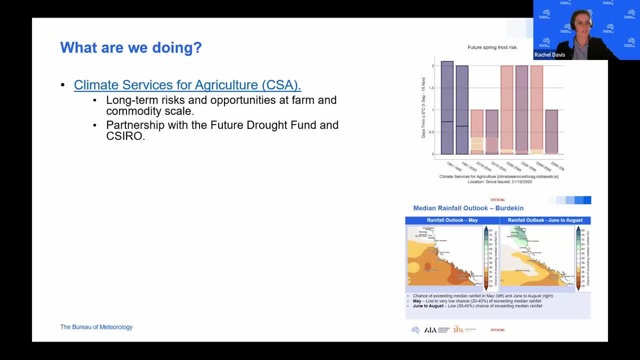 And so, as mentioned, it is in still in development phase and potatoes are actually currently in review, for you know, on a wishlist To be released on the next update to the platform. so watch that space. but you can go play on that platform and choose general, even though it may not have your specific commodity. 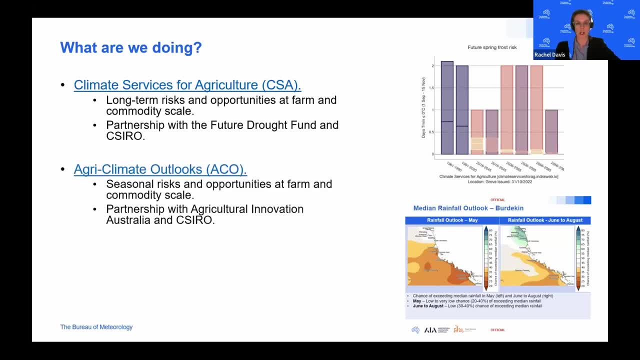 Another large project we've got going on is called agri-climate outlooks, and so that's fitting not the long term like CSA, but fitting more into the seasonal space. So what's happening in Tendad and it's not in the up to 200,000 population, So that's, you know, almost 100 days up to you know. 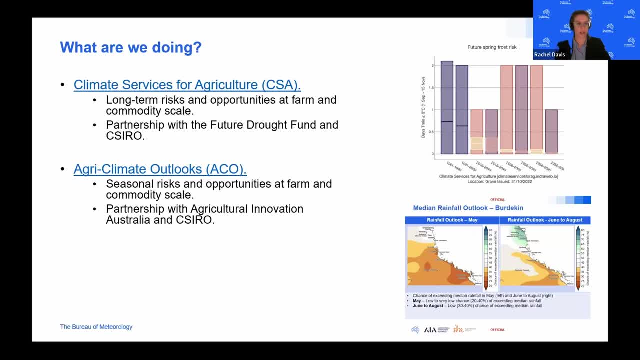 I think we're kind of trying to cover up to 210 days or something like that. So it's in partnership with AIA and funded through the RDC. So actually haunt innovation, um, maybe, um about sign on, sign on the dotted line and investment through the vegetable levy funds. So that's really exciting. 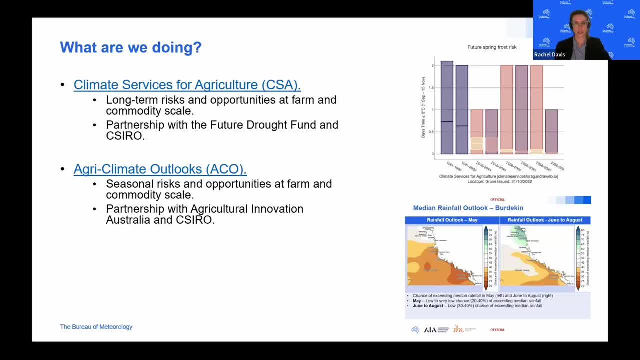 Exciting space as well. I've just included some stuff we've been doing as well publicly available. there we are some projects that have beenи a screenshot for the sugar industry that have invested in that. Another project, or product as you could call it, is OBSCHECK, and this is using trusted private automatic weather stations and 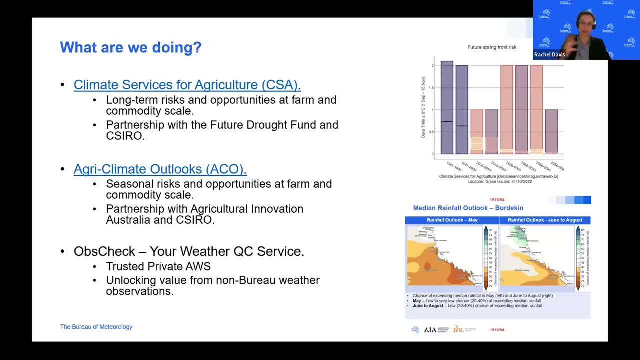 doing a bit of a quality check, noting that there are gaps in the Bureau's weather stations and trying to fill that gaps with, I think, the 20-odd thousand private automatic weather stations that do exist across Australia. So that's getting some legs this year, which is great. 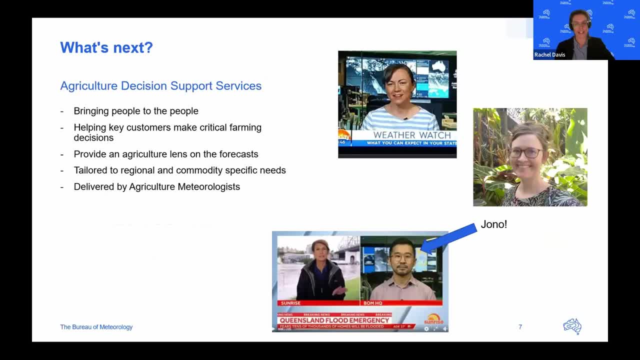 So just wrapping up, I guess what's next- and this will lead into Jono's presentation- but through the Agri-Climate Outlooks project we've been able to stand up, essentially agricultural meteorologists and bringing, yeah, I guess, people to the people and putting an ag lens. 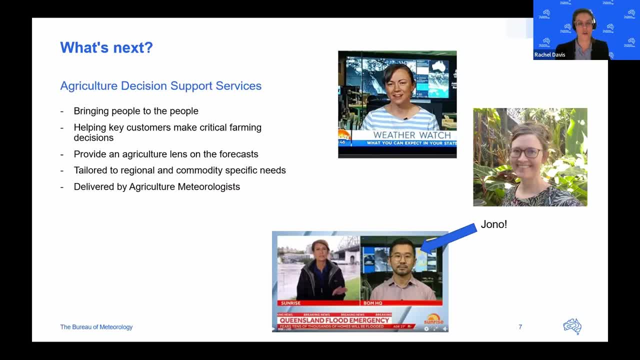 on the, you know, the publicly available forecasts that do come out and so really making them like impact specific and a bit of a so what to what's going on the weather and what that means for you in your region and with your commodity. So yeah, a little bit. that's Jono there in you know. 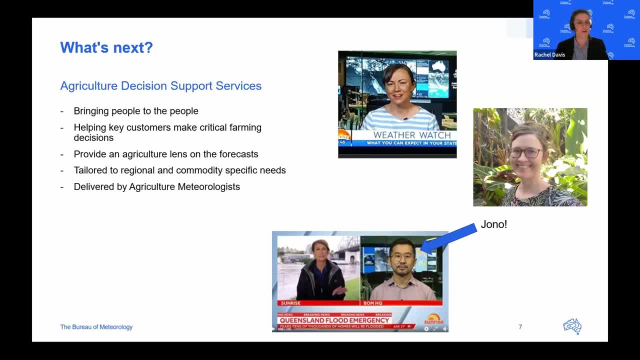 one of his media roles- public facing media roles. so, without further ado, I'll get your computers ready. I think we've got a poll coming up and I'll go back to Steph for that. so thank you for giving me the opportunity to give you a little bit of insight into the big picture of what we're doing. 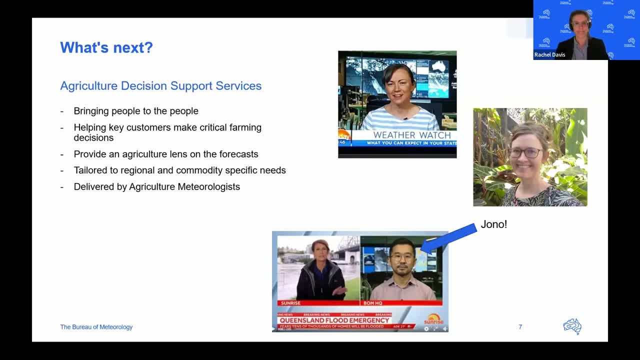 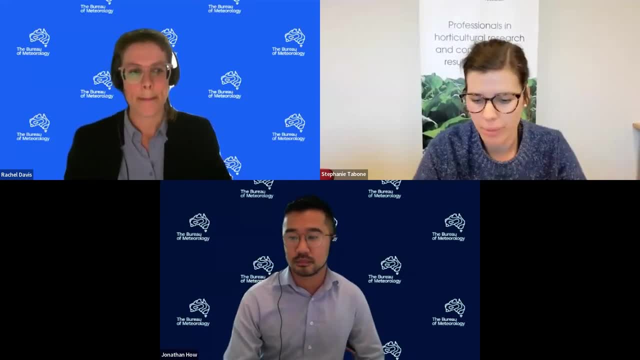 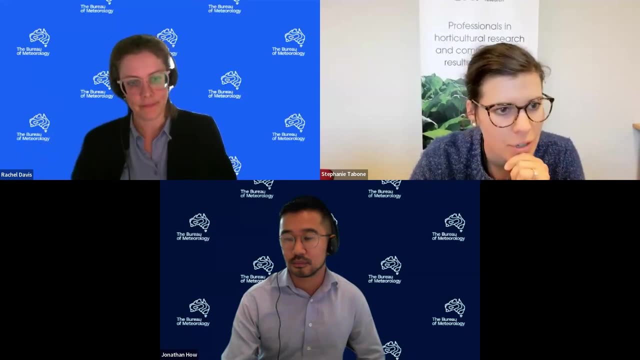 at the Bureau of Meteorology for Ag. Thanks for the introduction, Rachel, and you had some really great links there, so we'll we'll look to capture those links when we upload the recording of this session, that you can access the tools that Rachel outlined Before we jump over to Jonathan, I might 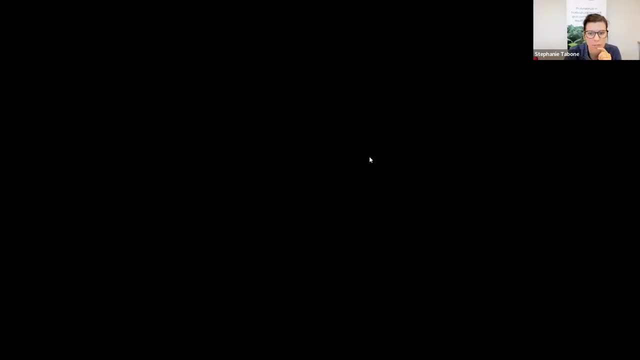 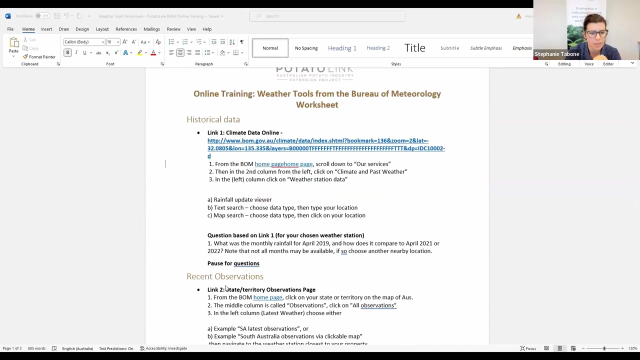 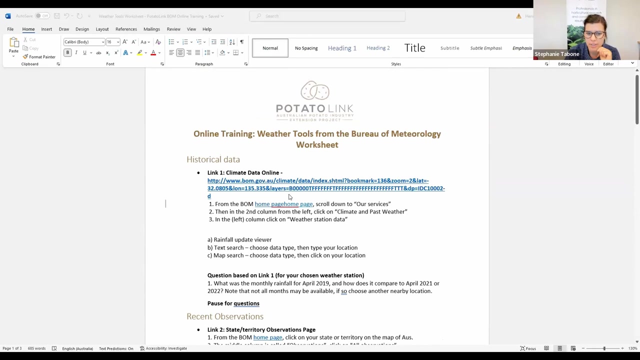 just share with you the worksheet which you should have access to and just roughly how this is going to run today. So we've broken this into four segments- historical data, recent observations, now casting and forecasting- and you'll see that there are a series of links. 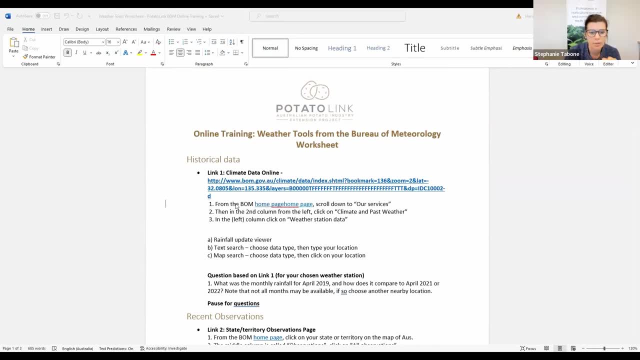 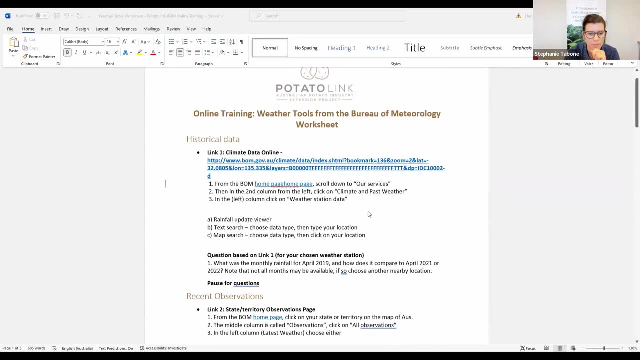 The top link takes you directly to the tool, but if you want to follow through the steps that Jonathan will work through, we've provided some links for you to click and follow along as we go. So I think that should be most of it. We'll have a couple of polls where you can pull out your. 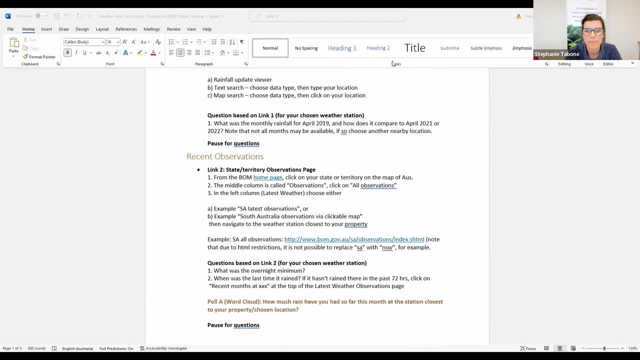 smartphone or access it directly from your computer, and I'll also share some polls now to get this started. Bear with me just checking that you guys can see that One second. okay, there we go. it should work fantastic. Okay, so using either the QR code: 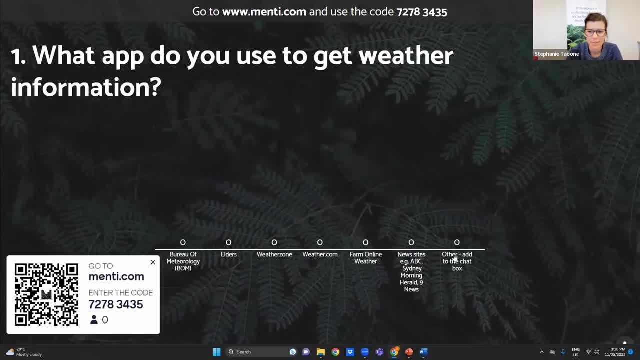 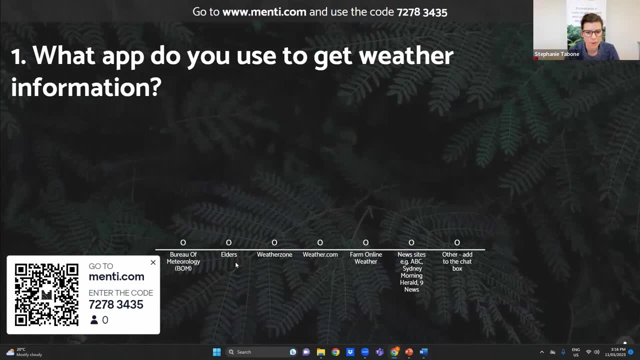 at the bottom, or menticom, and entering the code for participants. today. it would be great to know what app you are currently getting your weather information from, Whether it's the BOM, Elders Weather Zone, weathercom or any other potential weather tools and you're. you're welcome to pop. 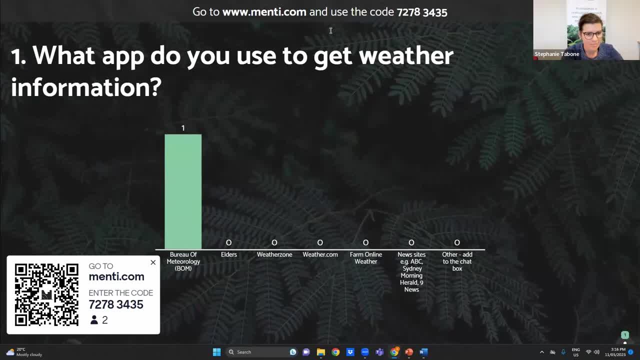 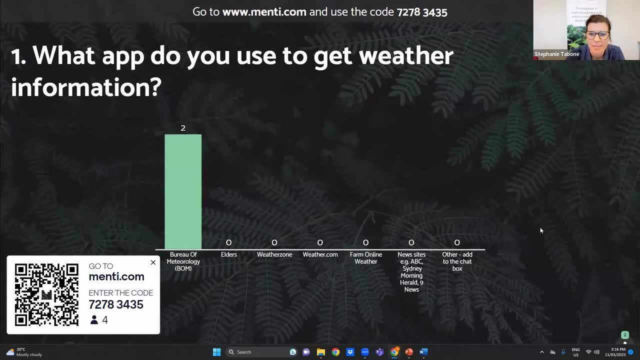 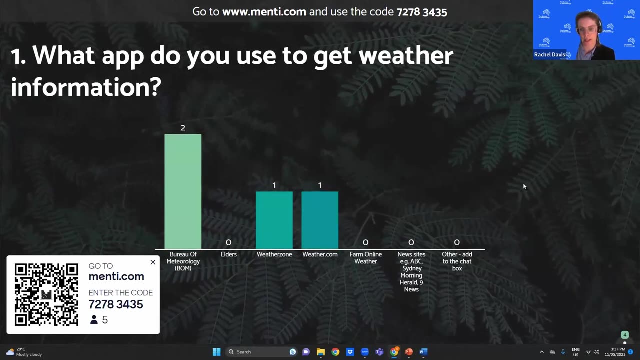 anything else that I've missed off here in the chat, And we've got one respondent with the Bureau. we've got a few people joining now as well, So is this Steph as well The one you most use, bearing in mind that you can only click one answer? 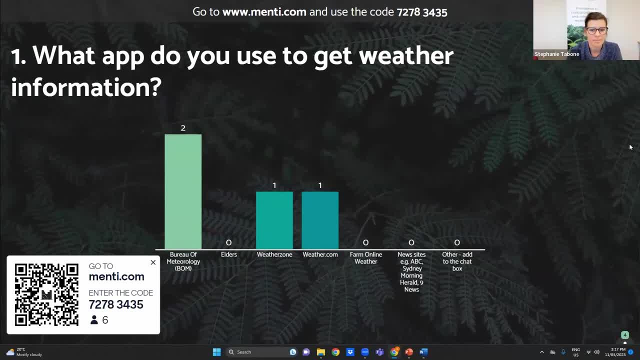 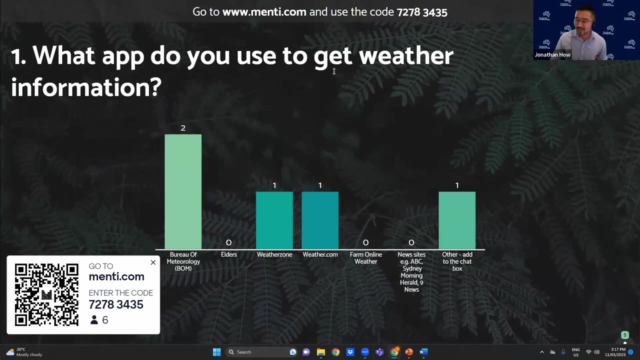 Great, yes, Okay, might be interesting, Jono, as a few more comments are coming through here. What is like the difference between the Bureau tools and other tools that are available? Thanks, Steph. Good afternoon everyone. So yeah, there's so many different apps out. 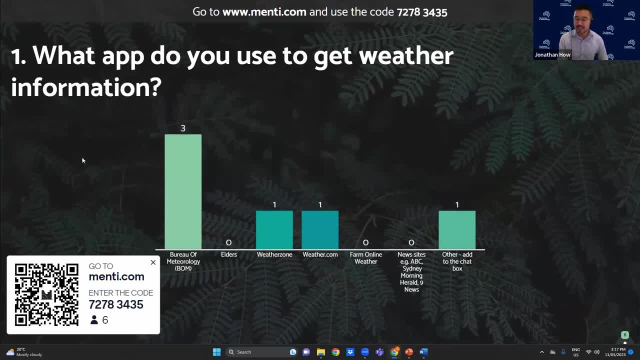 there to get your weather from. Obviously, the Bureau one is the one that we develop and we use quite a bit of model data to do that. but the difference between the other ones does come down to first. you know different features. there might be different colors, or some people might find the layout a little bit more user-friendly- For me, for example. 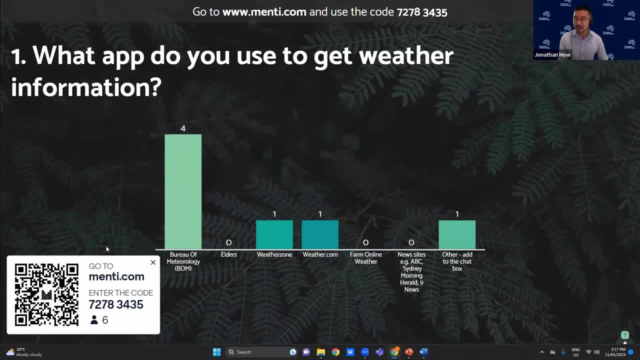 I love using Wimdycom. I think that's a really great and easy one to use, but they basically what they do is they take the model data- whether that's the Australian model data or European data- and then repackage that so the Australian access data is really easy to use. So the Australian access data. 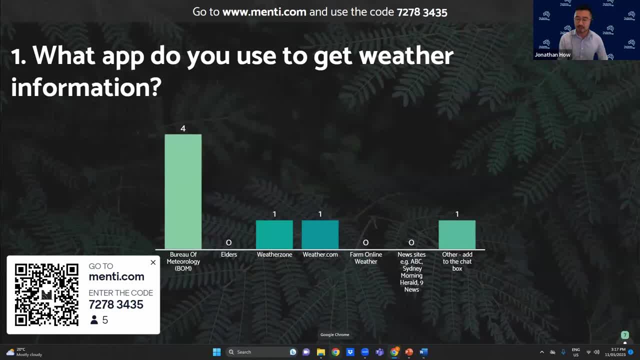 is freely available, and then all these different app companies come in and package it to what? to what they need, what they want to show. Thanks for that, Jono. So it looks like most of the people online today are looking at the Bureau app. All right, see if we can progress. 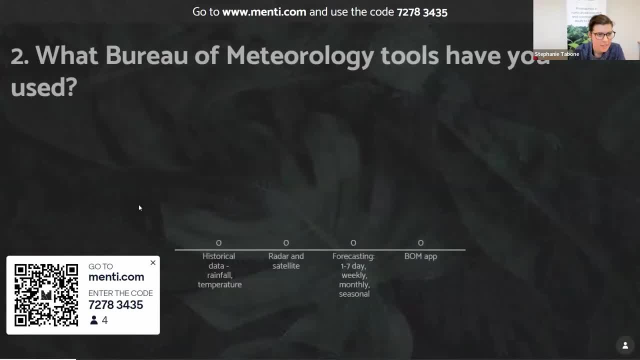 to the next question. All right, so second question is: what Bureau of Meteorology tools have you used before? I imagine there's probably a big range of different tools. We already have a number of different tools that we use and we know everyone's using the app. based on the last question, 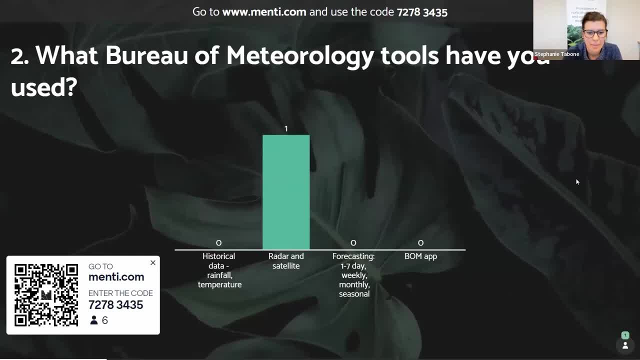 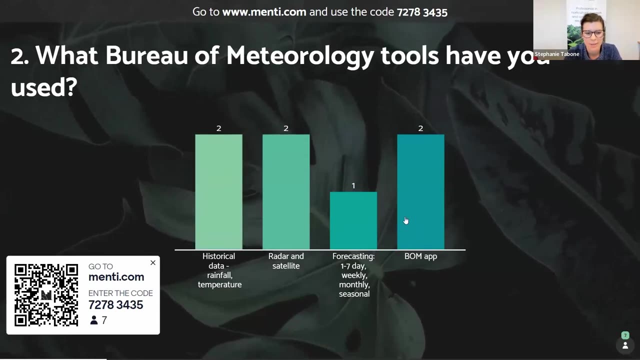 but let us know what have you accessed? Fantastic Should give you the option to select model one, I believe, if you are using all of them. Yeah, it's um a range of different tools being used across, So a lot of these we're actually going to delve. 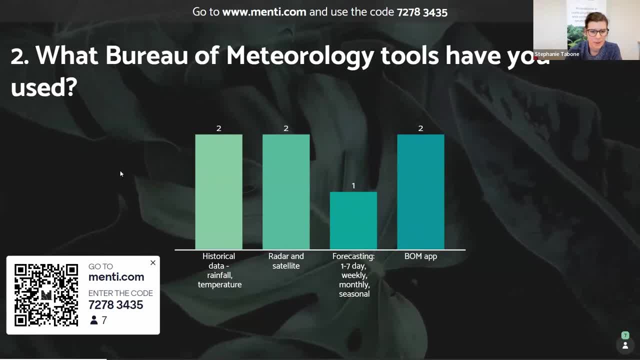 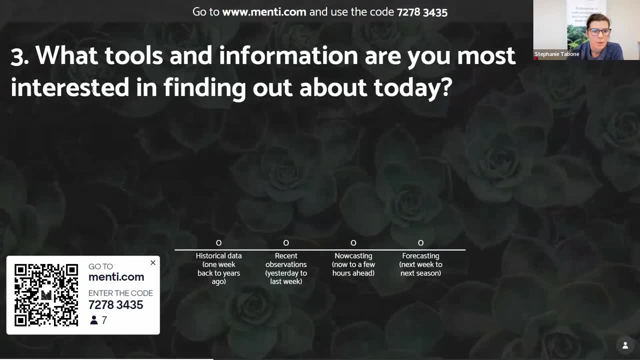 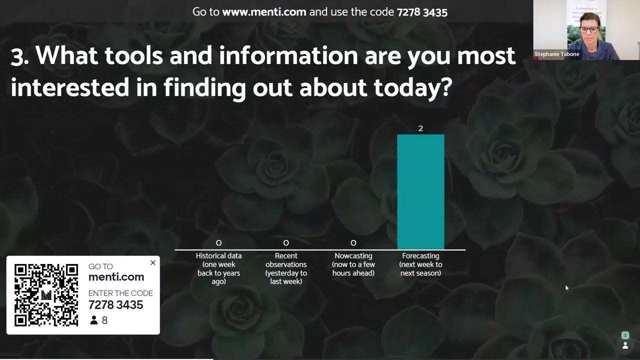 into more detail today. So, okay, move to the last question. What tools and information are you most interested in finding out about today, during today's session? That way, we can focus our attention predominantly on what you're interested in. We love to hear from you about it. 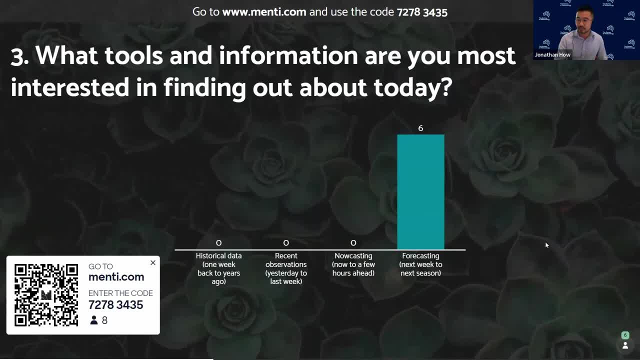 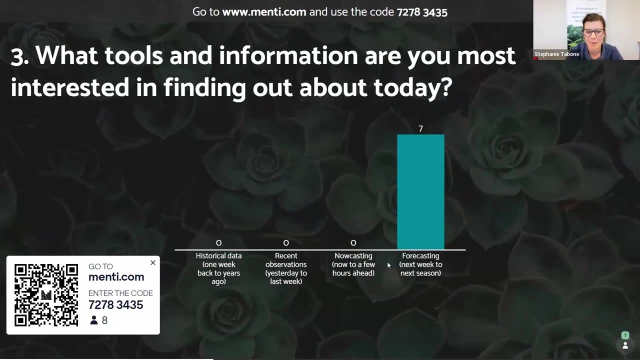 So I'm going to hand it over to you, Jono. Yeah, that's, that's good to know. So I'm definitely focusing on forecasting. Well, it looks like a consensus. Yes, I think this, this one might have only given the option to select one, So there's probably 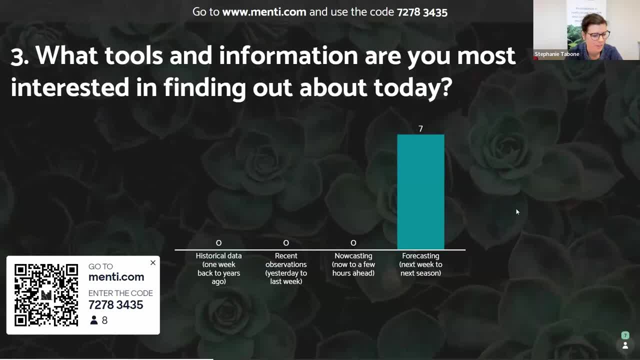 more interest in the others, But um, seems like forecast, I don't know. Okay, fantastic, I'm going to stop there and hand over to you, Jono, so we can get started in the interactive session. If anyone has any questions or issues tech-wise, 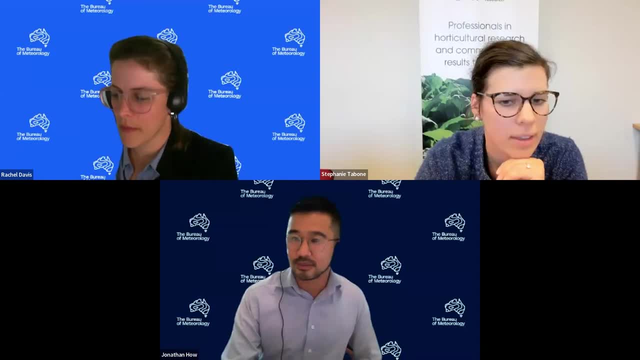 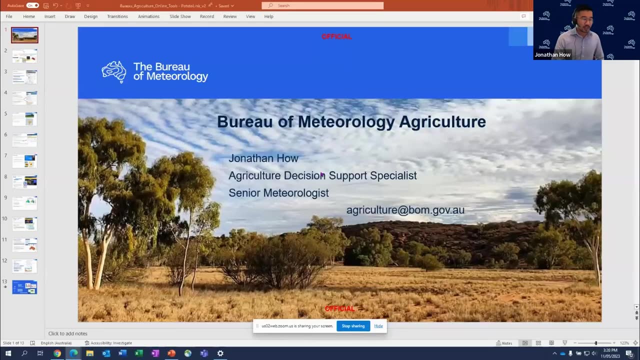 please let us know. Thanks, Steph. So good afternoon everyone. I'll just share my screen, make sure everyone can see that. So yeah, today I'm taking you through quite a few different tools available predominantly on the Bureau of Meteorology's website. 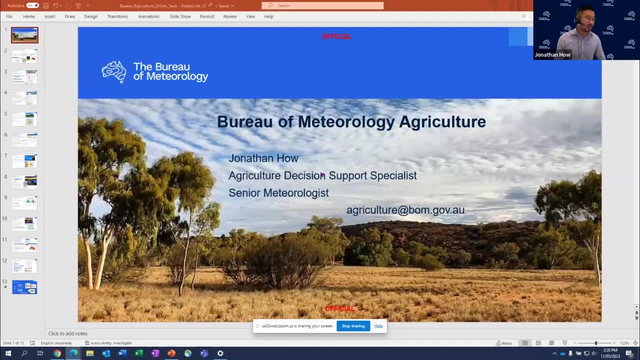 Definitely acknowledging that there's so many tools out there, including different apps, but these are just some of the ones that us, as forecasters, particularly tend to use quite a bit and just kind of give you an idea of what is available out there and how you can apply it to yourself. 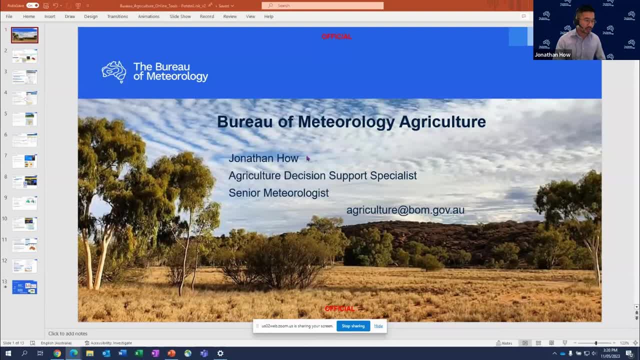 So I'll be sharing these slides on the screen. Follow along in this purple cursor as best you can, and I'll be stepping through each of the examples. So feel free just to follow along and watch the screen or, if you'd like, you can definitely follow along at home. 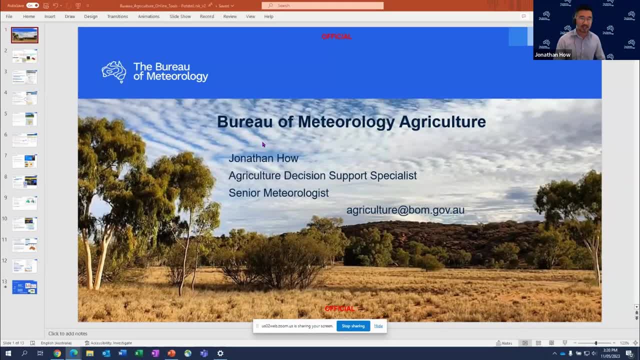 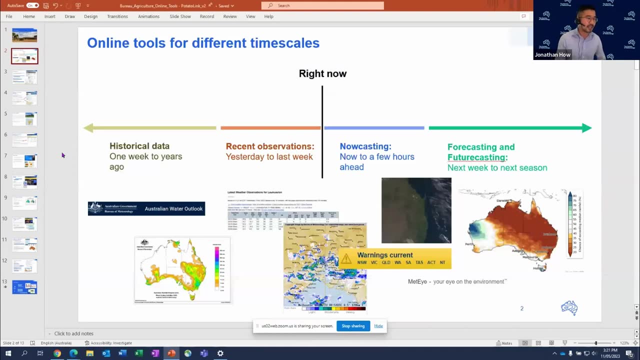 for a particular weather station, that one places to you or anyone across the country. So I've just got the worksheet next to me at the same time and I'll be flipping back and forth between this PowerPoint slide and also the Google browser. So, in terms of online tools, 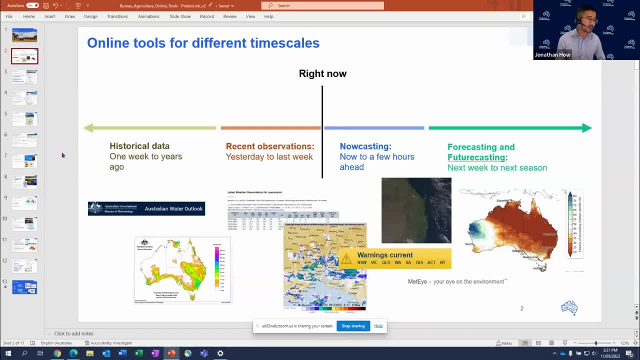 the easiest way to think about it, as Steph's really alluded to, is on different timescales, So stepping all the way back on the left-hand side to historical data. the Bureau has data all the way back to 1900, all the way up until next year or even a couple of years. 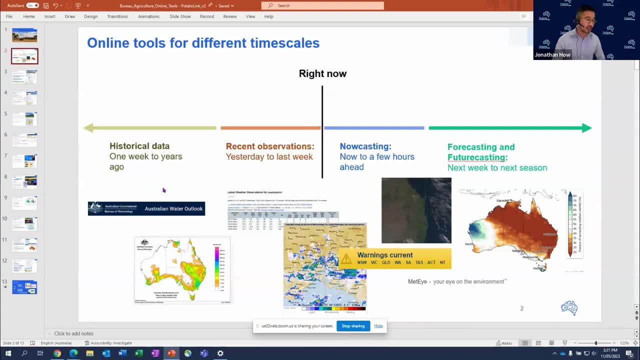 ahead of some of these really advanced computer models and then everything in between. So at the bottom these are some logos and maps and some tools you may have used, you might recognize, taking all the way back from historical data, all the way to forecasting. 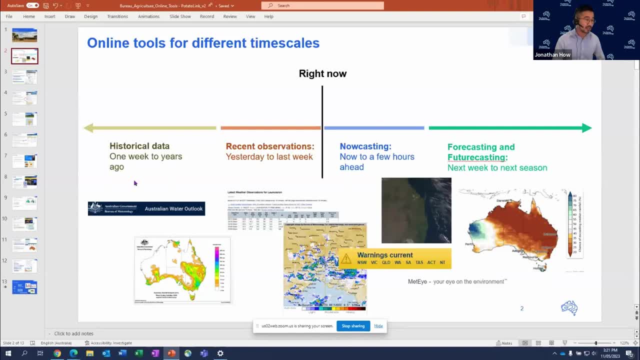 and future casting. So I'll be stepping through each of these four segments: The first slide for each one- we'll just be giving an overview of what it is, some of the main links that you can use- And then the second slide of each section. 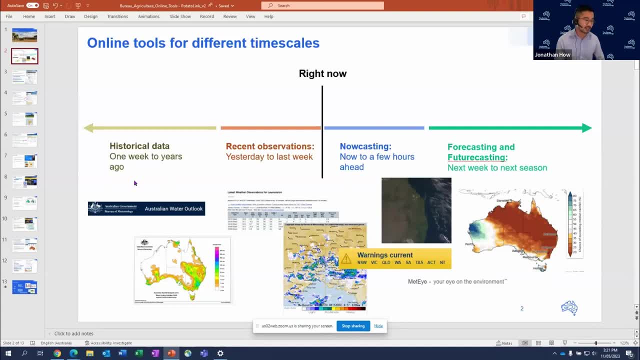 will be just doing a bit of a step-by-step interactive sort of activity that you can follow along on the worksheet or just feel free to watch on my screen. There are quite a few things to get through so we might not get through it all. 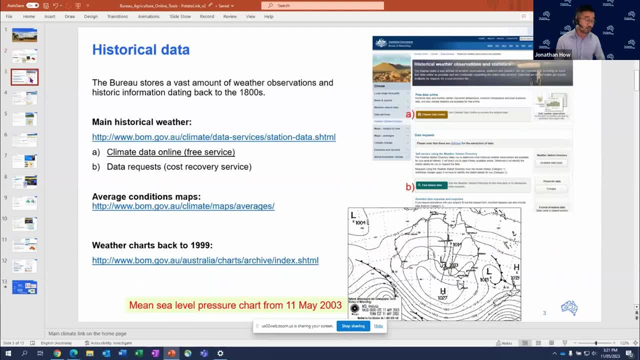 but certainly, if you don't get through it, feel free to go back on the worksheet or have a go in your own time. So the first section is historical data. So the Bureau stores data all the way back into India- sorry, in pre-1900s, 1800s. 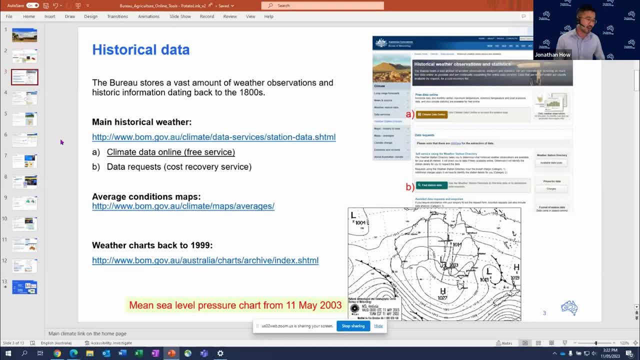 And I've got a trivia for you. The first modern weather observations recorded in Australia was with a lieutenant who came across in the first flight back in 1788, recorded for three years in Sydney before returning back to Australia. So that's a little bit of a long story. 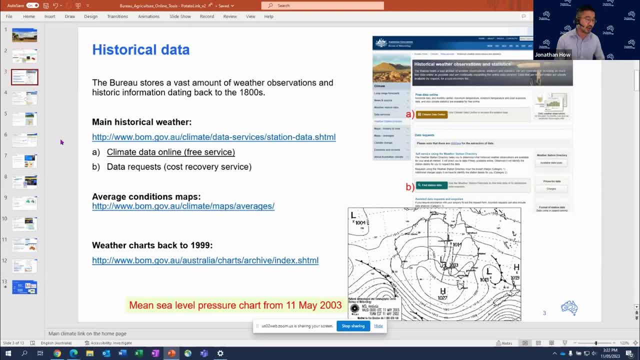 But the longest running, continuous, continuous running observation site that hasn't really changed location too much is Observatory Hill in Sydney, CBD, And the longest running city that has been recorded for is actually Adelaide, So all those go back to the 1800s. 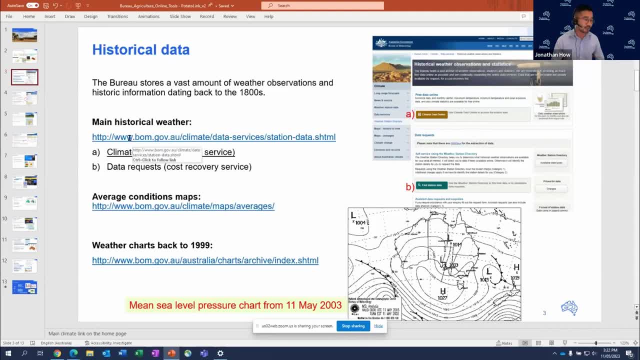 So the main historical link is this one here, this historical weather, climate data services, And the image is on the right-hand side. This is kind of the main portal for your historical data. Number A is climate data online. That's a free service. 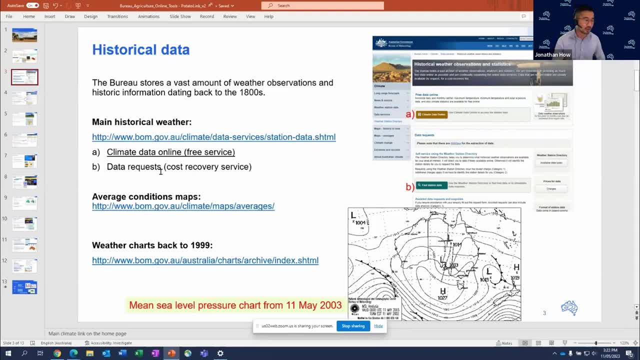 And I'll show you how to get what we can do with all that. And also B is data requests. These are your more kind of out of the box requests, that which basically are a bit of a cost recovery service. So I'll just show you how to get to that. 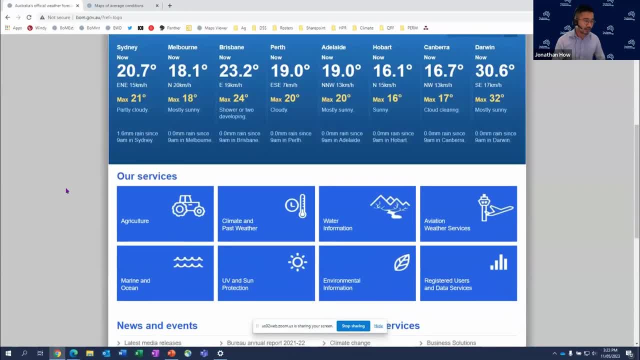 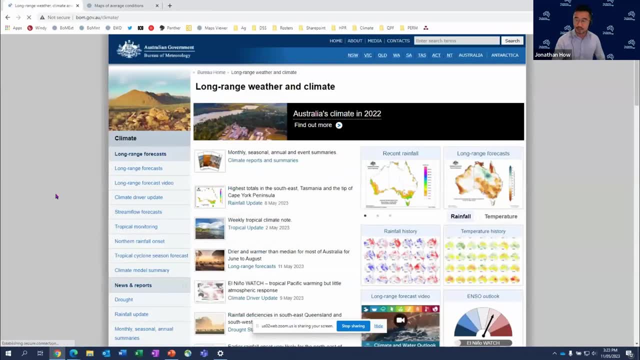 kind of climate data page. So from the homepage you scroll down to our services and you're looking for this climate and past weather link. Just click on that And here we go. Oops, That's not, Sorry, That's not doing its thing. 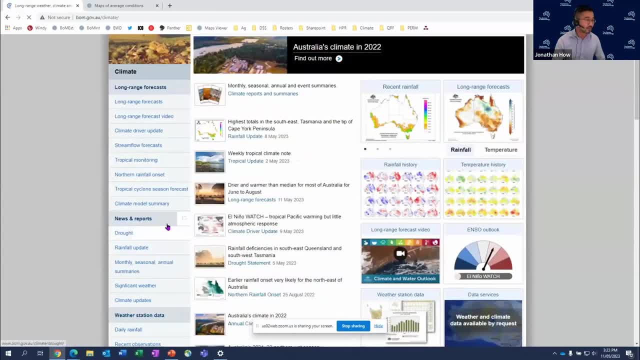 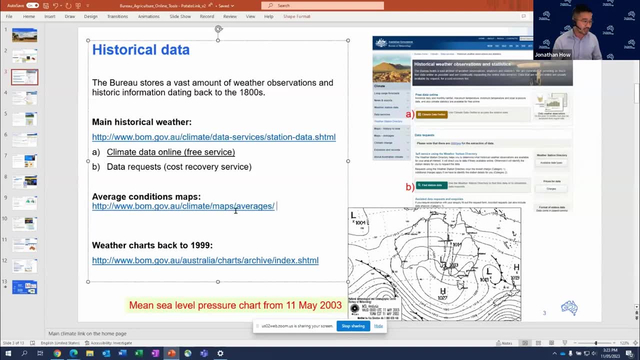 Oh, I'm sorry. I'll come back to that in a moment. Another great one we've got is these average condition maps. So if you're just looking to find out what is the average rainfall particular month, This is the one here. 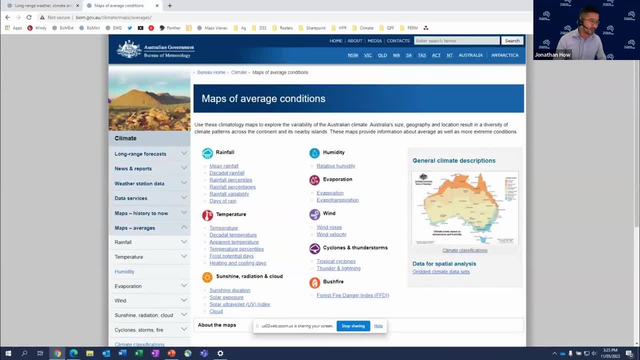 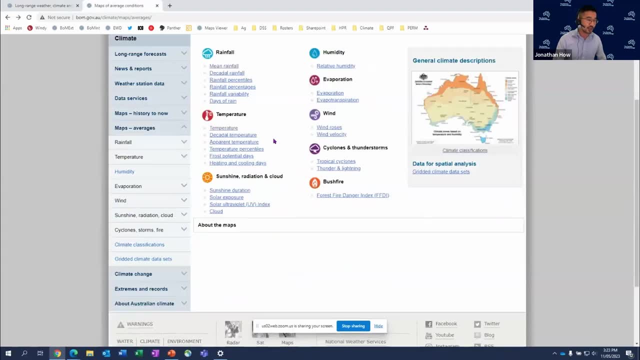 This one is the page that you're texting to before. There we go: Climate and past weather. Yeah, So give us have a look here at the next page. So this is the context. This is the kind of the mean rainfall. This is just the Australian rainfall. You can break it up by month. 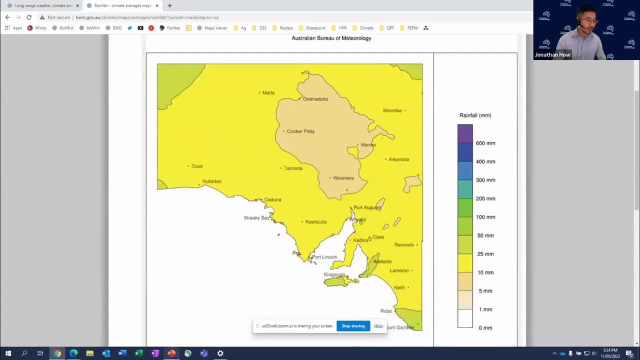 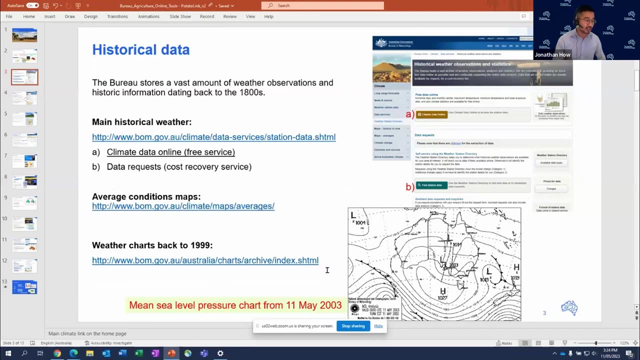 also break it up by the state as well. That's a really great resource- Another great one that people don't know too much about. if you do have a bit of an interest in looking at old weather charts, you can actually go back and look at all the different weather charts back to 1999.. So I've 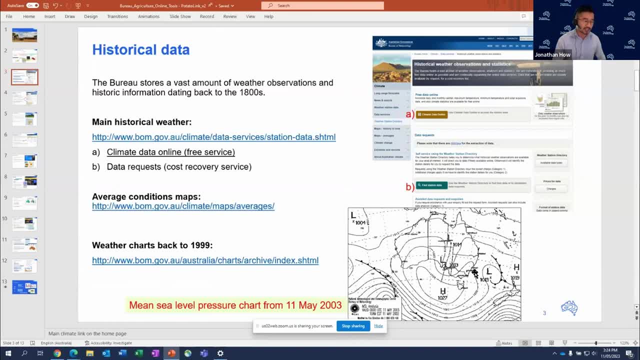 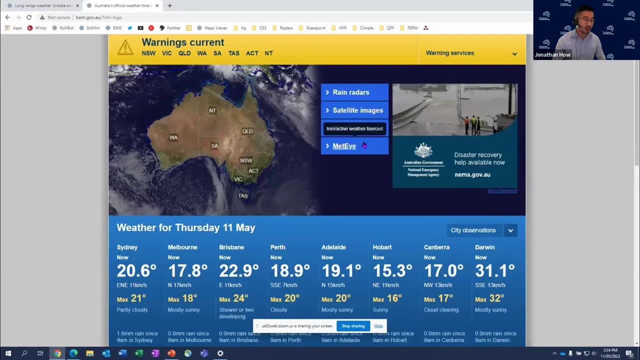 put the one here from 20 years ago today: high pressure system in the Southern Ocean and a bit of trough. So the way to get to that: if we go through the home page, click on weather maps and we want to go into the analysis chart archive here or just follow that link on the 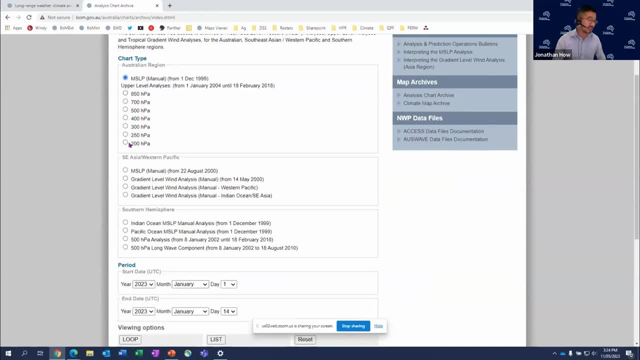 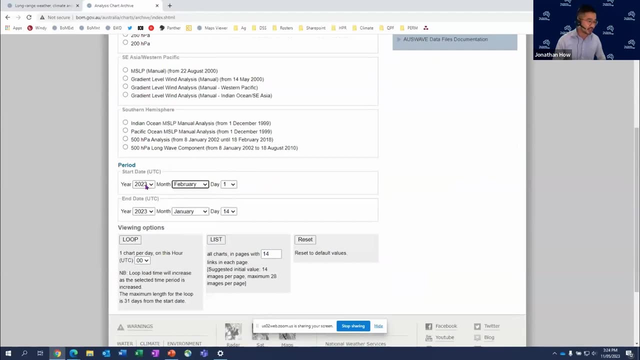 worksheet And you choose a number of different charts here. The most common one is the MSLP one, the one you see on TV and on any kind of publication, And you can just kind of choose that here. So I'll go back into February 2011.. I'm not sure people might remember what happened. 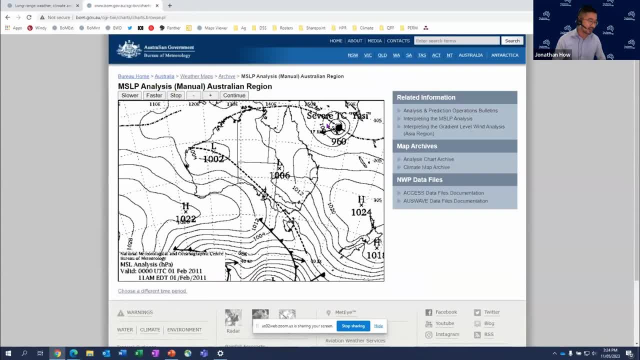 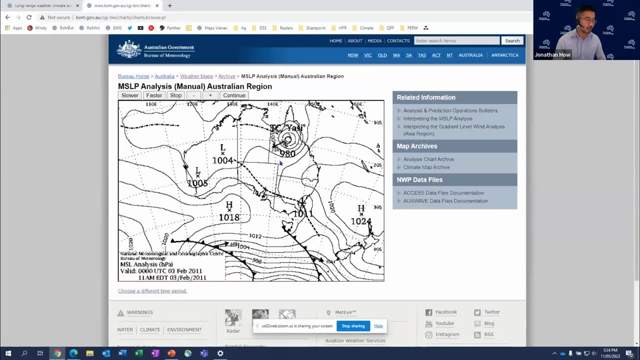 beginning of February 2011.. It was tropical cyclone Yasi, So you see here just a bit of a loop, So a really great tool. You can go back to any date since 1999 and see what was happening at that point in time. 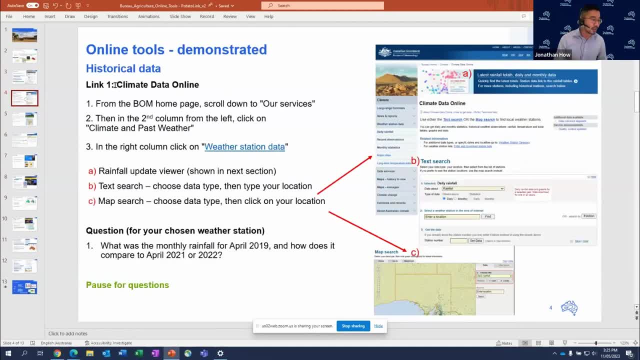 By looking on the next slide, so I will just demonstrate this tool. So what I want to show here is link one: climate data online. So on the top number A, we've got this rainfall update viewer. It's a fairly new tool And I'll 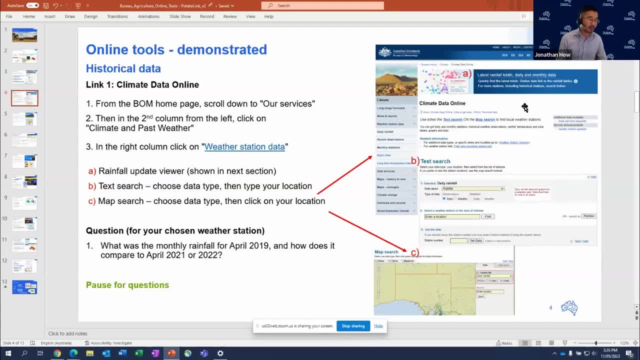 show that in the next section. It's a really great way of showing the rainfall, not just for the weather stations but also all the different private rain gauges across the country. Otherwise, for any sort of weather station, you can either do a text search B or do a map search. 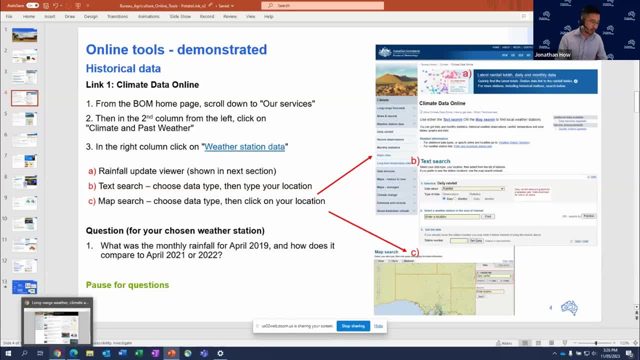 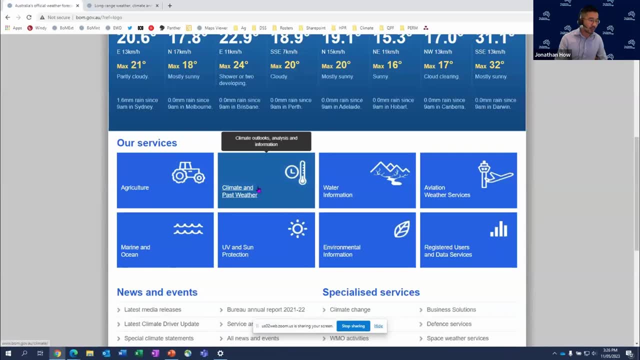 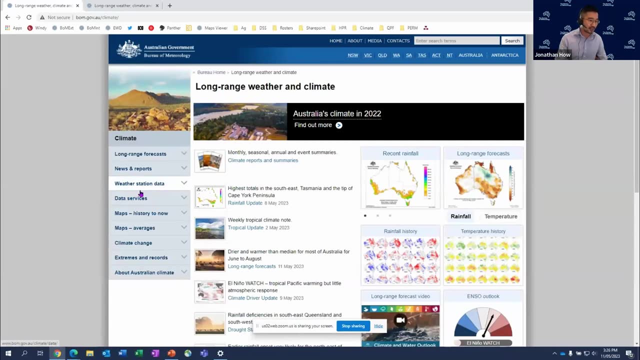 in C, So I will just show you how to do that before going to that question. So back to the homepage. what I do is I'll scroll down again to climate and past weather And on the left-hand side- apologies for the link before this- is where we do want to go to weather station data on the. 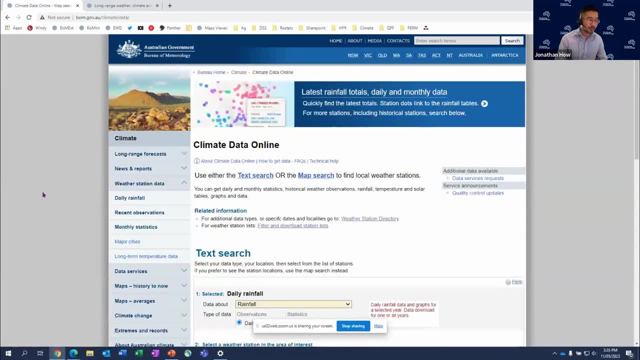 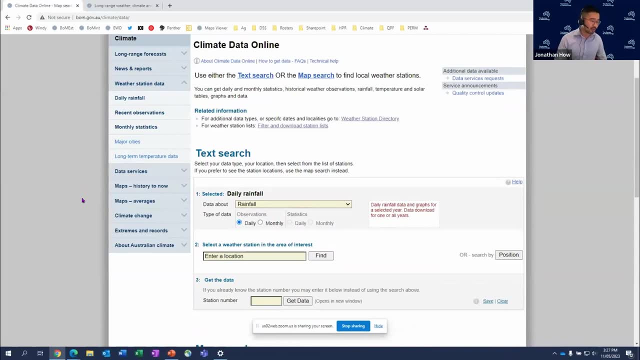 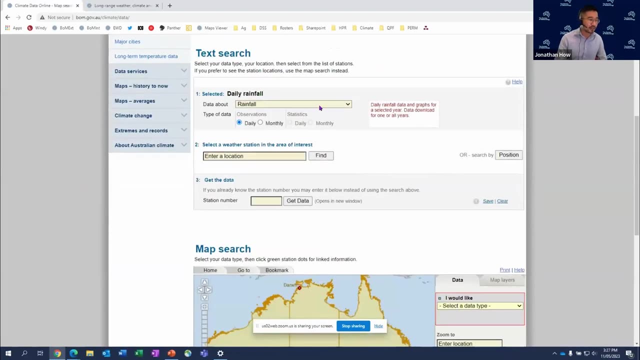 left-hand side takes you to that screen that you did see before. So, for this example, I'll just pretend that I'm in Launceston, for example, and I just want to see you know what was the rainfall over the last couple of months in Launceston and really any any station in the country that has the data. So, firstly, you, 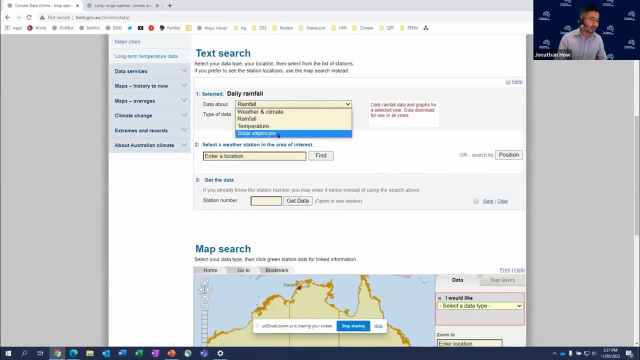 can choose between weather and climate, rainfall, temperature and solar exposure, but for this activity I'll just keep it on rainfall. So, yeah, feel free to enter your own location, but I'm just going to go with Launceston here, and it comes up with quite a few different matching towns and 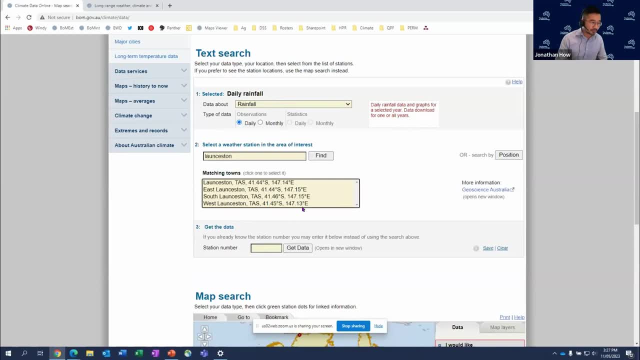 different observation stations. So as you can see, here there's- yeah picked- quite a few TAS and Launceston, east, south and west- I think the first one- and again it'll take you to the different nearest bureau stations. So a couple of stations in town, but I might want to be most interested in 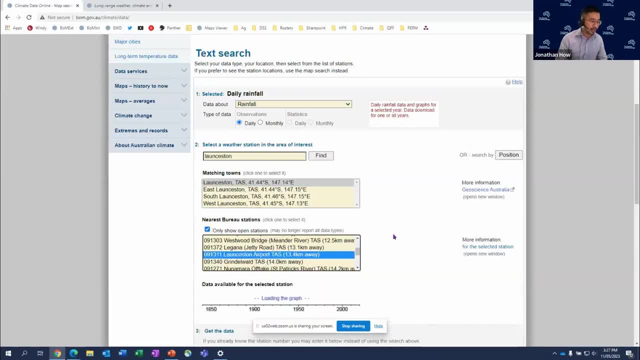 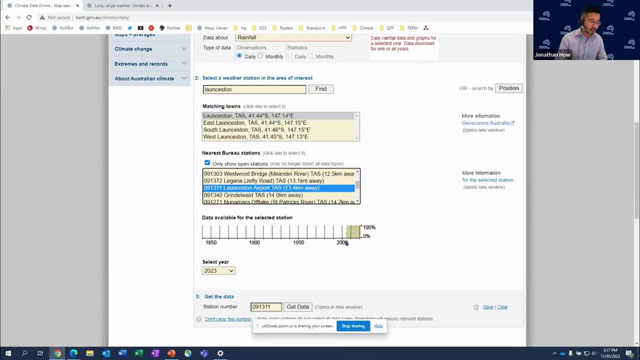 to scroll down Launceston airport. So, clicking on that, the next thing you'll see is how long the data has been available for. So, looking at Launceston, yeah, it's been available since probably 2004, but some of these other sites might have much more data available. So, 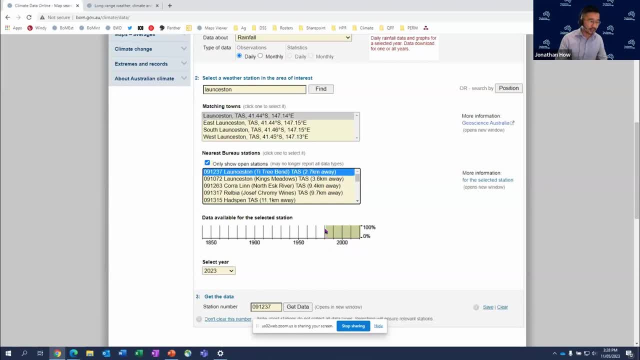 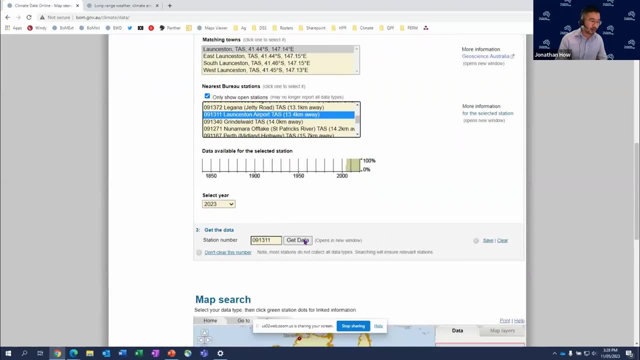 Tea Tree Bend looks like it goes back into back to 1980.. What I'll do is, yeah, really, for the purpose of this, I'll just choose Launceston airport and then click on get data and what you'll see is the daily rainfall figures going back as long as the date of the event. So I'll 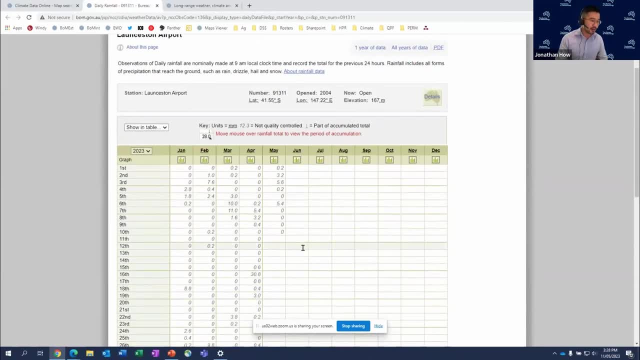 go ahead and hit it as early as the date of the event and change the date for that. So 1 month later you will see the rainfall is gone for about two months, almost twice as long as the data is held. So it starts off in 2023.. You can see here rainfall so far this month in May. 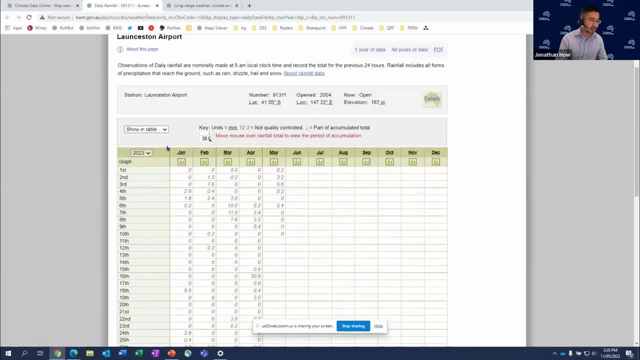 and then the last four months so far this year, and what you can do is filter on this top left-hand side here, or you can also go back in time as well through here. So if we just look at the question, question one: What was the monthly rainfall for April 2019 and how does it compare to April 2021, or? 22, depending on what. so they list over here that kind of palm tree acredальномia is, You'd see, ポン curious definition for April which, if they look at this political graph as well, they'd put more. therefore rather chopping, and so we can go back and look and look, basically the results. so yeah, that's. 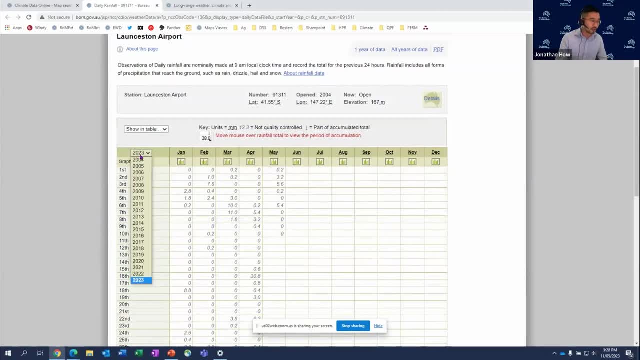 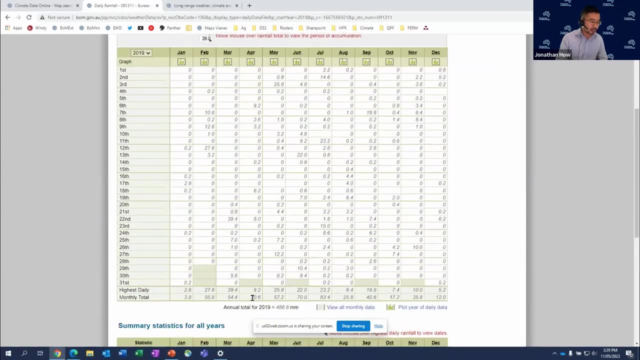 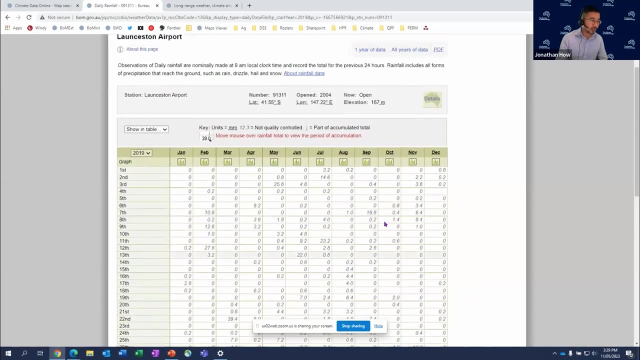 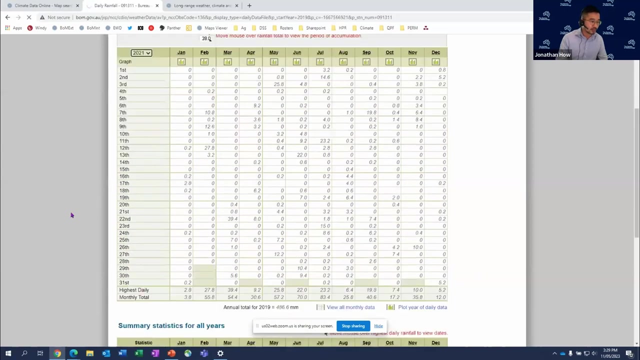 what data is available. So if I just want to go to April 2019 here, I can see that for Launceston the monthly total was 30.6 millimetres- just at the bottom there, and comparing that to April 2021, so that was 30.6 and looks like April of 2021 was 19.6 millimetres. So 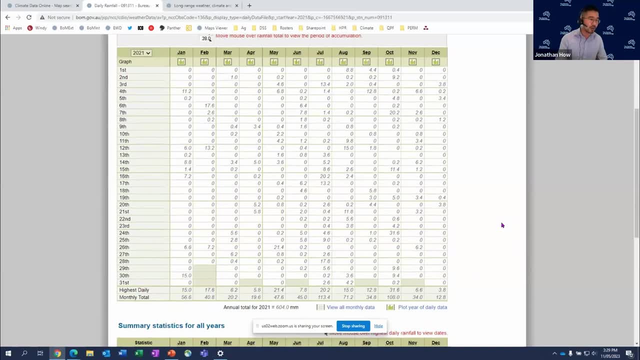 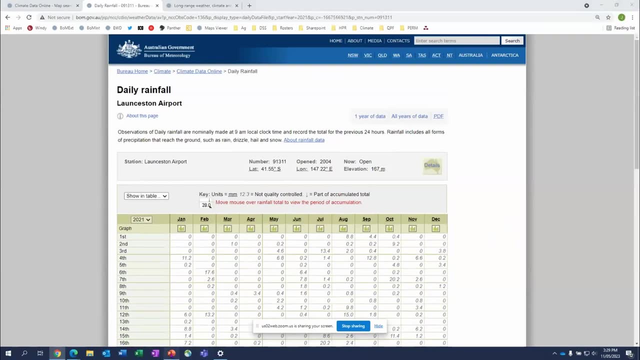 just a bit of a tool. if you're curious, definitely spend some time going through. if you're interested going through this kind of climate data tool, a lot of information available on there. Yeah, and otherwise there's also a map search. so basically the same kind. 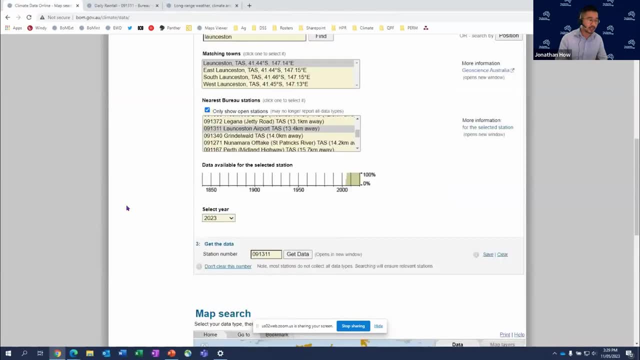 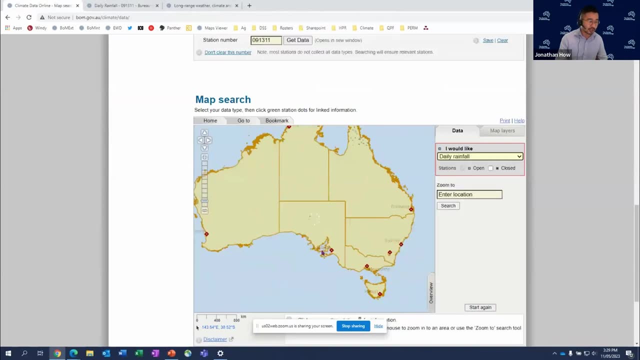 of functionality. If I go back to this climate data page and scroll down even further, there's a map of Australia and if you just kind of select Daly Rainfall, it shows you all the different locations right across the country and there is a zoom capability. 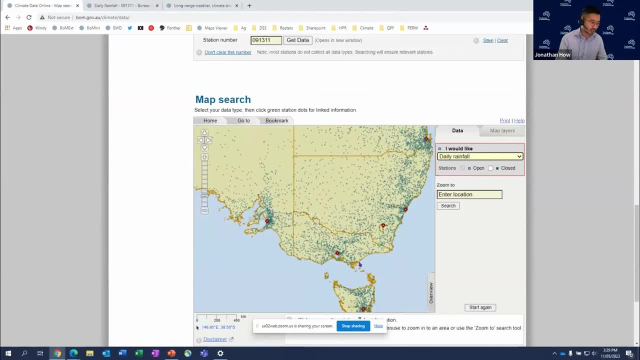 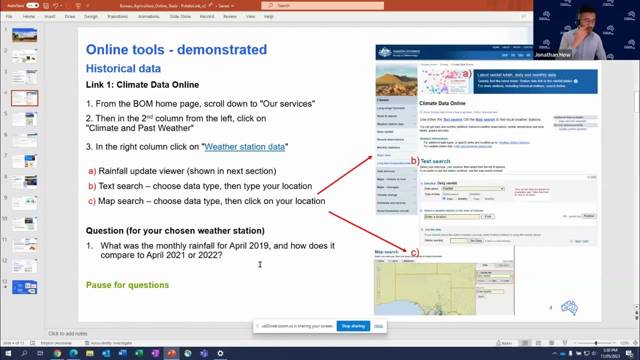 So you can definitely spend quite a bit of time going through all the different rain gauges and all the historical data that is stored. So I'll just pause for any questions- Yeah, any questions. people might have pause for a little bit Just while we give the opportunity for people to pop questions in the chat or to come off mute. 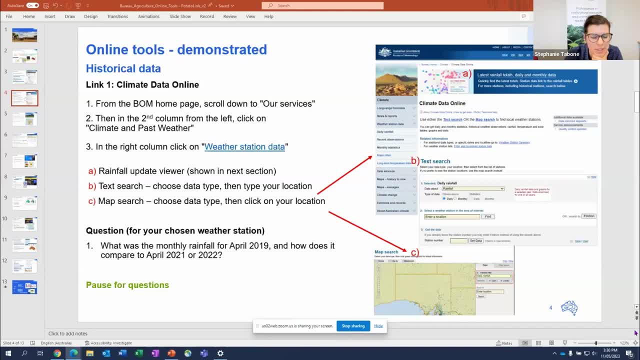 I just thought I'd ask Peter or Brian if you wanted to share a couple of comments on how growers might use this information with respect to planting or harvesting. Well, for me, I think the historical data is really important If you're in a new area. 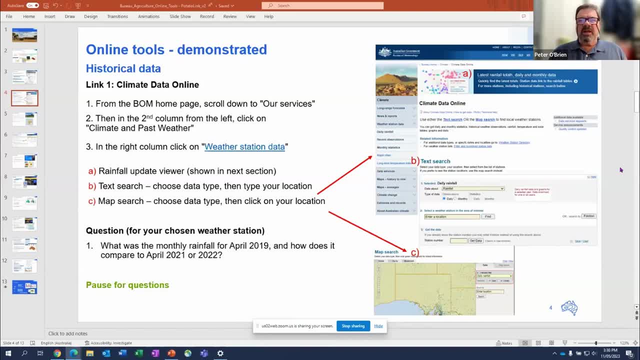 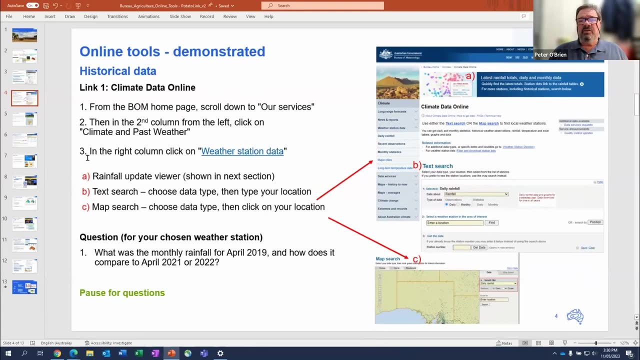 understanding. you know the key times within your planned growing time. it's kind of important to understand those things and you know, in my previous life I did startups for PepsiCo and I used to go to this kind of data to work out where I should grow potatoes in a country and 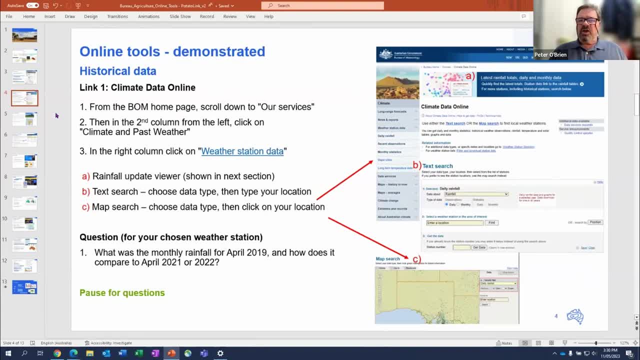 it's no different if you were to go to a new location. find out as much as you can about the climate within the window you're planting, and it will be highly enlightening as to what the risks and opportunities you might have for a specific region. Thanks for that, Peter. There is a comment in the chat here, so it's from Peter. 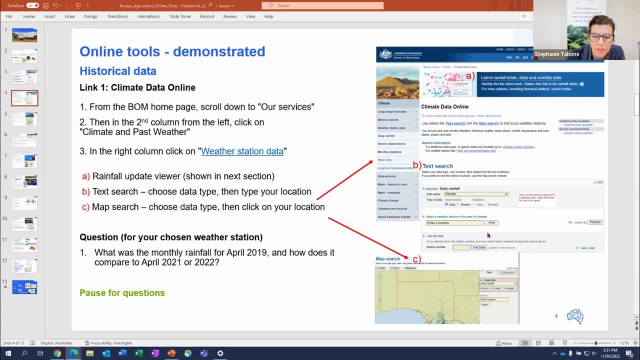 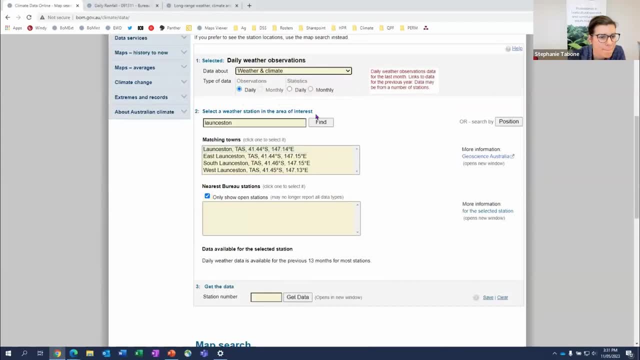 Smith. John, is there any historical data for evapotranspiration, something similar to rainfall? I think you're on mute there, John, Sorry, thanks, Peter. So I think that not all sites will have it, but some of the sites will certainly have it. So if I just kind of go through weather and climate, 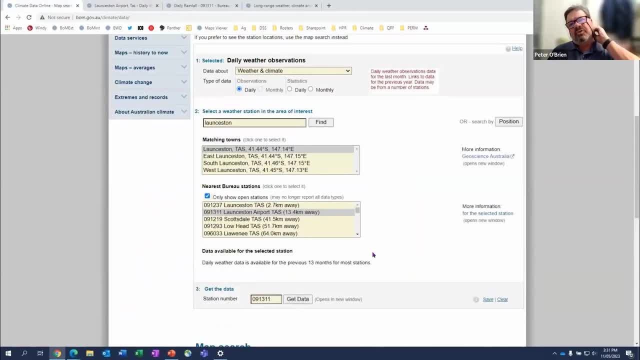 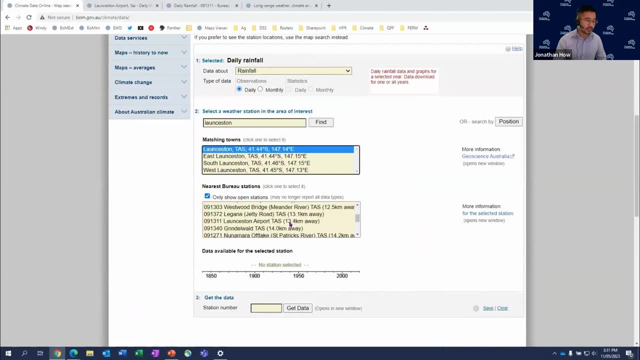 Okay, so it's a lot of the old agricultural sites, agricultural stations have it. I'm pretty sure. Yeah, so certainly, if you go through the main page you can see the last 12 months of evapotranspiration. I'm just not entirely sure of how far it goes back in terms of 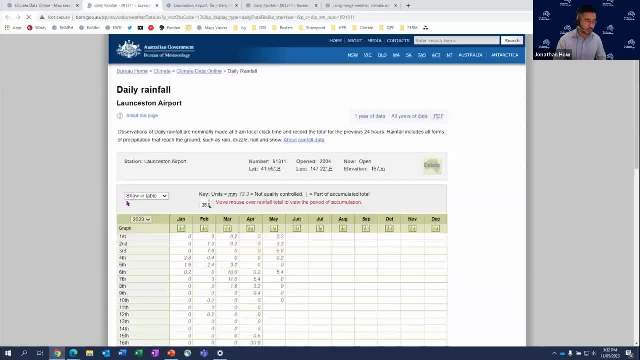 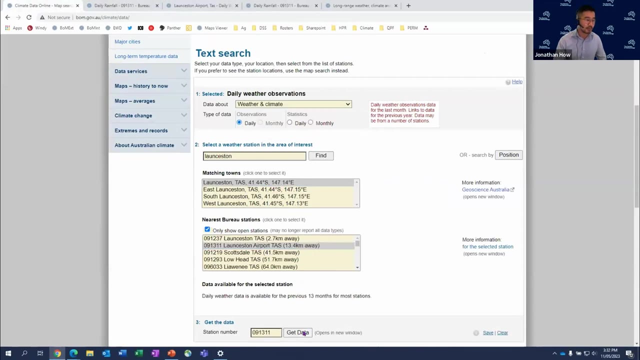 kind of longer term. I'll definitely check on that. Statistics- yeah, I'll have a look for you, Peter, but I don't think there is. I think the main one is if you go, yeah, weather and climate, Launceston, for example, the main way you see it is this: evaporation. 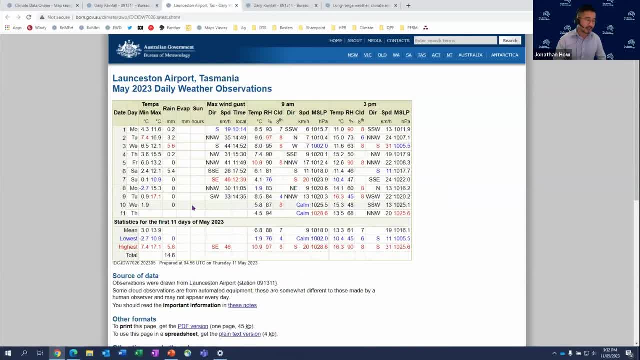 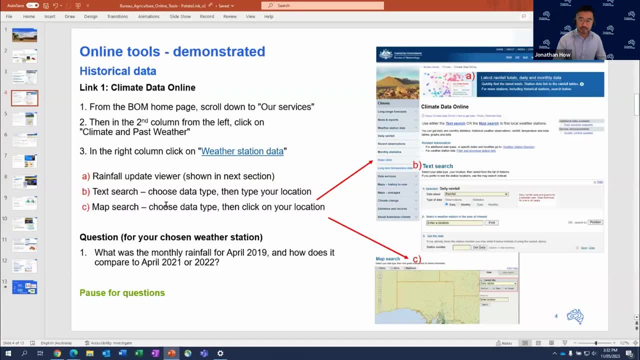 So there's a lot of the evaporation column and not all stations do have it. It's mainly, as Peter was saying, the main one, the main stations and some of the airports as well. So, given that I might press on, Yep sounds good. thanks, John. 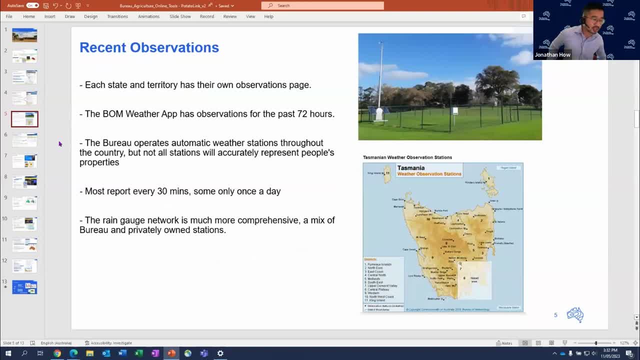 Thanks to the next slide looking at recent observations. So this recent observations refers to anything that's kind of happened in the last hour or the last couple of days or so. So most people will be fairly aware if you've kind of looked at you know. 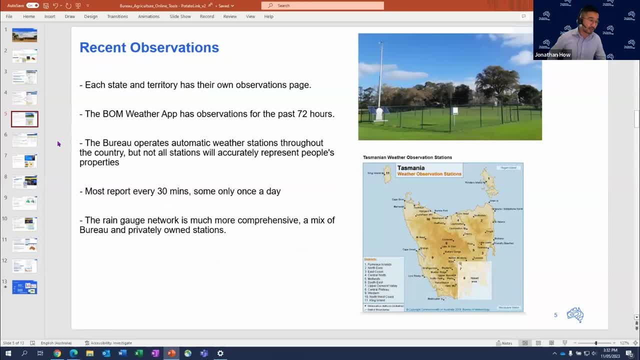 some observations at your place and each state and territory does have their own observations page and the right hand image is Automatic Weather Station. This is the one in Frankston. That's a new one down at Ballin Park in south of Melbourne. Otherwise, if you did use the 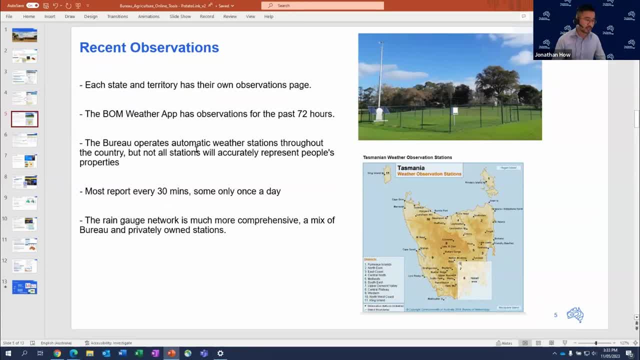 Bond Weather app observations are available for the last 72 hours for all the different locations that we do have before on the app. But it is important to know that the Bureau, even though they have a fairly comprehensive network of Automatic Weather Stations, it's not always going to accurately report the weather at your property. So 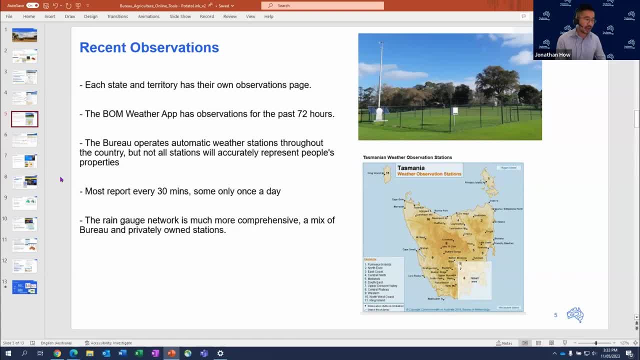 certainly you know we've had chats with many people how the weather station might be five kilometres up the road but it doesn't accurately represent what's at kind of your site. So kind of having an idea of what it can and doesn't represent is really important for your location. 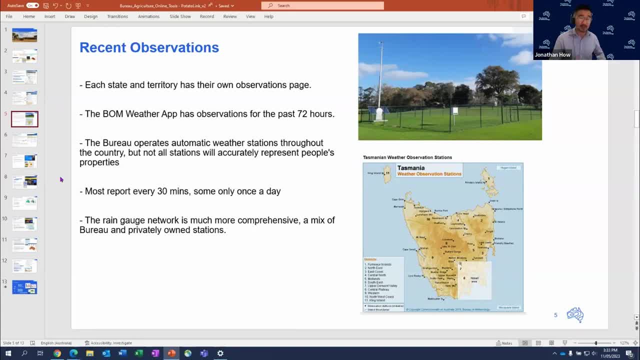 because there are certain things like microclimates which may exist at your property which aren't properly represented at the weather station. Most weather stations report every 30 minutes, so that's a good thing. Some only report once a day, but then the exception to that are the tipping rain gauge. 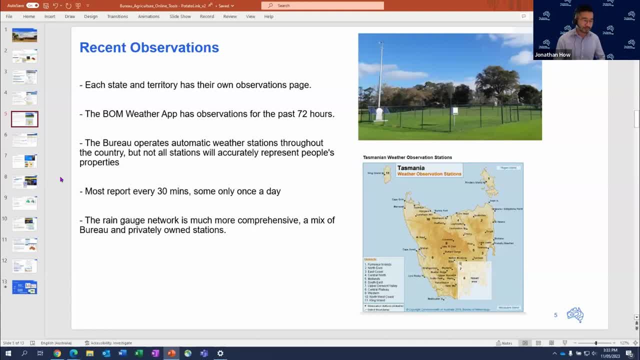 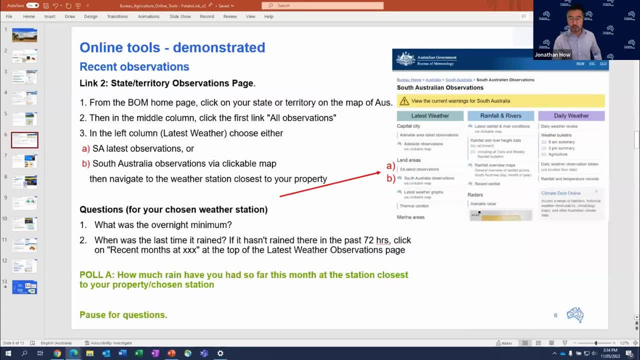 buckets which report every 0.2 millimetres of rainfall, And I'll go through to the next slide. So this is back on the worksheet. So the main way of getting to the observations page- and I've just put South Australia here as an example so I can follow along or just kind of watch on the screen- 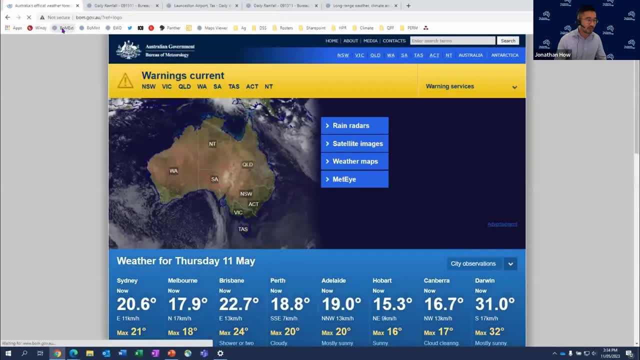 here. So for South Australia again, I'll go back to the BOM homepage. The fastest way is probably to click on the state or territory on this map of Australia. So each little one is a little link which will take you through to that state of territory page. So I'll just click on South Australia and this will take. 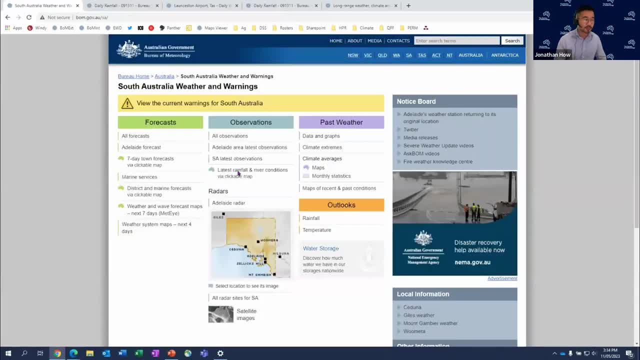 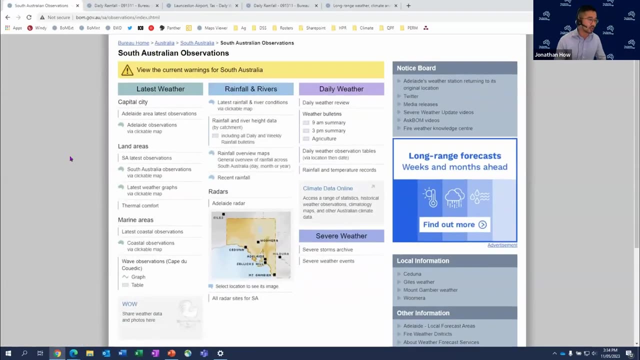 you to the entire South Australian weather and warnings page And what we want is the middle column, this observations here, just in that little white blue centre column, And we want to click on all observations, this first link up here. This will take you to another link showing all the 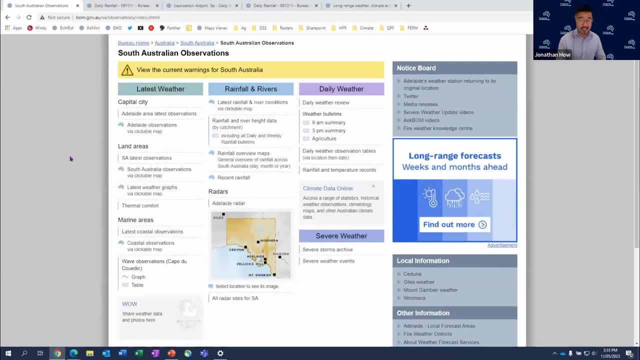 different rainfall, climate again, rivers, as well as temperature and rainfall observations, And so certainly, you know, have a bit of a poke around, if you haven't already before. But for this activity what we want to look is on the left hand side, under the land areas, There are two links which 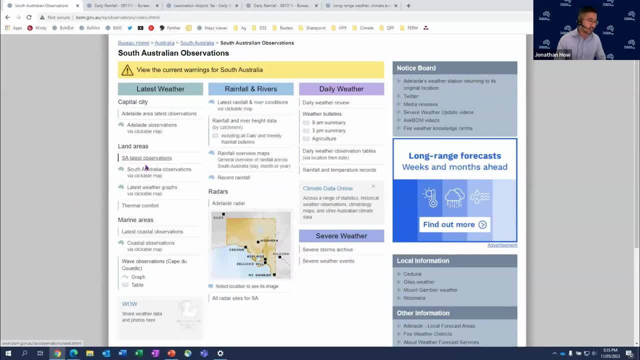 you can use. So you've got SA latest observations as well as South Australia observations. So the main difference is that one's a map and one's a table. So let's just say, for example, I click on SA observations, It takes you to all the different bureau observation sites across. 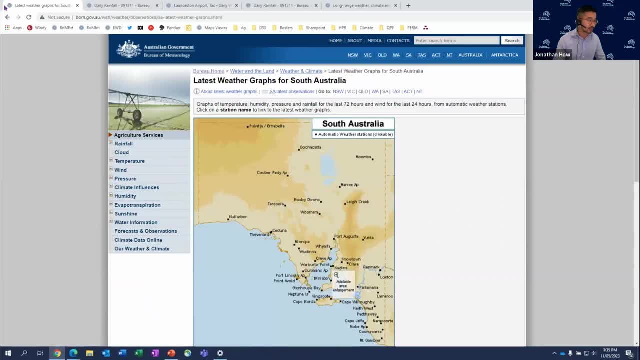 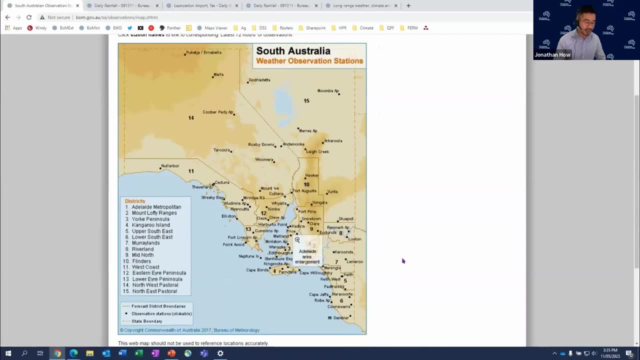 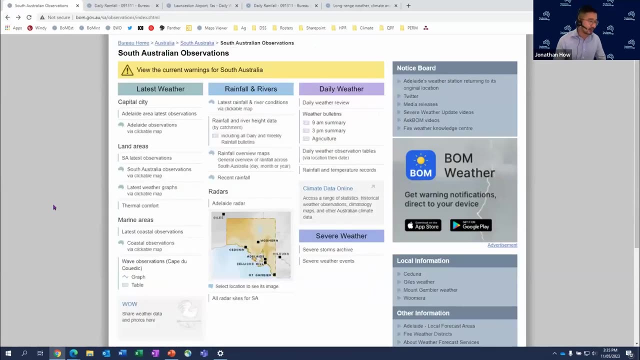 South Australia, whereas the link before takes you to the map, just a clickable map, just to kind of see where you're at, And there's a bit of an enlargement for the Adelaide area as well. So I guess, for the purpose of this activity at the moment, I'll have a look at Redmark Airport. 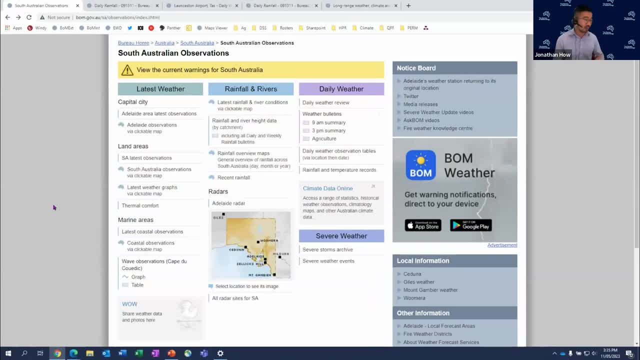 for example, And what we want to see in this activity is what was overnight minimum and when was the last time it actually rained in Redmark. So there are two ways to get to that, So I will show the first way. So, clicking again on latest observations, You can either just do a Ctrl F and 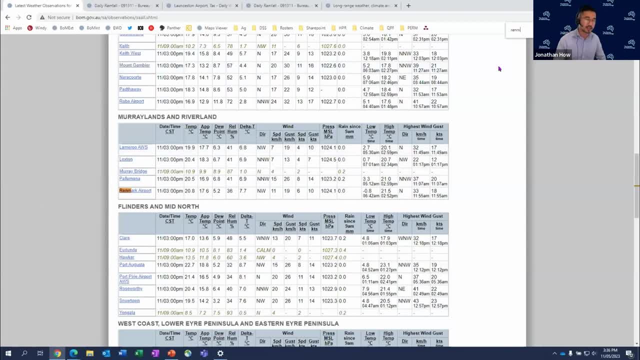 just look for Redmark here or just kind of scroll down. I'm just under Ctrl F, I'll take you down to Murraylands and Riverland. I'll just click on Redmark Airport here. This will take you to the 30-minute map. 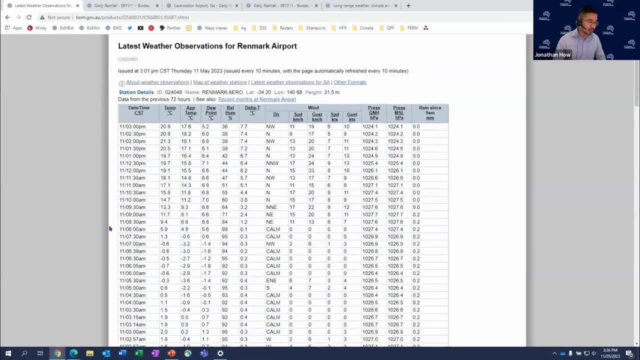 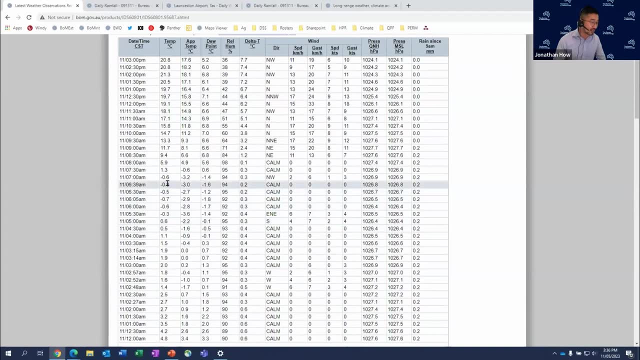 So you can see the data for that station and you know, looking, what was overnight minimum. You need to do a little bit of an eyeball. It looks like the overnight minimum was probably looking around minus 0.8.. But you might have noticed as well compared to the previous page. 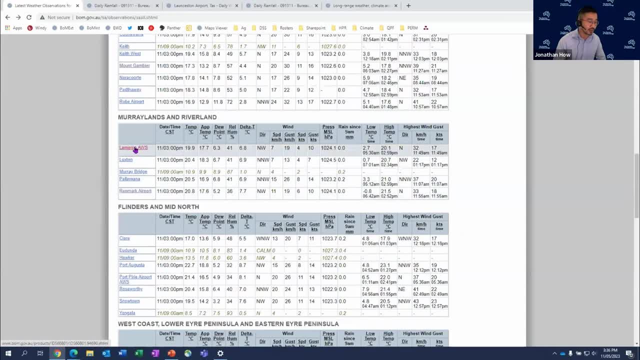 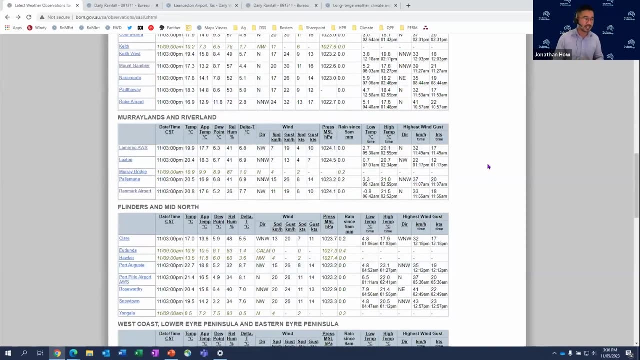 the oh. that's probably not a good example. Let's go to Lameroo. So overnight minimum looks like it was somewhere around 2.8.. Then the previous page said 2.7, and this is a common kind of trick for those not too familiar with the weather stations. is that? 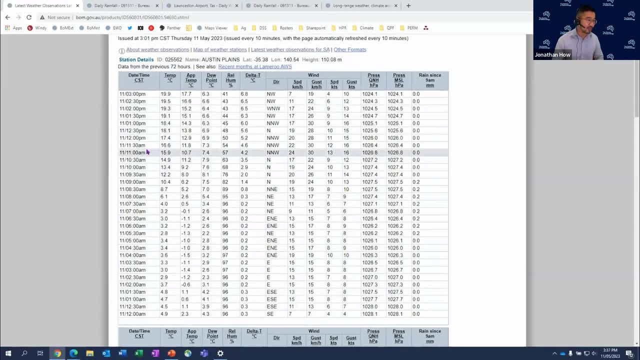 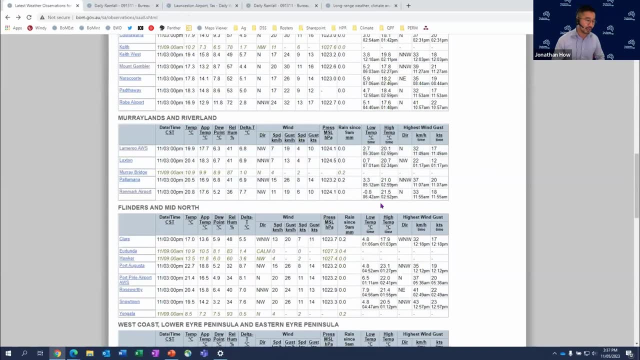 the one this page here only reports at every 30 minutes, whereas the minimum might have been recorded within that 30 minutes. So it is important to kind of look at both that the, what you're looking at, the 30-minute data might not give you the actual overnight lowest minimum, like it did. 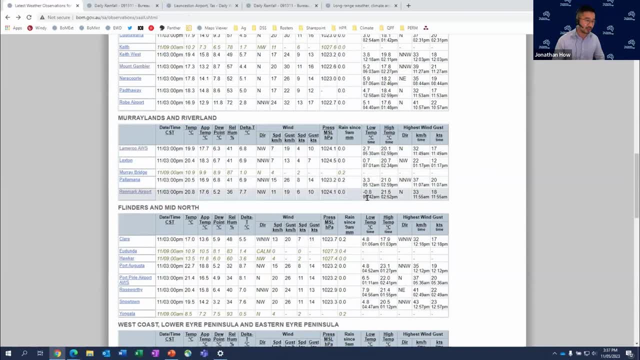 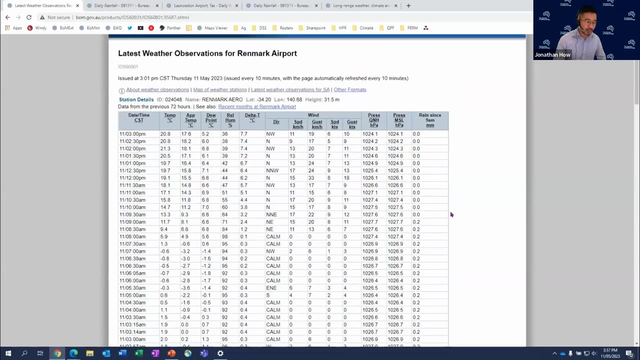 for Lameroo. So certainly this kind of page here does give you the absolute lowest temperature and highest temperature That was recorded in the previous 24 hours to 9 am. The next question: when was the last time it rained? Probably hasn't rained in Randmar for a couple of days, to be honest. And oh, here we go. 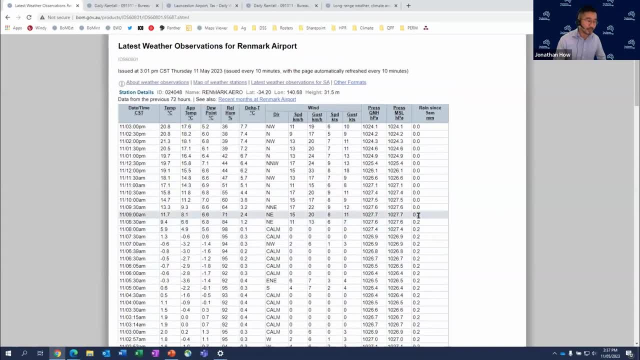 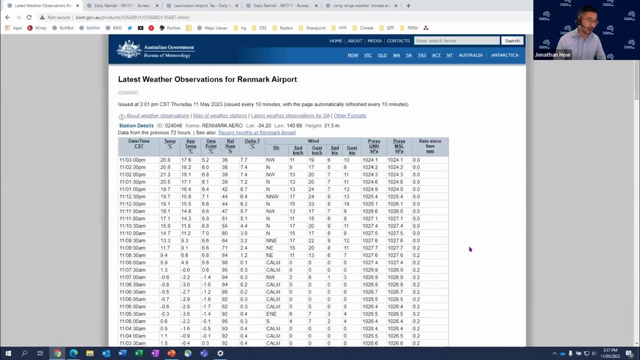 There was a 0.2, sorry, there's 0.2- yesterday through there, But scrolling back it takes you through 72 hours, 72 hours of data. But just say, for example, it hadn't really rained there for a. 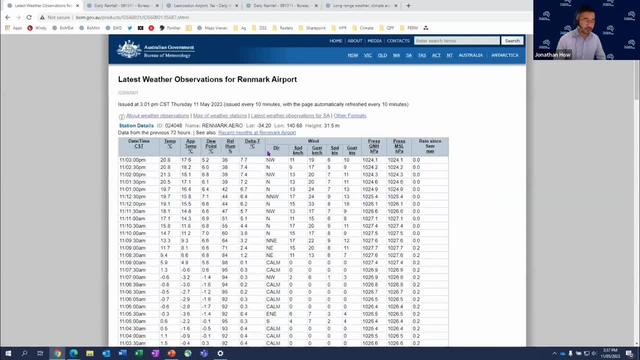 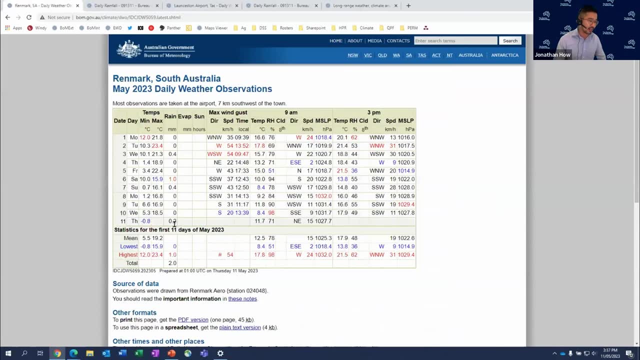 couple of days. What you can do is go to recent months app, just in the top. Clicking on that will take you to all of the day-by-day rainfall observations. So that's that 0.2 from yesterday and just have a look through that rainfall. So this is the same link as the climate website. 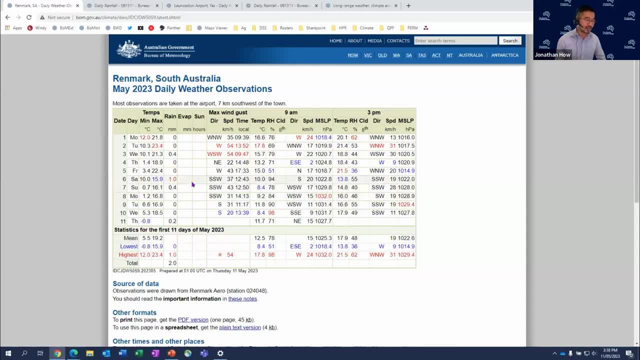 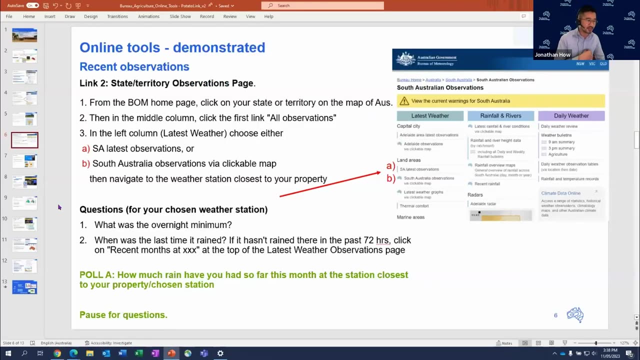 As you can see, the Bureau's website. it's a beast. There's many different ways to get to the different links, So certainly one way is not the only one. This way is not the only way to get to this observations page, But I think we'll pause for questions before going into. 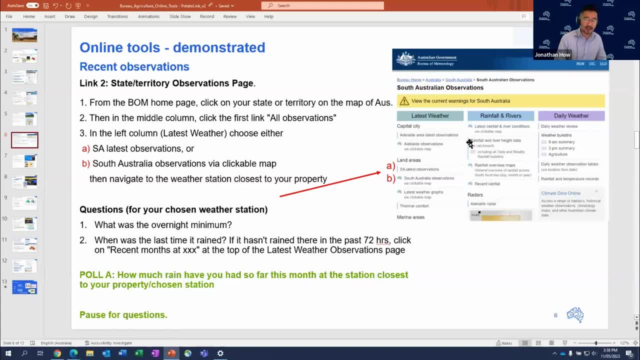 poll A So I can hand it over to you, Steph, to do the first poll. Yeah, just while if there are any questions coming through in the chat again, Peter, is there anything from your perspective? that would be the main reason why growers would. 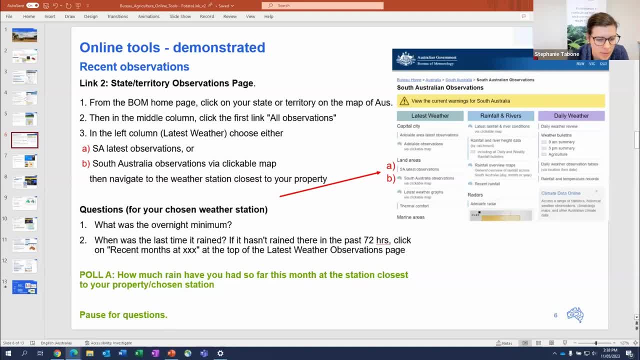 want to be using this tool. We've got Peter on the line. Sorry, I didn't have my At the same time. I think it's. whilst it's obvious that, because they're in the time, in that time, so the observations, but if they have properties some distance away, 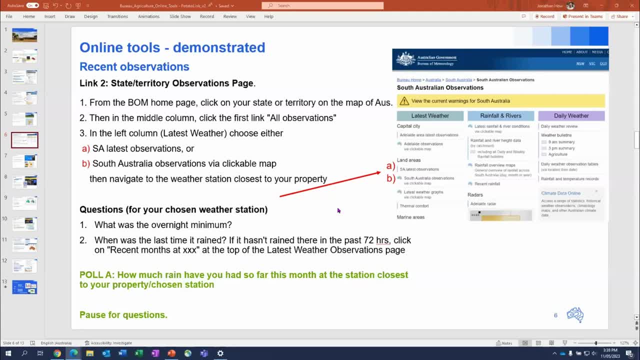 understanding what's happened, particularly in terms of rainfall, frost and the like, is a pretty useful bit of information for growers. Thanks for that, Peter. So the next poll interactive part of the session is: if you've followed along with Jono, I'm going to launch. 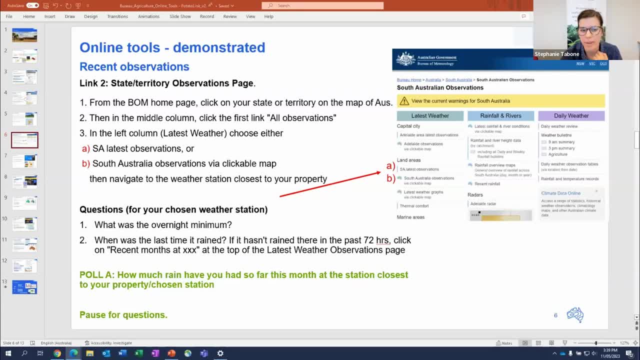 a poll and get you to pop in how much rain you've received so far this month at your chosen location. So bear with me as I share my screen. Steph, there's a question about private weather station networks there. Yeah, sure, I'll have a look. 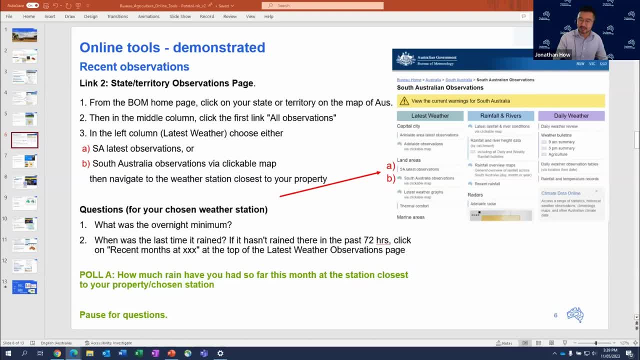 I think that was just someone's response to how they get there with what tools they use. Ah, okay, So Sorry, I think that was just someone's response to how they get there with what tools they use, Right? So if you, yeah, if you followed along, we'll run this poll now. 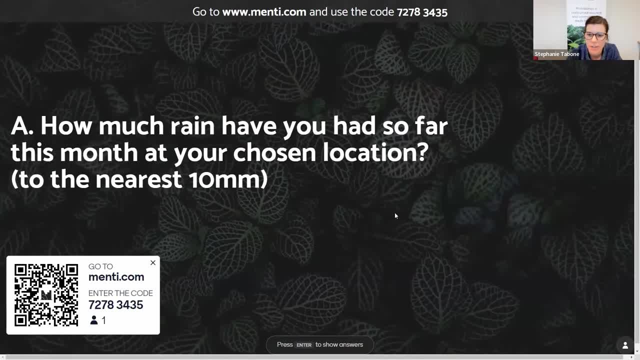 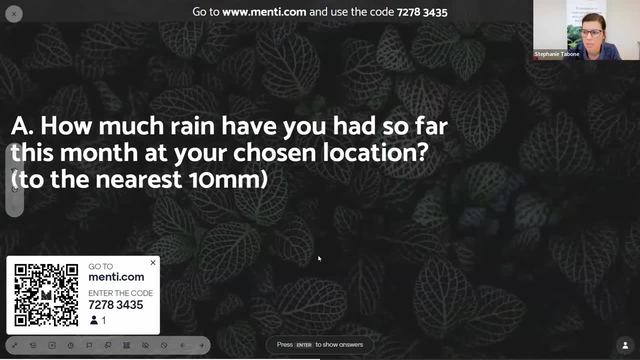 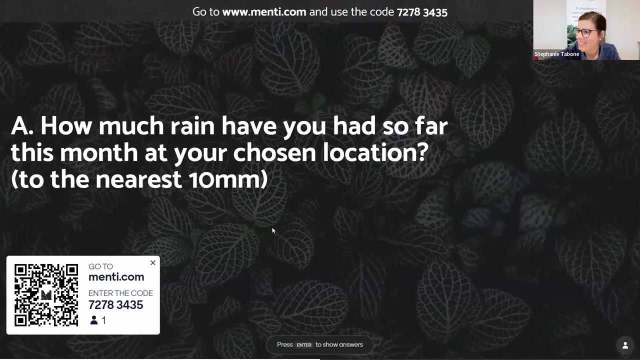 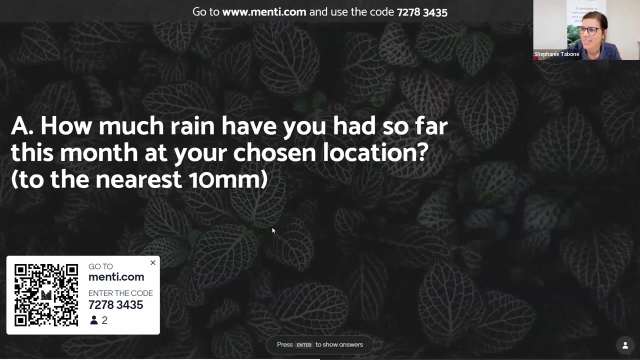 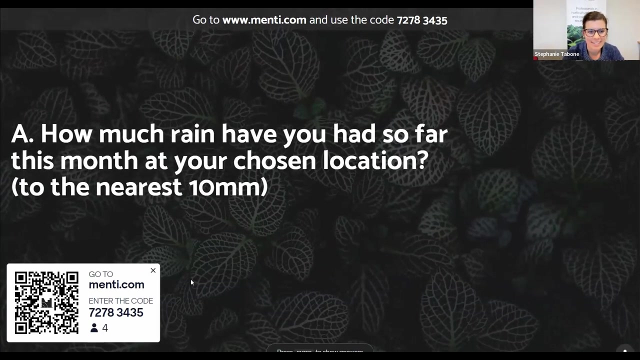 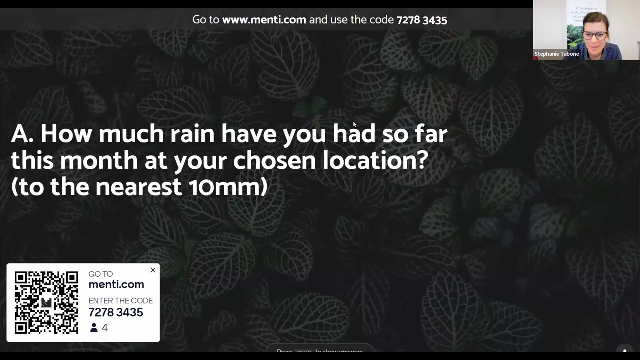 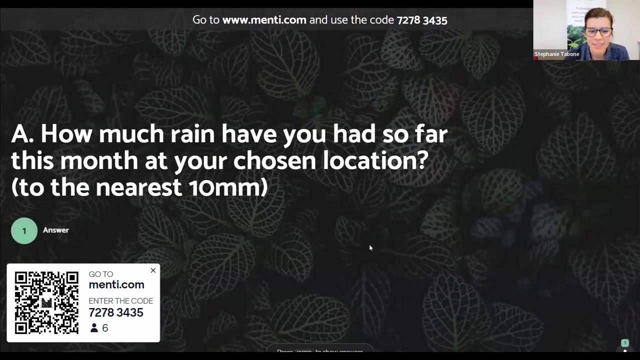 So how much rain have you had so far this month at your chosen location? So, using Jono's guidance and the worksheet to figure out how much you've had, We'll see if anyone's been following along at home. Okay, Maybe just drop me a note in the chat. If you're not following along, we can keep going Proceed. 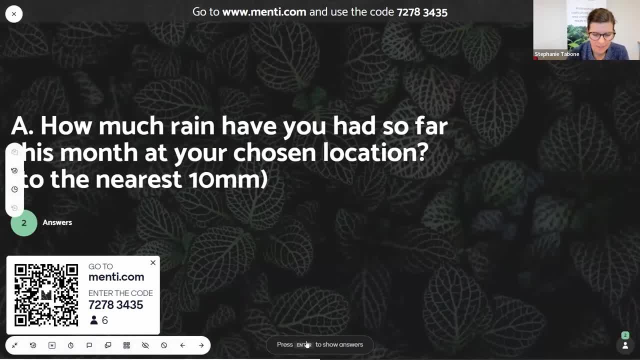 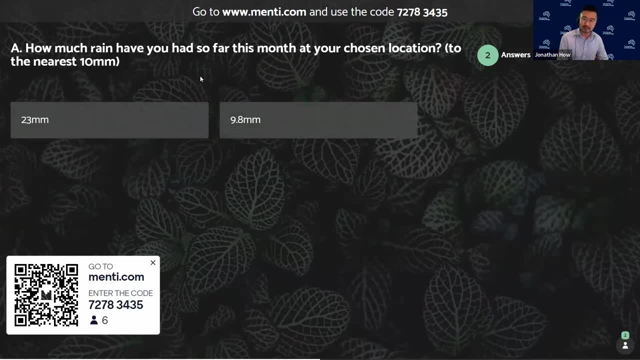 Okay, Okay, Okay. Share the comments. Share the comments. Yeah, most of the rain so far this month's been across Southern Australia. We've had a couple of cold fronts move through Southern WA, Southern SA and Southern Vic and Tas. 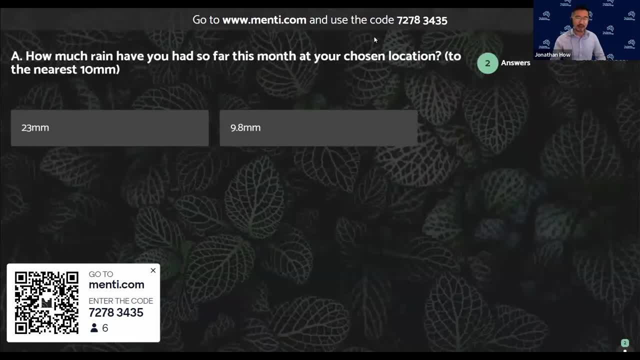 so yeah, for New South Wales and Queensland. yeah, in line with kind of expectations. Yeah, fairly dry months so far, But yeah, looking to be continuing with drying trend for this month for most of the country. So good to see those responses. 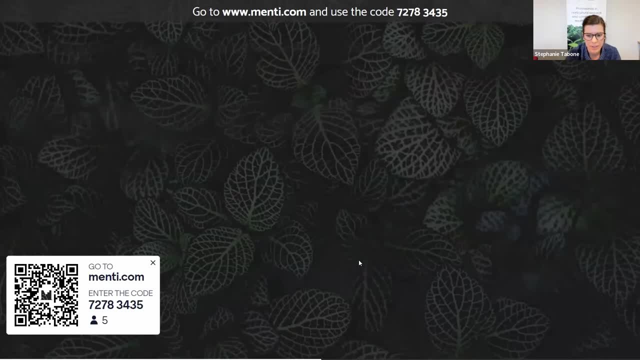 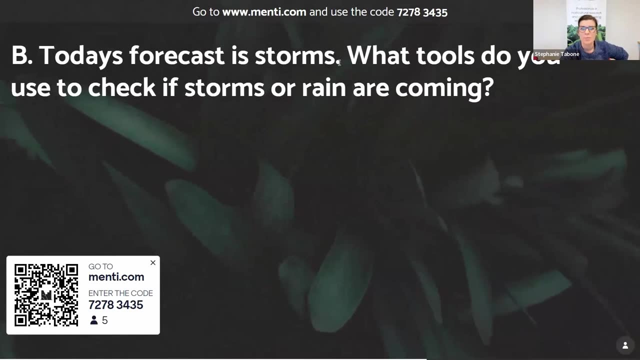 right. so maybe if we proceed to the next question, because i think this kind of moves on to our next uh section that jonathan's about to cover- uh, today's forecast is storms. what tool do you use to check if storms or rain are coming? feel free to elaborate here, jonno. yeah, so just to set the. 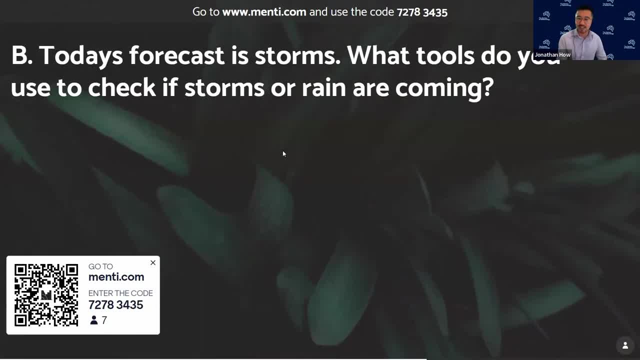 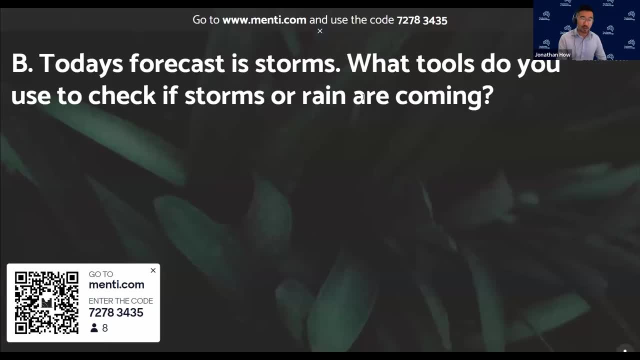 scene. uh, you know, just say you're woken up, turned on sunrise and there's, you know, a storm alert for your location. uh, you know, you're about to step out in the morning or the afternoon and you know, you want to know a storm's coming, you know, to your property or to your house or for your commute. 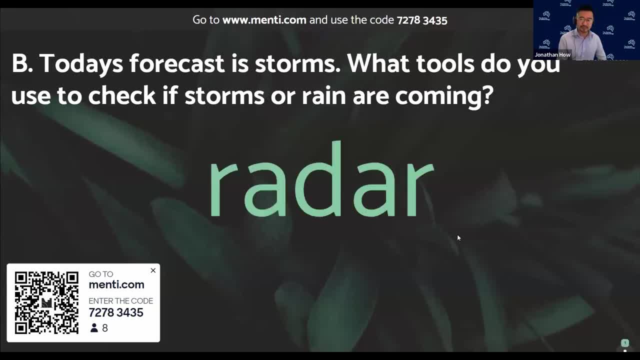 so you know what, what tools are you kind of using to um to figure out, yeah, if there's anything coming at all? yeah, so radar, yeah, radar is definitely um the big one that gives you every six or ten minute updates of um, of the rainfall. so certainly, yeah, that's definitely the main one that you 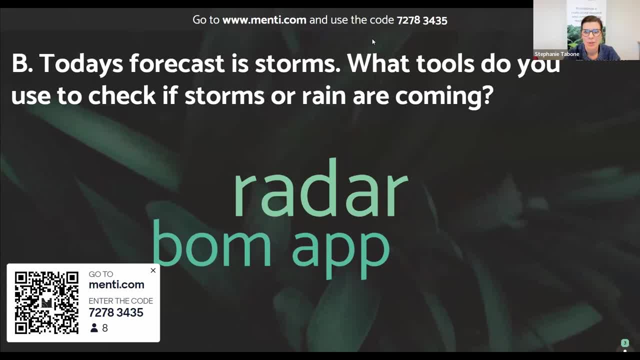 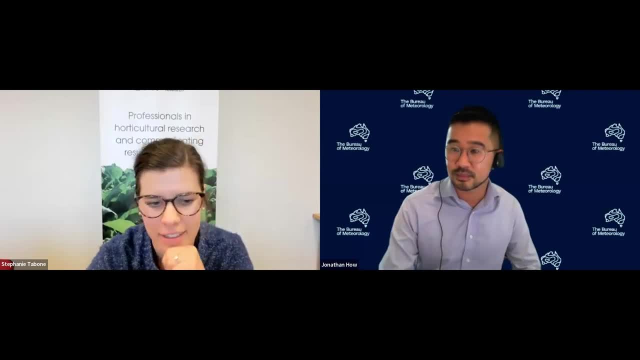 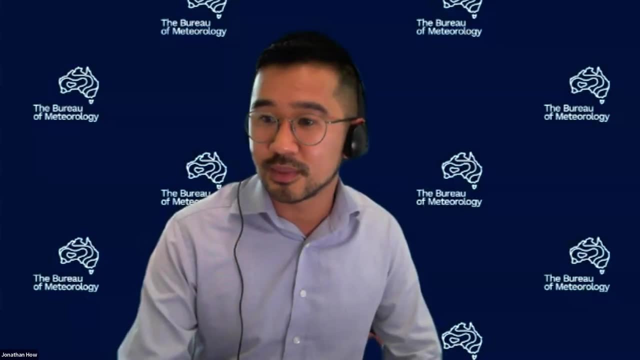 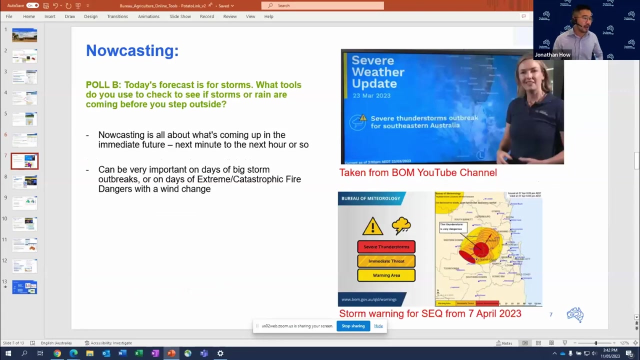 probably use awesome. so we'll jump over to your session now where we'll be covering this exactly. thanks, let me try to share my screen again. so yeah, now we jump across to now casting, and this is all about what's coming up in the immediate future, so anything from the next minute or next hour or so. 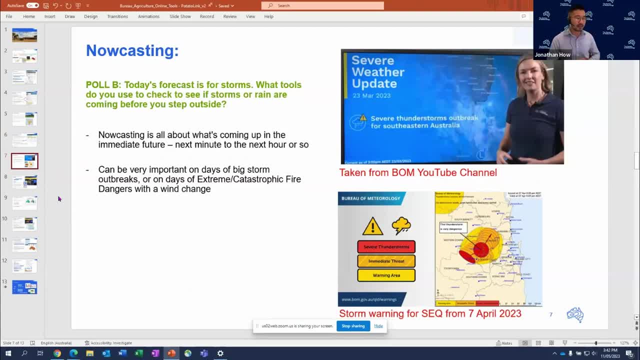 um, now casting is. it's a pretty important skill that um, we um kind of good knowledge to sort of have, especially on days, for example, of big storm outbreaks. on the bottom right was the big storm outbreak across southeast queensland uh, earlier last month with a couple of warnings and there. 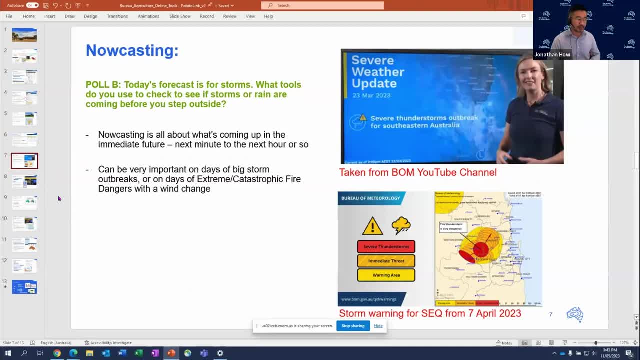 was 11 centimeter hail out to western brisbane as well. so just kind of looking at you know what spots coming up for you from a safety perspective. but also looking at the other end of that, you might also want to know if there's a big wind change coming on, those days of extreme or 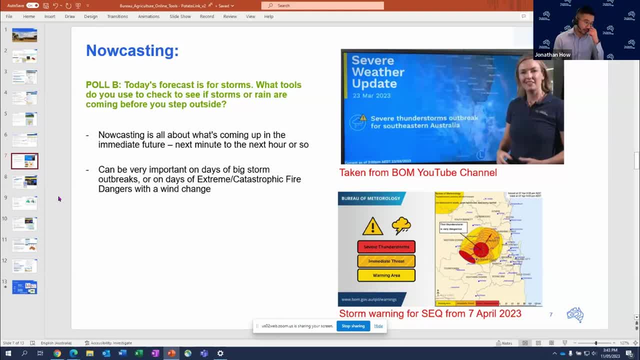 catastrophic fire dangers. you know when is the cold front coming through, when is the wind change coming up? and the top right hand side. the bureau does have a number of different um tools that we kind of put out to the public. we have these severe weather updates, which provide people with a bit of 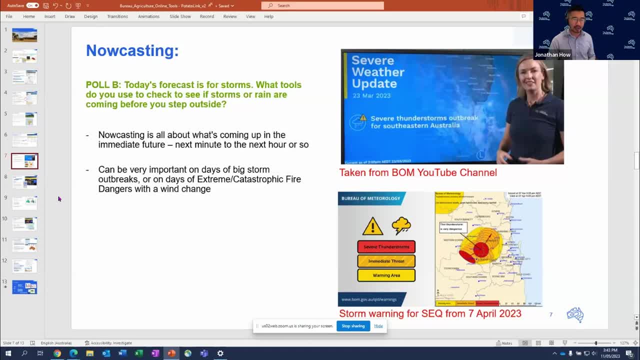 a heads up of something that's coming up. so this is, uh, my colleague sarah presenting from something back in march. otherwise, we do put out thunderstorm forecasts on our twitter page. that's a really good resource for you to look at. so that's a really good resource for you to look at. so that's a really good. 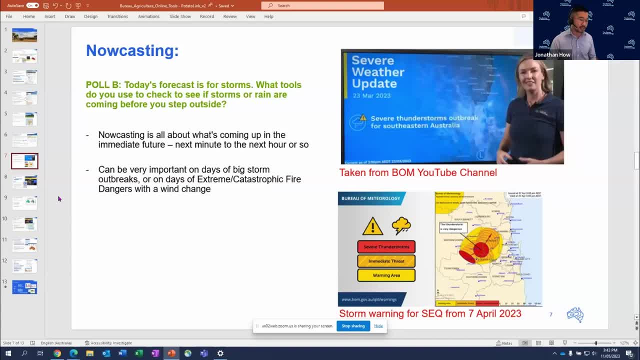 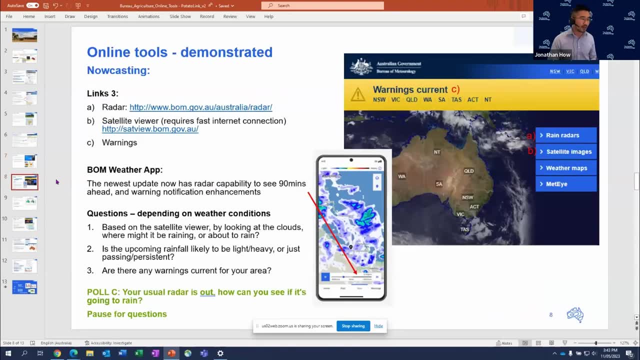 resource for you to look at. so that's a really good resource to check in um ahead of any severe, to check in um ahead of any severe weather, but also twitter itself for warnings as well. so i'll jump straight to the next. now casting slide and yeah, with no surprise, um looking at. 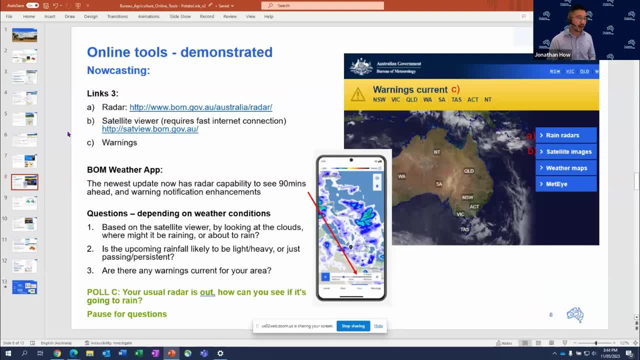 the list, a radar is the number one kind of now casting tool that we do use and the radar link on the bureau's website. it's probably- i think it is- the most used link on the bureau's website. so it is a really important tool, um that everyone, everyone uses, you know, to plan parties or 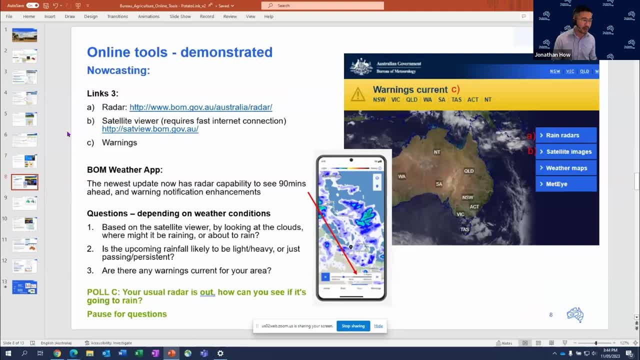 anything to do with other storms and safety as well. but another tool which some people may not be too familiar with is uh tool b, this satellite viewer. so we'll show that in a second. it does require a fast internet connection but it does show um some satellite imagery every 10 minutes. 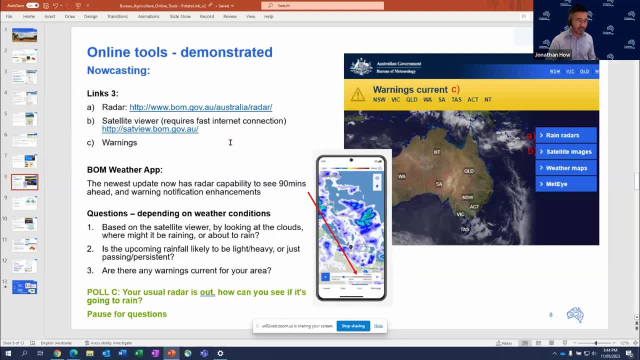 so you can kind of have a look and look at the cloud or look what's coming up for your location. and another really important tool is warnings- the warnings page of what's coming up, but also thinking about the bureau's weather app, we have, in the latest update, introduced this new kind of uh tool. 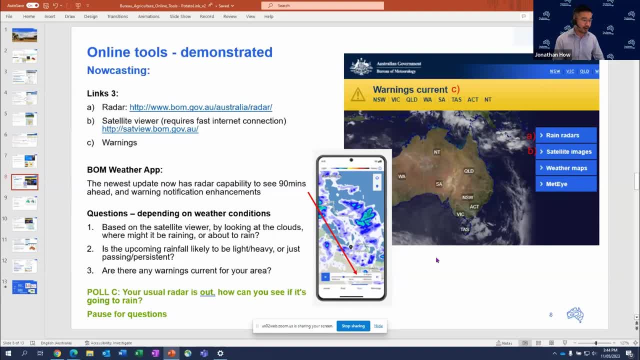 that lets you kind of see what's happening in the next 90 minutes. so the radar on your app will look through to now, but after that it will run an algorithm in the background and kind of give you an idea what the computer model thinks will go, will be kind of coming up in terms of timing and 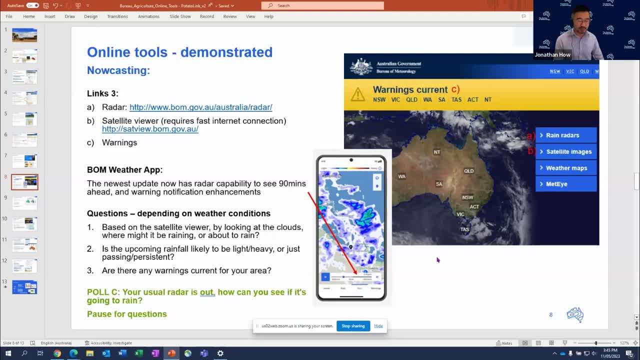 intensity of location. but of course, uh, with any sort of um modeling, uh, there are some limitations. so, with this um- you haven't seen this new rainfall um nine minutes ahead- it won't pick up thunderstorms which develop in the night next 30 minutes. it takes what's already there on the screen and what it does is just 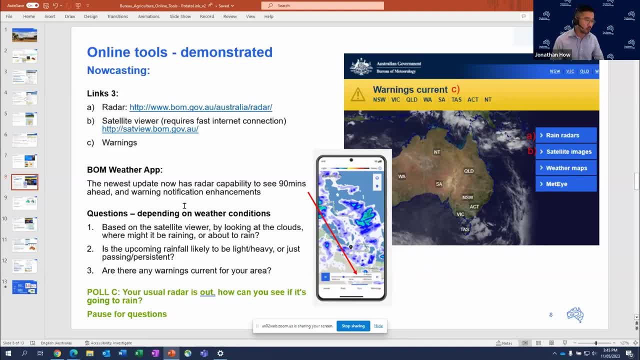 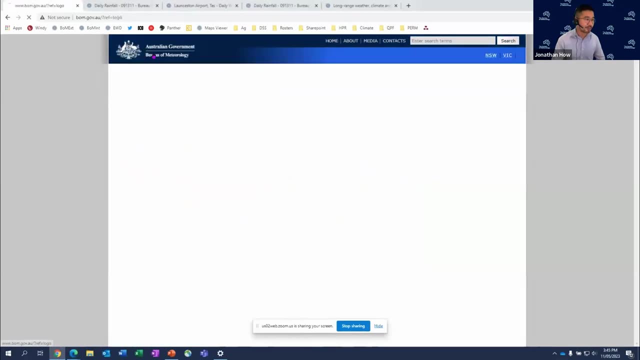 extrapolate it in time, and also in terms of warnings. the latest bureau update also lets you um look at two warnings at the same time. so have been some enhancements in that respect. so what i do is, uh, take you through how to get to each of those. so, starting first with the radar, this is my 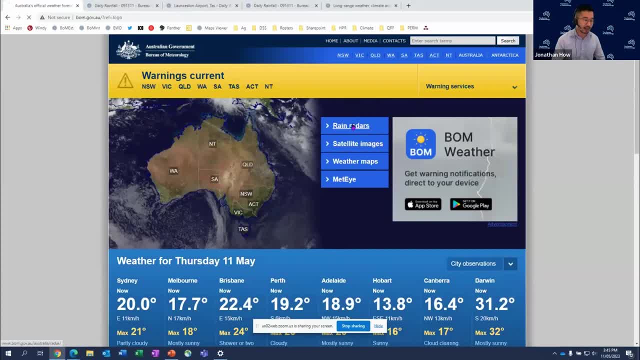 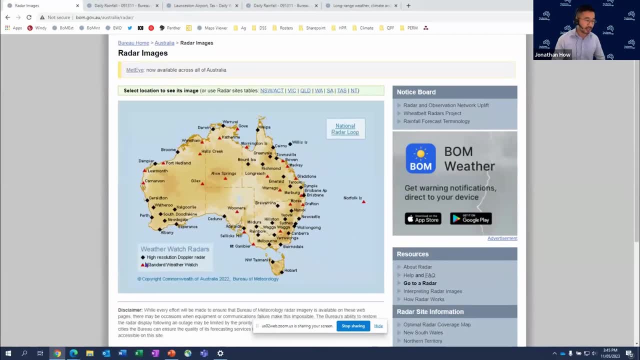 everyone knows and loves on bureau's home page, just under brain radars here and it'll take you through to all the different radars across the country. the main difference between the red and the black radars is that the black ones are the doppler radars, which give a bit more information. 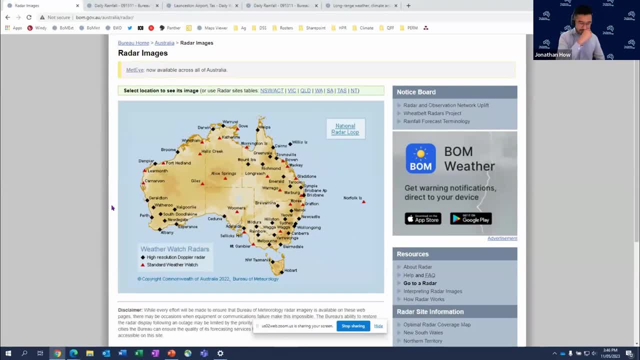 about the wind, for example, anything to do with wind changes, and the doppler radar is also really great for looking at insects as well. insects and any kind of dust avoid the smoke in the atmosphere which can be carried along by others. there's summertime wind changes, but showing you also this satellite um tool. 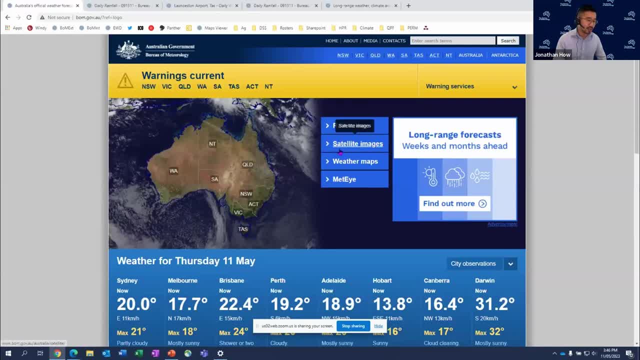 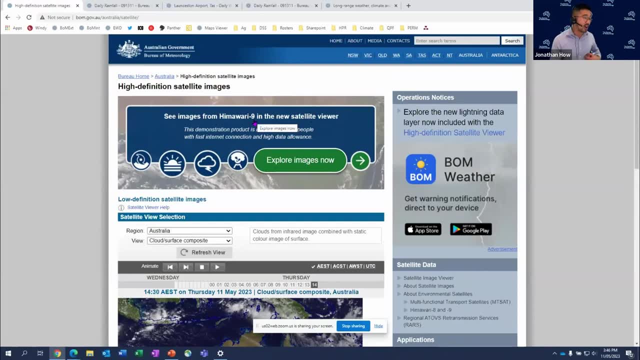 so back on the home page, but right below radars is satellite images. if you click on that it'll take you through to this page here, and this uses the himawari 9 satellite, which is a japanese satellite. um, australia has the fortune of being on the same longitude as japan, so we get. 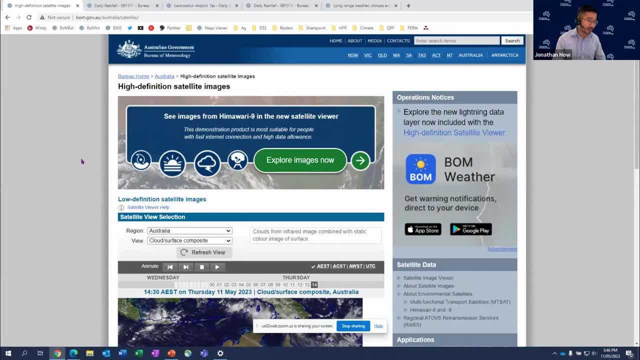 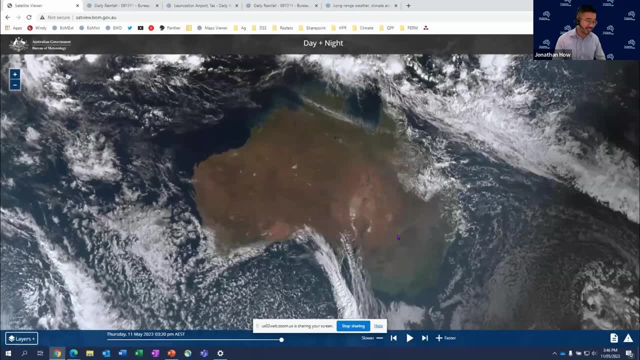 these imagery- high resolution imagery, uh- for free from the japanese meteorological agency. so if you click on explore images now and again, this does require a fast internet connection or mobile network- we'll take you through to this visible imagery. so this is what you'd see if. 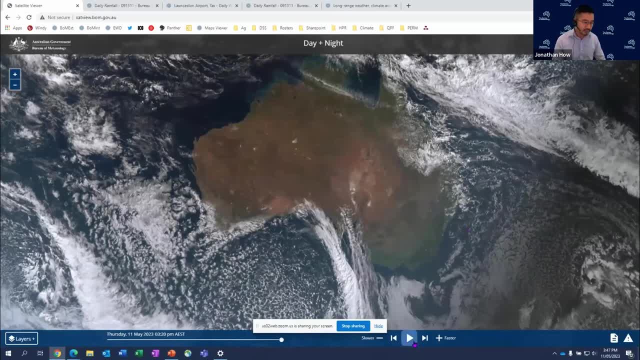 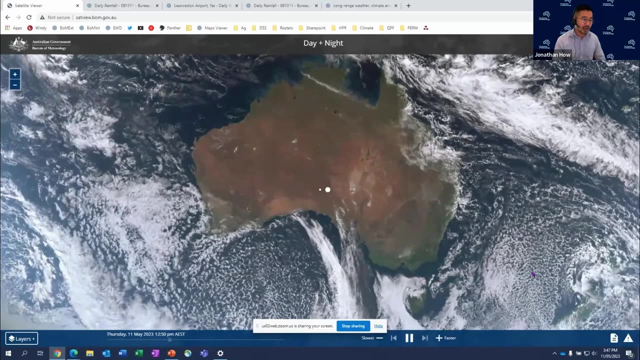 you're an astronaut above the surface of the earth in real time, and what we can do is actually animate that. we take you through every every 10 minutes or so. um, other than being pretty to look at, there are some really great ways that you can use this to your advantage. so just say, for example: uh, you're. 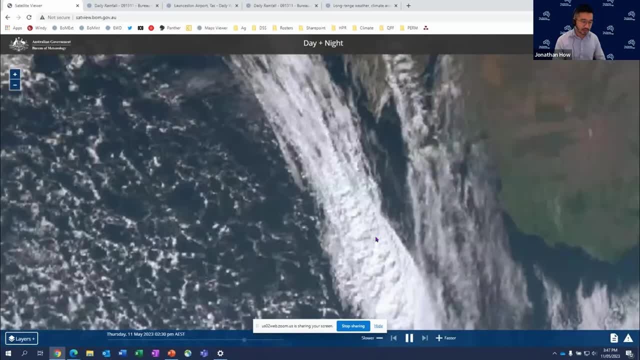 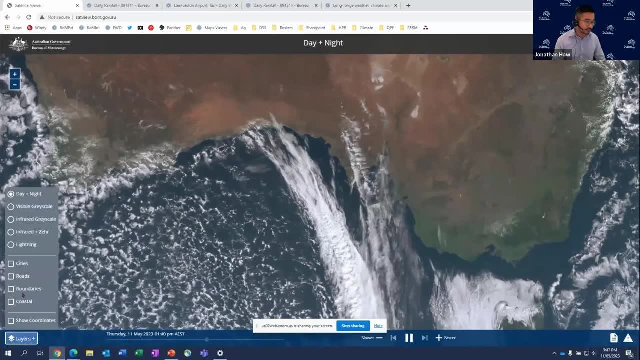 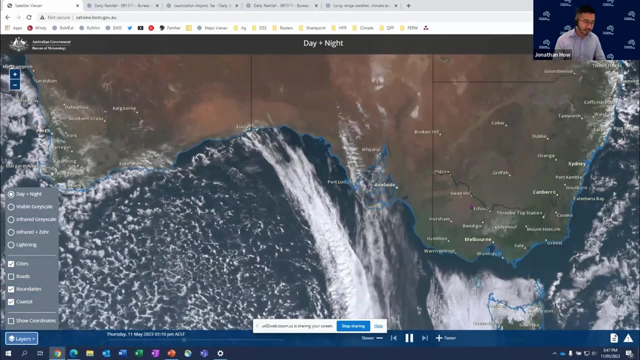 going to look at this most of the time, but having you looking at this for an hour or so is good, or maybe a day or two, but you want to scroll through to south australia. sorry, that's a little bit too fast, um. so what i do is i'll add a layer and i'll put in some cities. 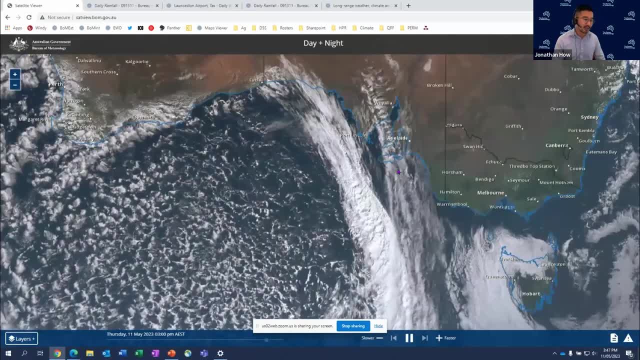 and some coasts and some boundaries. if you want to know, for example, you turn the news that cold front's coming up. where is the cold front? um, you know it does take a little, does require a little bit of weather, um, prerequisite knowledge, but you can basically have a look at cloud and there's that cold front coming through there, just about to get to port lincoln in the next hour or so, and then followed by news btc 06,. it will take a few hours to, it will take a few hours to sit there, and then the next hour or so, and then the next hour or so and then the next hour or seven hours. 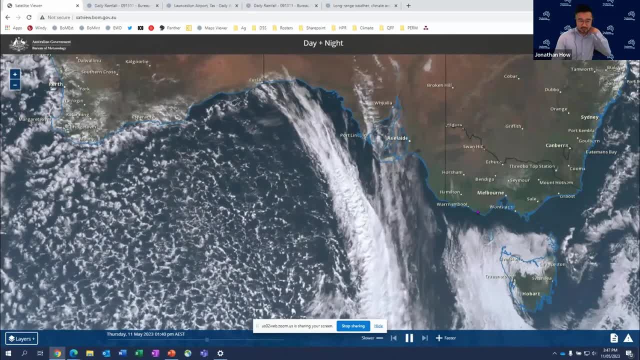 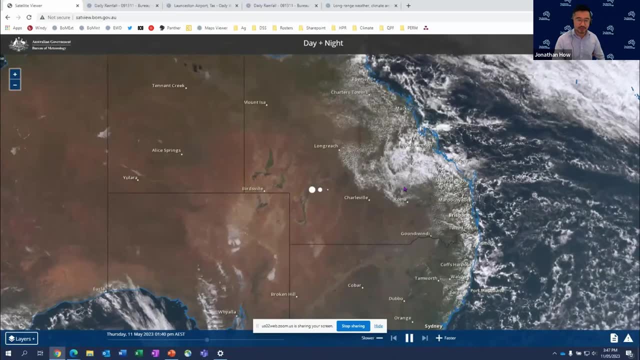 Adelaide and looks to be quite a way off from those in southwest Victoria and Melbourne. so just give you an idea of what's coming up if we scroll up to, for example, up to the east coast of Queensland. we can see here just some clouds streaming onto the coast, and it does. let you. 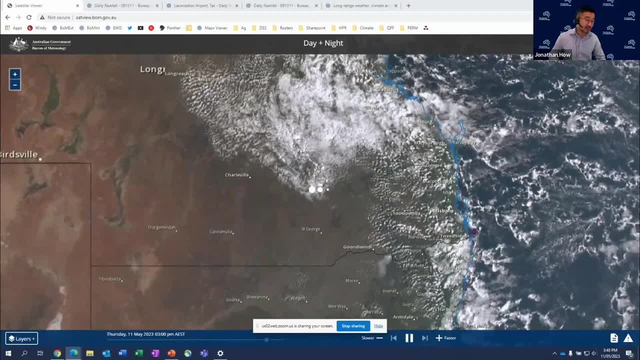 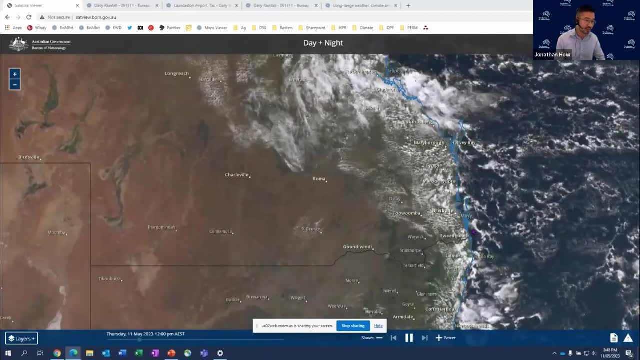 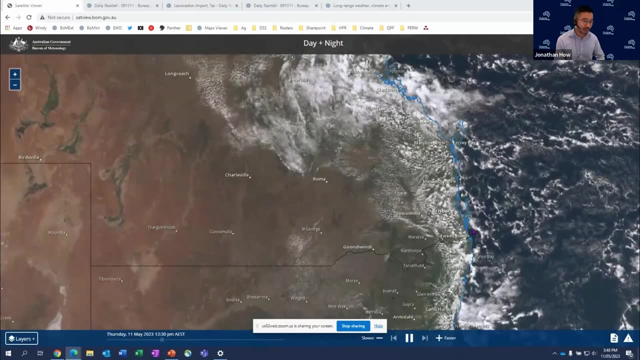 zoom in quite a bit. so the way that I would probably use this, if there's a big, severe thunderstorm day satellite can actually give you a bit of more heads up than a radar can with a storm. so what happens is, before storm develops, there needs to be a cloud basically forming. 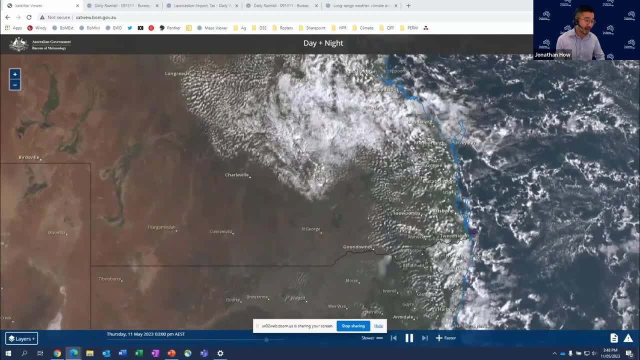 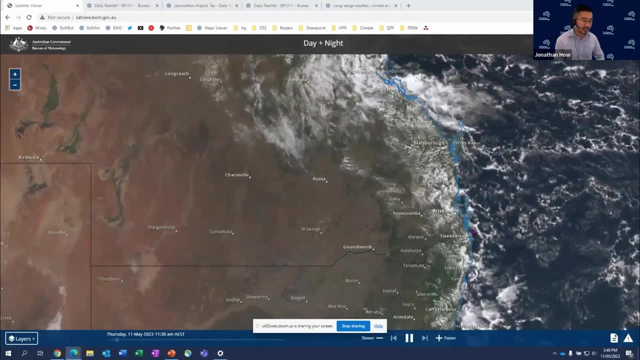 across the land and the satellite will give you that cloud before it starts to produce rain. so it gives you a bit of a heads up of where those storms are forming, and then the radar can be used to see which of those storms are producing the heaviest rainfall. so certainly is quite a good. 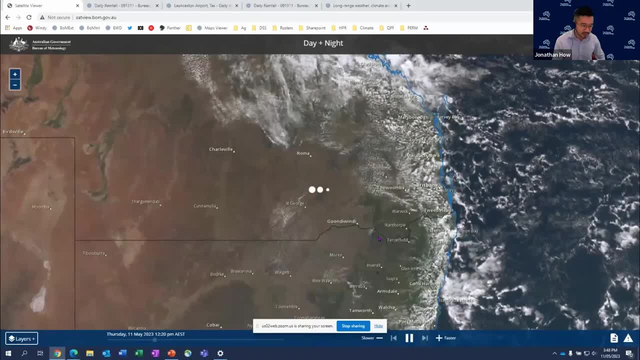 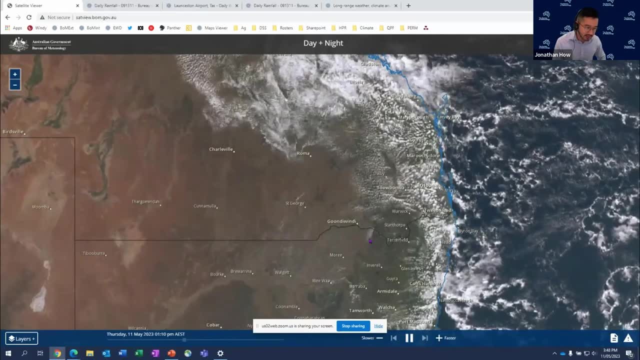 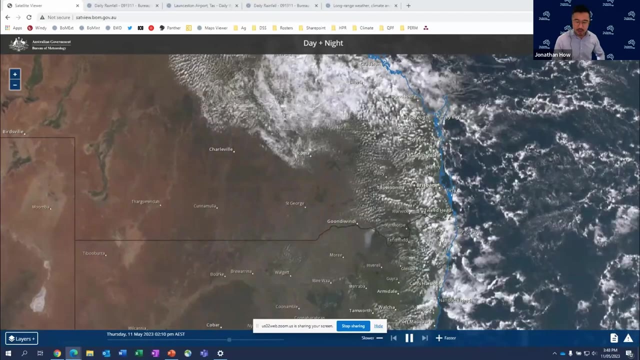 tool you can see here. if I just, if I just you can just kind of follow my cursor there, just the southeast of Gundawindi you can see there's some smoke as well. so this gives you some really great um ability to see a couple of different things on satellite. so, looking at some of those questions, back to the worksheet questions. 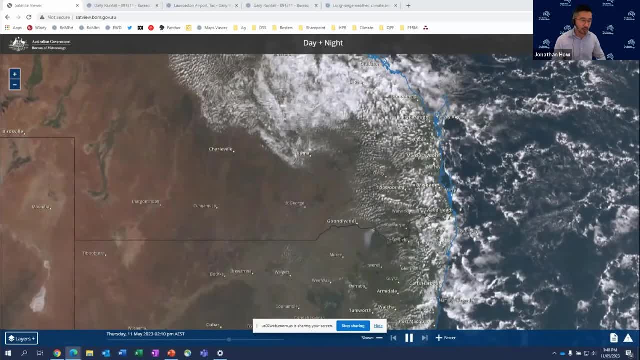 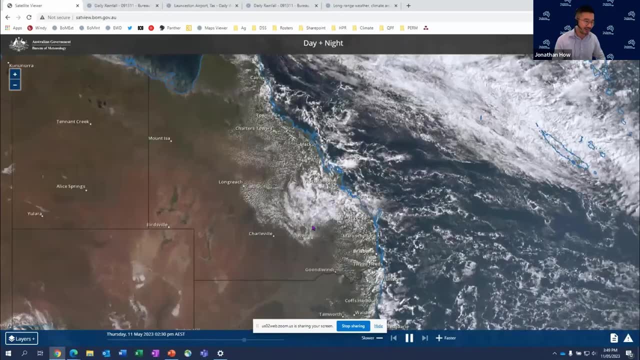 based on link number three, so based on the satellite viewer, by looking at the clouds, where would it be raining or where would you think it might rain? so today's probably not the best example. there's a big high pressure system over the country, but it looks like most of the 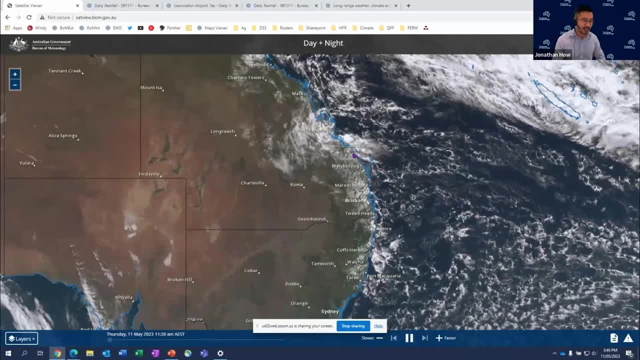 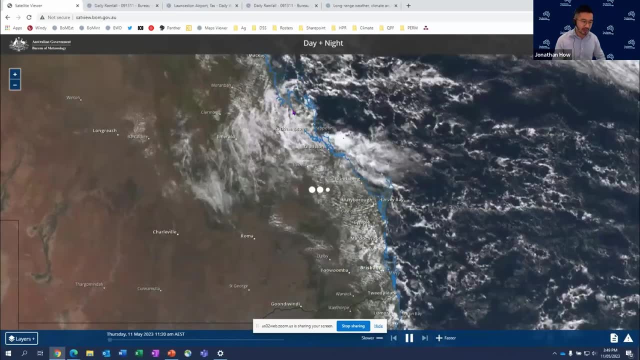 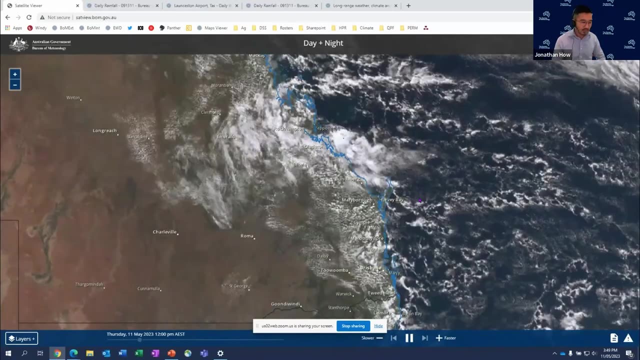 activities along the Queensland coast, particularly, uh, kind of looks. it looks to be kind of north of, um, the Sunshine Coast, up towards Waikiki, and, uh, Rocky up there. so this will give you, this will give you an indication of you know where their clouds, where do you want to start looking. so, um, given that we can kind of go, okay, let's, let's. 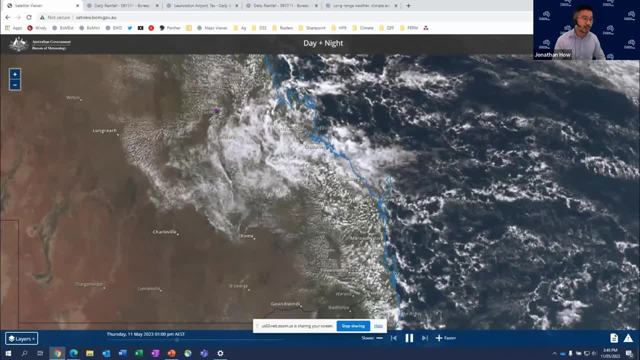 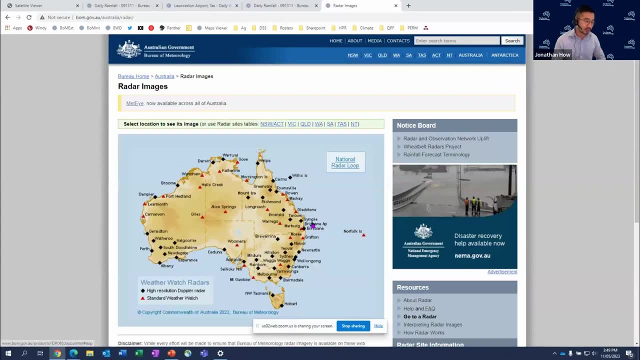 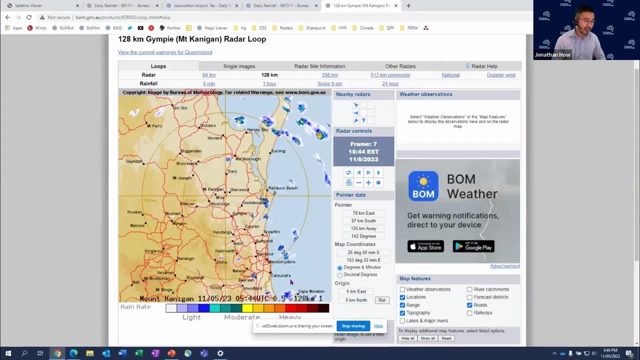 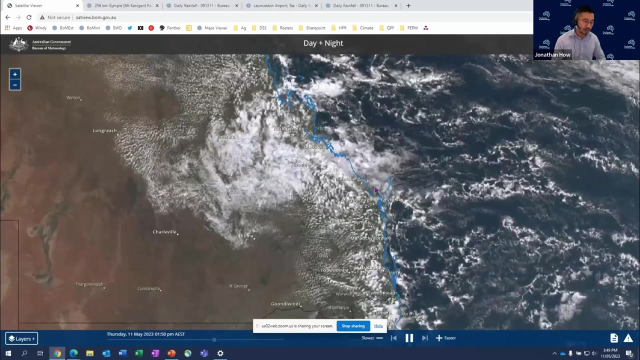 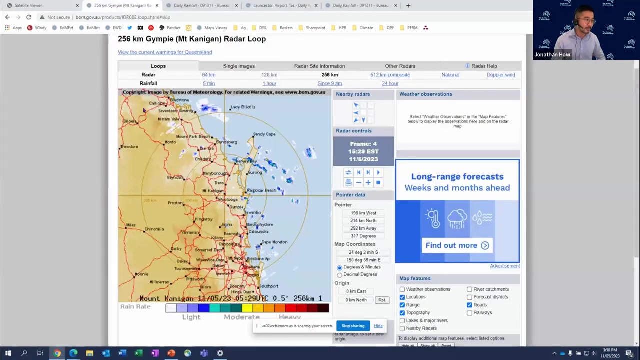 shift our focus to southeast Queensland and look at the radar there. so let's um go back to the radar page and probably you want to be looking at um the Gympie or Brisbane radar. we'll start with the Gympie. so one example that I did was I approached the example over here, especially what you meet, the voltae, and in our case we have some rain showers growing on one side and little leaves are appropriate and we're left limited because the seeing the rain over is obviously a little strange in some of our gegenüber quite rare. Here we go, and I'm here. we have a storm in a small area here in the south wasting. there's a shower deeper here, but if you want to amassascan more 딥, different forcing the flow, dann, and sure enough we do see some stream showers coming through, not particularly. 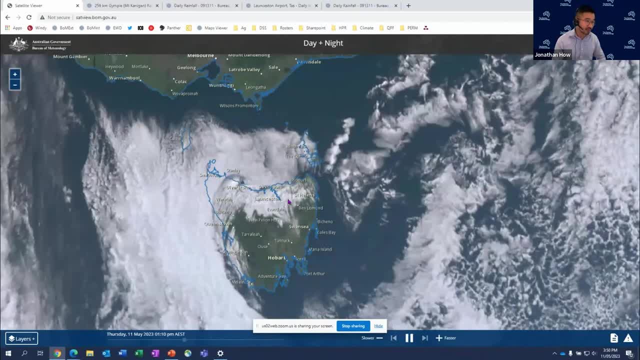 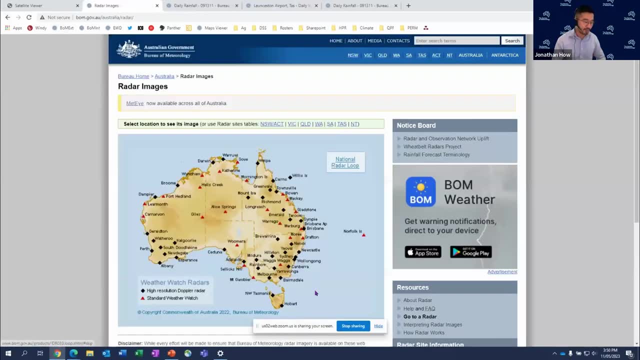 cloud. It looks to be kind of low cloud, so at most probably drizzle, but to confirm that we can actually have a look at the radar. So, going back to this radar here and for Northern TAS, we look at Northwest TAS radar. Sorry, it's unavailable there. It's not a great example. 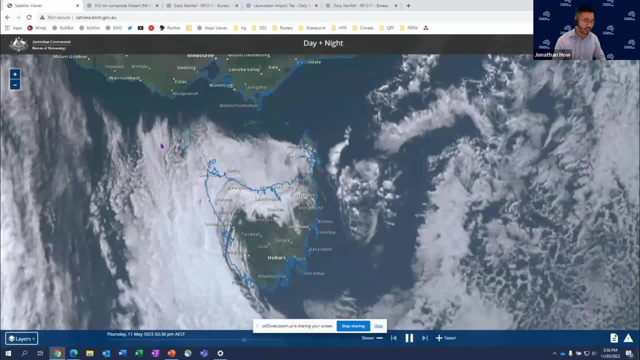 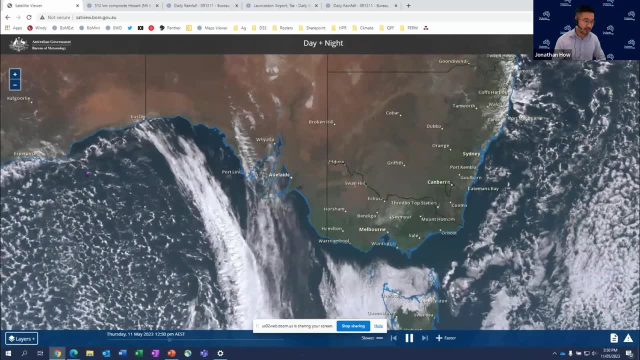 I don't think the Hobart radar goes out that far north, so let's switch and probably have a look at over in WA. Quite a bit of cloud across, yeah, the Albany coast and up towards Perth. So, yeah, is it raining across there? We'll have a look and see. 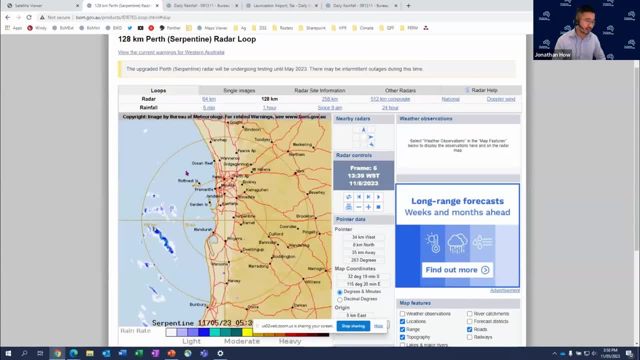 Yeah, not a lot, Not a lot. Everything's kind of offshore, so it just gives you an idea of where there is and isn't rainfall. but certainly I'd still recommend using radar as your first go-to. And then finally, last question, number three: Are there any warnings for your area? 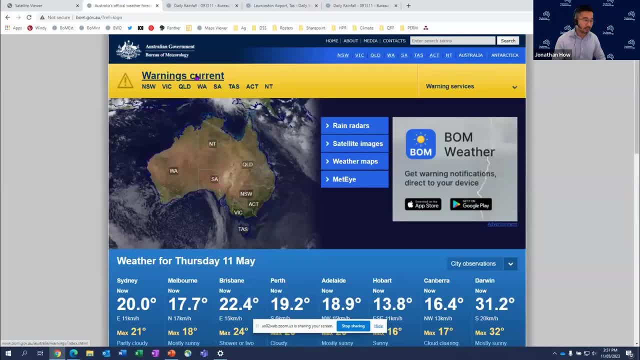 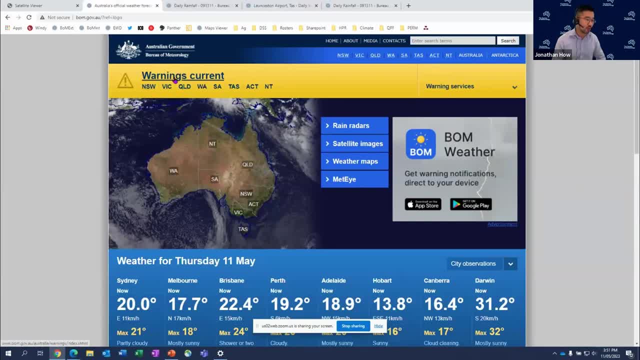 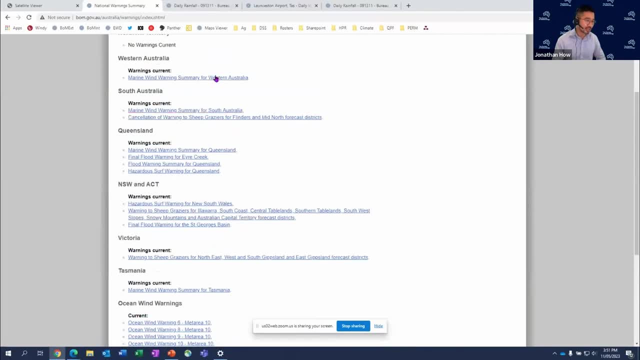 But if I go to the national warnings page- that's that warnings current- you can scroll through and have a look and see that well, there aren't many warnings today and what warnings there are are mostly marine warnings And a little bit of a fun fact. 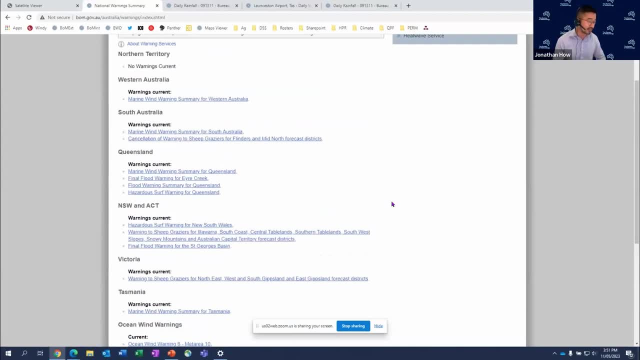 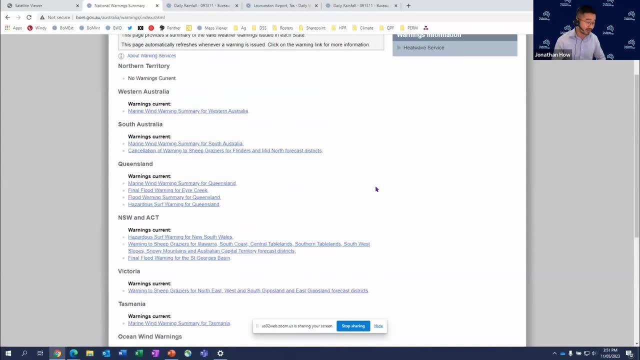 today is actually the first day since September 2021 that there's no flood warning for anywhere across Australia, So it certainly does show that La Niña is well and truly out. So we've had flood warnings for more than a year and a half every day, So that's a fun fact which. 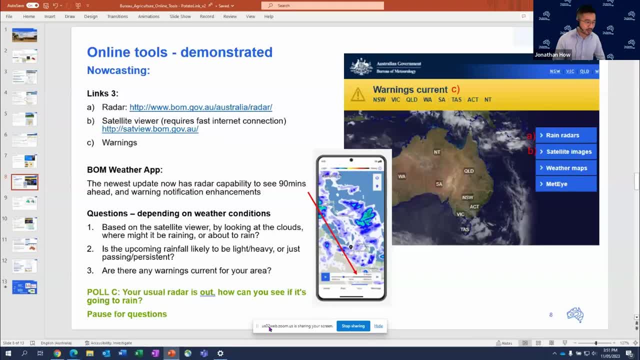 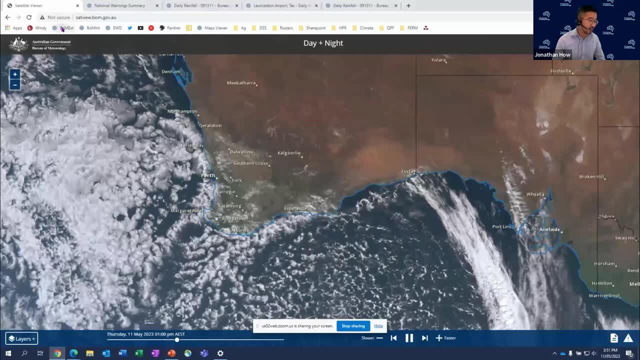 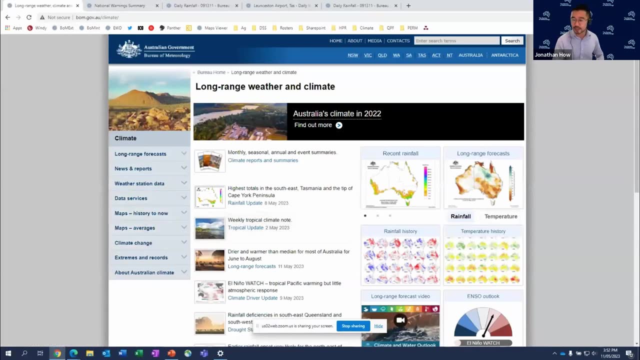 came through this morning. Otherwise, before I go to this policy, I will show. I forgot to mention before this rainfall viewer. It's a new tool that we've got here at the Bureau. So if I want to go back to this climate page, 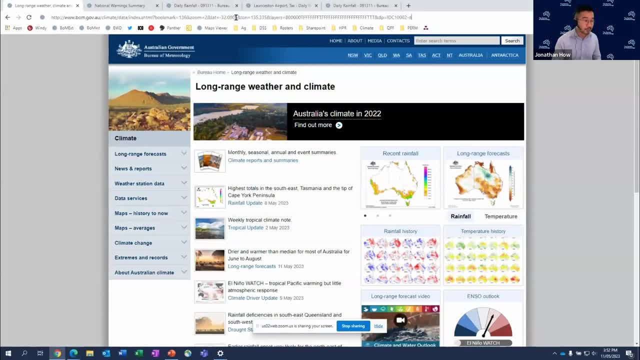 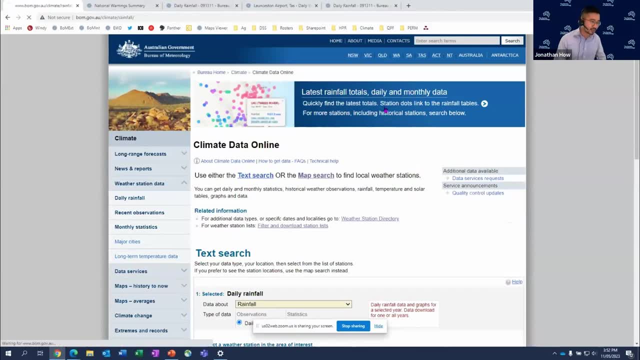 that climate data online link. just pop that in there, So at the top banner here. this is this rainfall update. It's fairly new tool and it came in the last six months or so, but it is an absolutely fantastic tool. So what it does is show you visually all these different 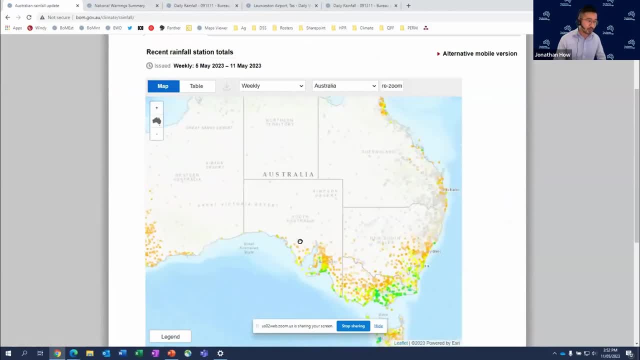 rainfall dots And what you can do is zoom in to see what's happened either daily, weekly or anything up to three years. So, for example, if we're looking at across southeast parts of SA, rainfall for the week to 9 am today, you just go through and click on all these different dots. So 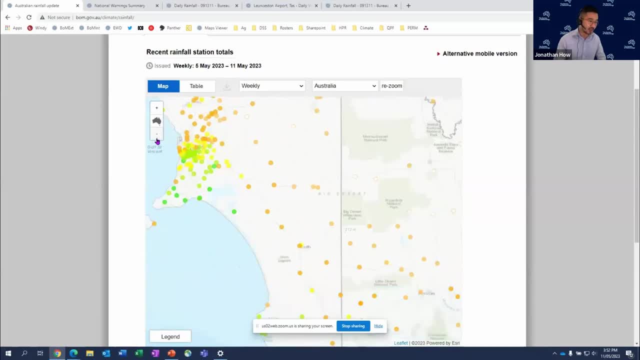 Perunda 6.6,. it's all color coded. It's a really fantastic tool to use if you want to have a look at month to date. This is all the rainfall that's fallen- gives you a really quick snapshot of how much rainfall- and I just have that legend there- how much rainfall has fallen from your chosen. 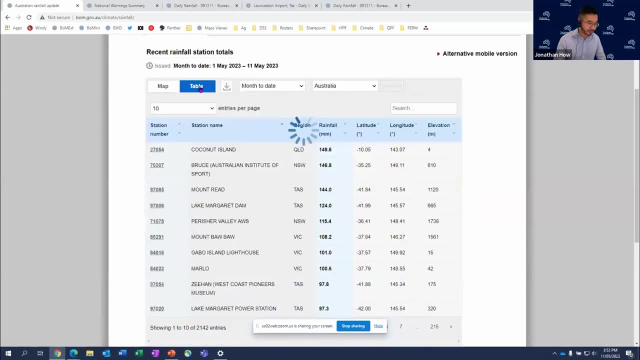 timescale. It's also viewable in table form So you can filter by. you know highs in the country. you can filter by time, also location. So absolutely recommend looking at rainfall update And there's also some commentary which comes through from the climate team. 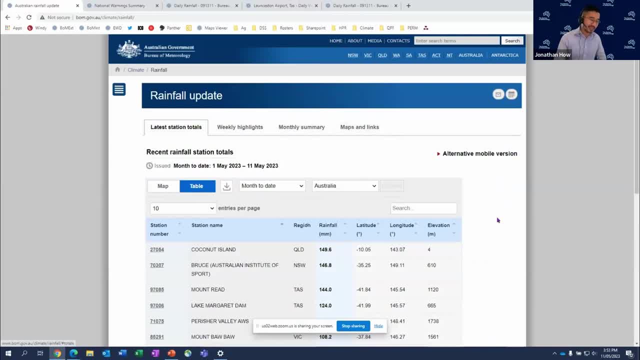 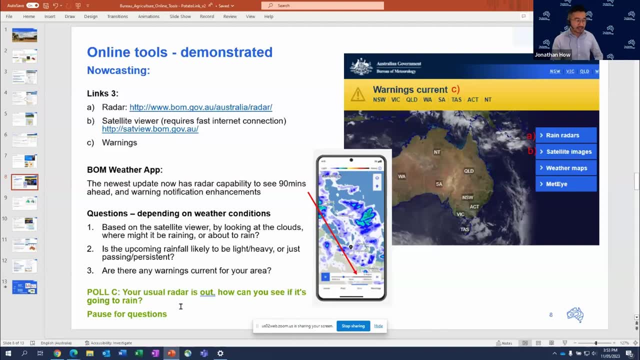 as well. So it's not a very known about tool but certainly a great one if you have a chance to use it. But we'll go back to this poll C So I can hand over to you, Steph, basically asking what you do if your usual radar's out, which we saw across north northwest has. 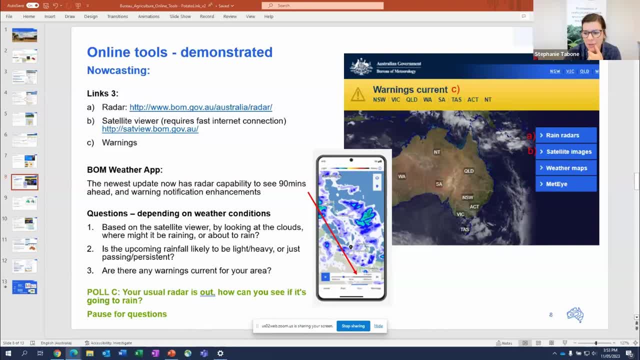 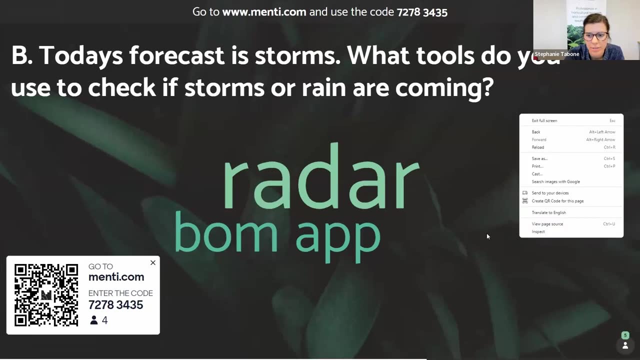 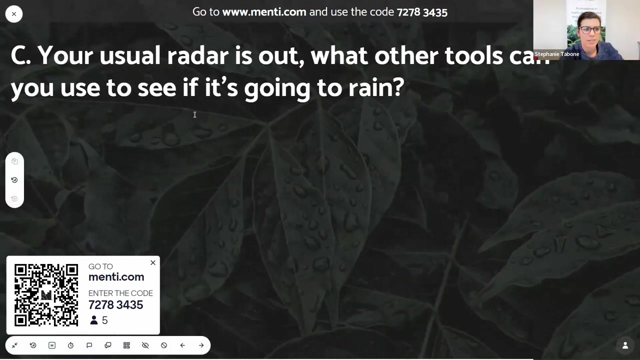 Okay, Feel free to pop any questions on the now casting segment. while I pull up the poll One sec, We'll just progress to the next question. Okay, So if you're able to jump onto Menti, your usual radar is out, like what we saw in Tassie. 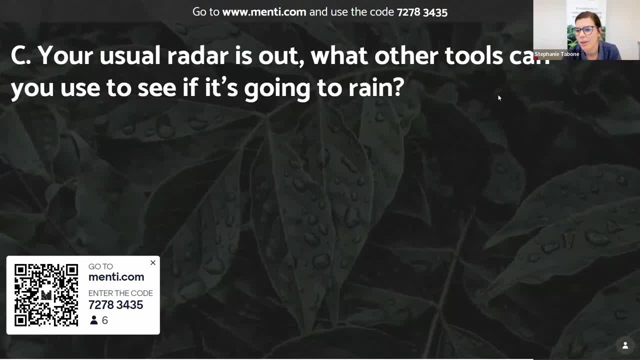 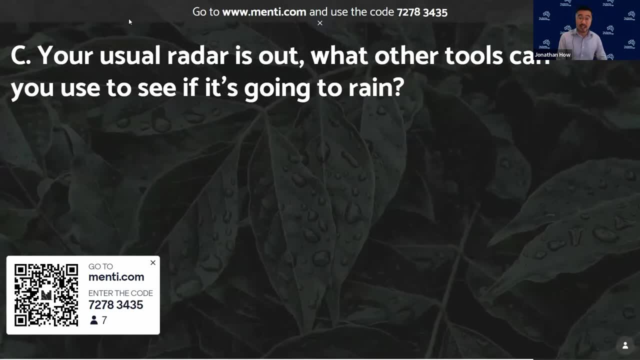 What other tools can you use to see what's going on if it's going to rain- And this can happen from time to time- You know there's radar makes, as we should normally schedule, And you know in Darwin, for example, the radar maintenance was done during dry season. 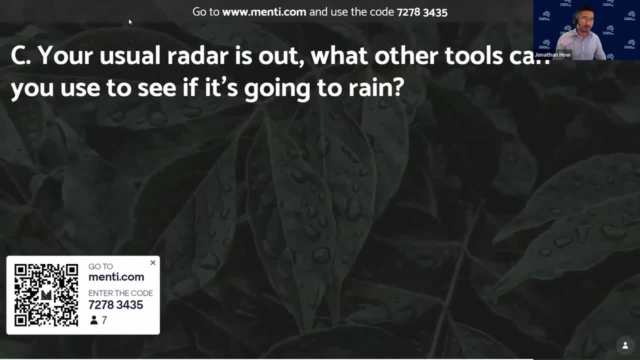 So it can be out for a month or two at a time. So yeah, just kind of find out, you know, if you want to see if it's going to rain, how you're going to find out if the radar you normally use. 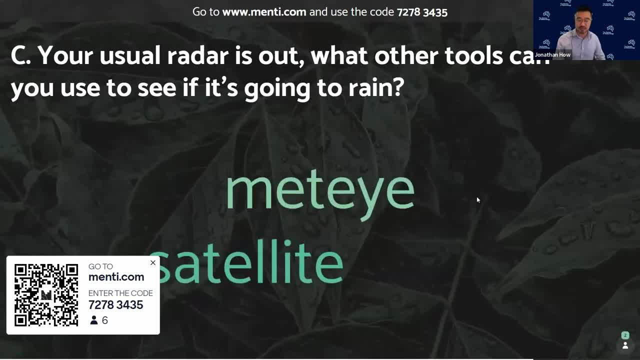 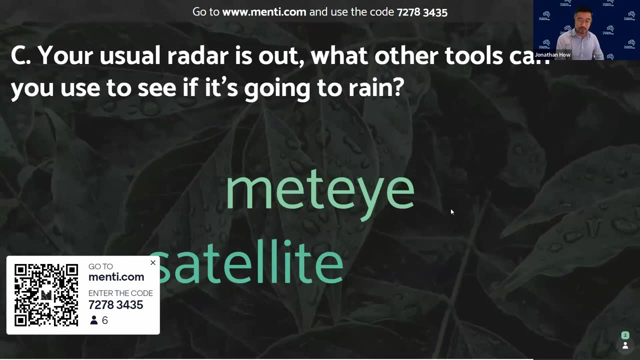 is under maintenance or broken. Very good, We've got satellite which you just showed there. We've got a response here, MetEye. Okay, Any other guesses? Yeah, So it's certainly. those are some really great ones to look at Also. 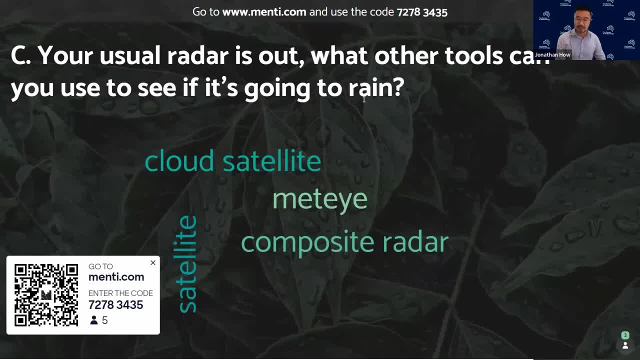 if you look at the national radar, yeah, the composite. exactly The composite tries to piece together all the different radars which are active to somehow, you know, sometimes a bit of overlap, particularly across Southwest WA with the new network. quite a few new radars There. 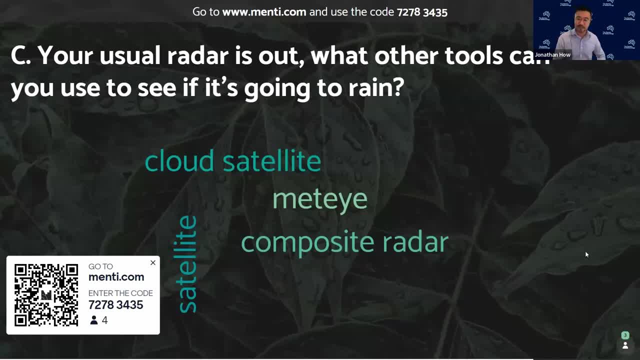 is an overlap between radar coverage, So sometimes it can kind of capture that, But of course sometimes it doesn't cover you. So yeah, looking at MetEye, which I will show in a moment, and satellite can also give you an example, can give you clues of if it's going to be. 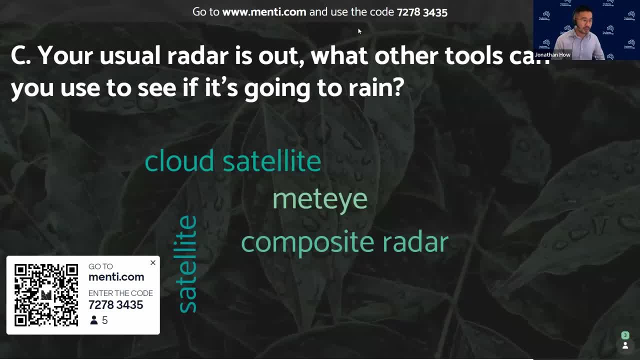 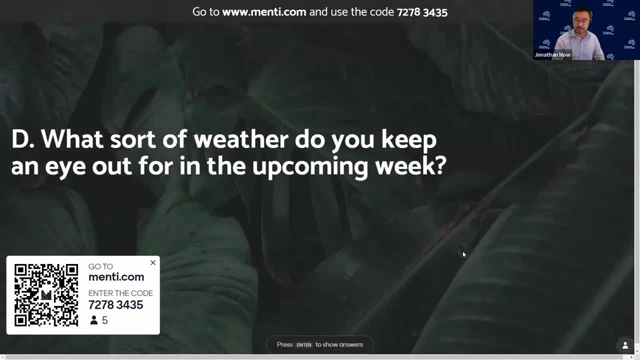 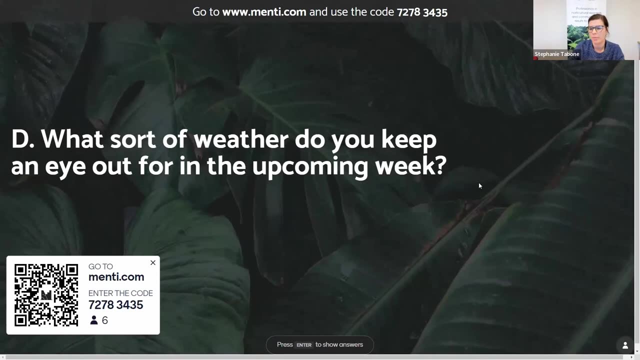 raining in your place, So we can go to the next poll, I would say So jumping into forecasting now. So the question is: what sort of weather do you keep an eye out for in the upcoming week? Can you elaborate more on that? 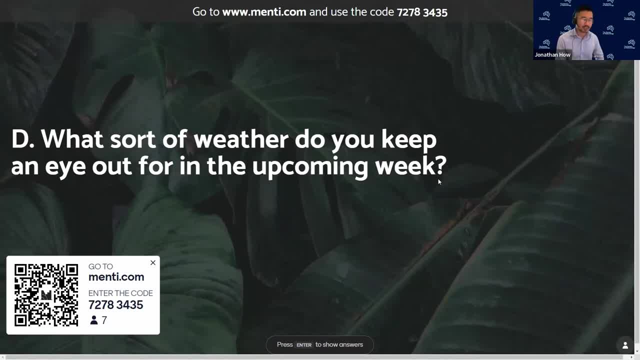 Yeah, So just to kind of, also for my kind of, to kind of tailor this. you know what's important to you. You know you're planning for the next week. Is it going to be because you know of? 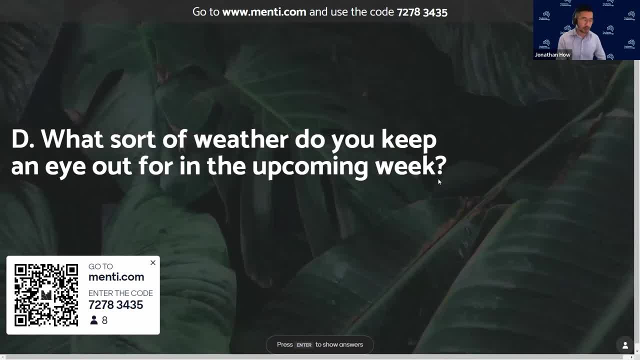 course, depending on the time of year. but you know, if you're looking at rainfall, are you going to look at temperature? Is it more important to you, you know, to look at the wind, for example? just kind of you know, what sort of things would you want to be keeping an ear out for? 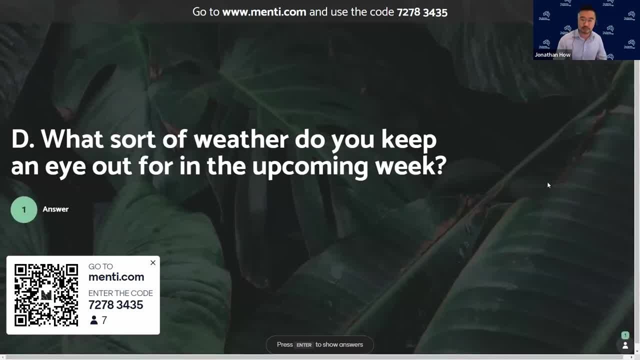 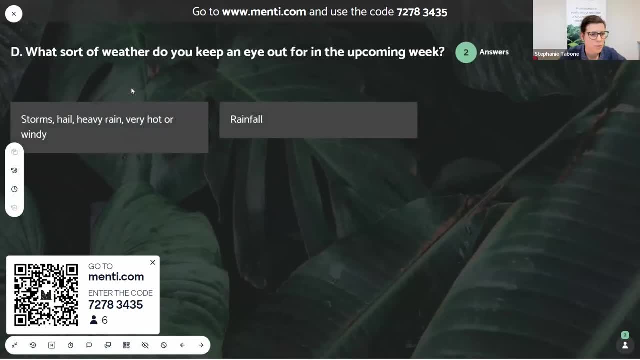 over the next week? And then, what does the forecast for feast the day require of you for the future? So we've got storms, hail, heavy rain, very hot or windy weather. rainfall from a couple of respondents: Yeah, so I think from my experience, most people want to know if rainfall is coming up. Everything. 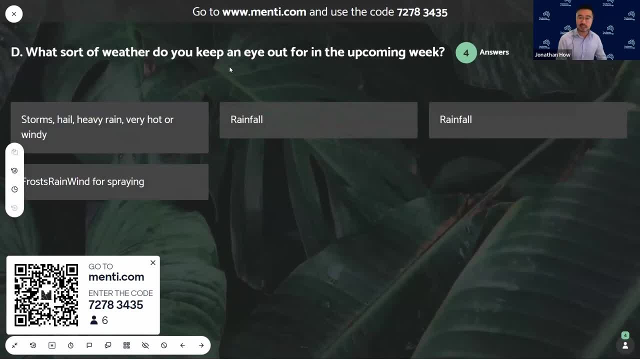 from you know, do I want to water my garden? Do I want to wash my car? You know, is there going and another flood, for example. And also you know for those living across South-East Queensland, North new south wales, you know, come september, october, november, are there going to be big storms coming. 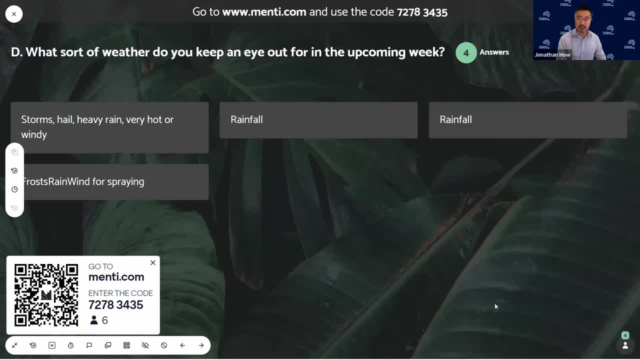 up at my place, is there going to be large hail. so these are all really important things. and also people mentioning that frost, wind, rain for spraying, you know, is there going to be um inversion, that sort of thing? so, yeah, all certainly things that, um, yeah, will be what i'm on the look. 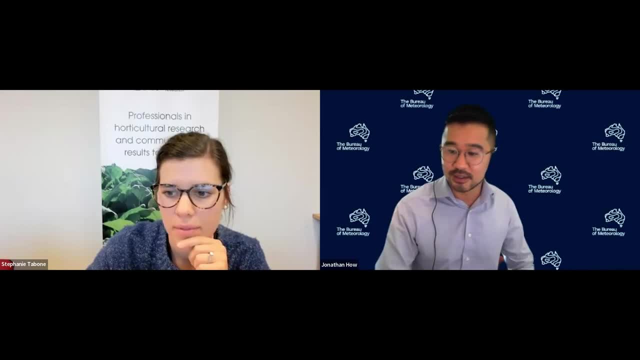 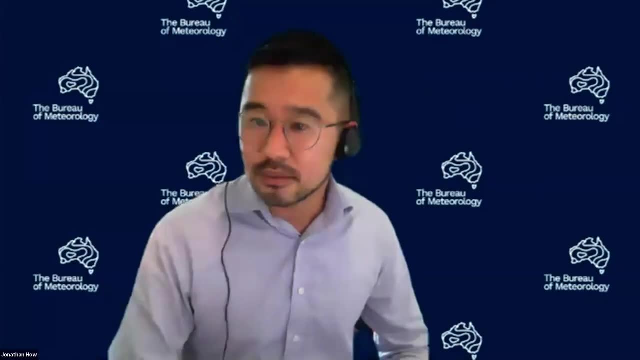 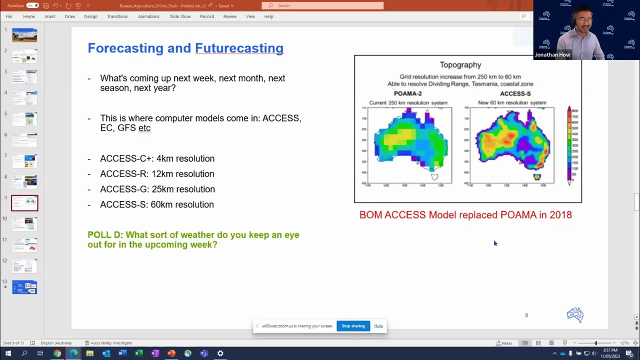 out for, so i can um jump back and share. so now we're getting into forecasting and future casting. so this is all about what's coming up in the next week, what's coming up in the next month, next season, even next year, and from a forecaster's point of view. this is where the computer models 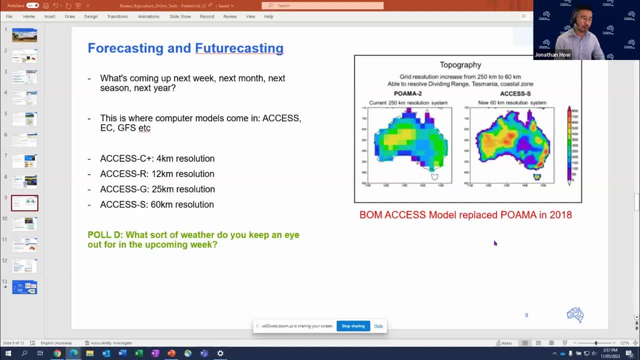 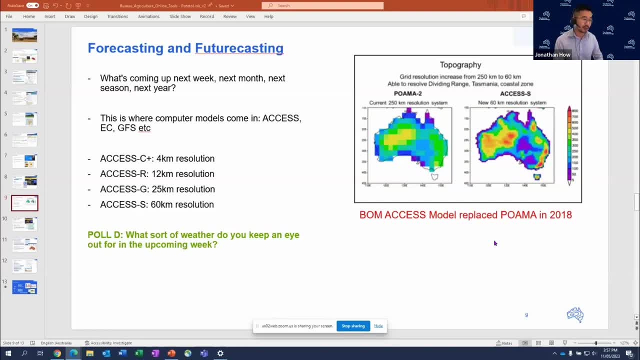 have their own weather and climate models. so in europe, have the ec, in the us and have the gfs. japan has one, canada has their own and, um, i guess the importance of the australian model is that it's developed by australians for australians. so these, these are run by, these are developed by. 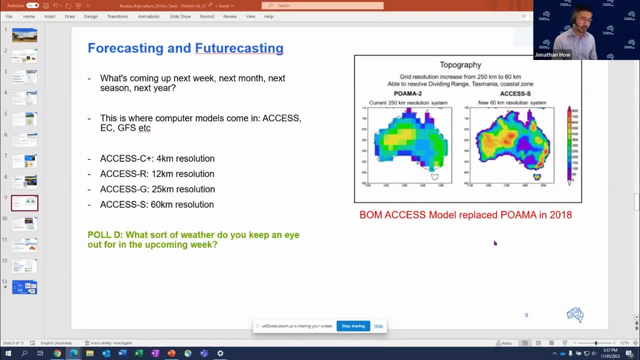 bureau scientists and the conditions are tailored and tuned to australian conditions. so you know that you're getting um a model that's kind of tuned for what australia needs. but of course models improve over time and they're constantly getting better. so the bomb access model replaced. 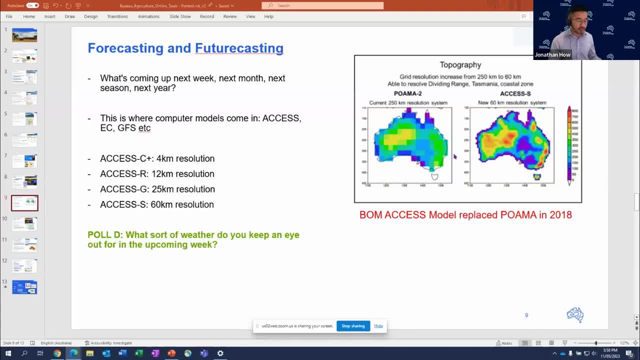 polama back in 2018. you can see on the image here that what it did was increase the resolution. so polama was 250 kilometer grid and access s is now 60 kilometer grid and we are out up to excess. access s2, the second iteration, and there are already plans to introduce access s3 within access there. 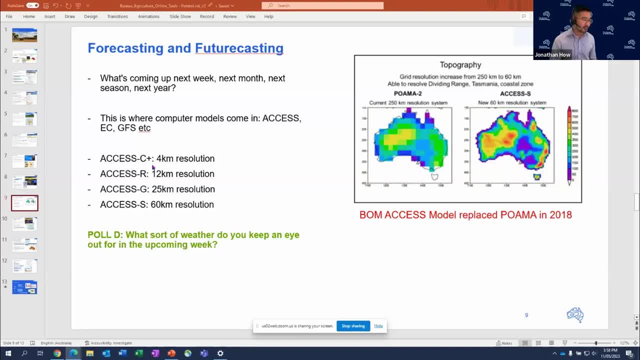 are a number of different sub models, as you can see on the left hand side, ranging from access c plus. so this is the four kilometer resolution. this is the model that can pick up anything from individual showers to thunderstorms at that um kind of small scale, all the way up to access r. 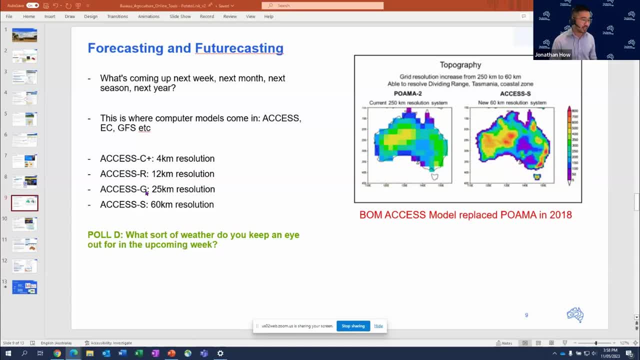 which is access regional- 12 kilometer resolution. access g is 25 kilometer resolution and access s, the seasonal model, is 26 kilometer resolution. so what the forecasters do is they take all these different models- access, european, us model- and we use a blend of all these models to produce the 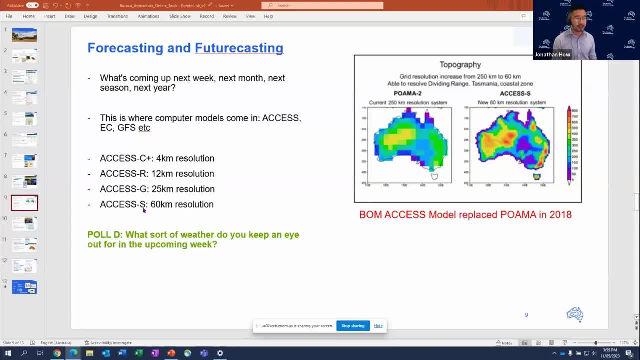 ultimate four kilometer resolution, and we use a blend of all these models to produce the ultimate four kilometer resolution and we use a blend of all these models to produce the ultimate forecast. so we take the raw model data which is being calculated by the supercomputer. 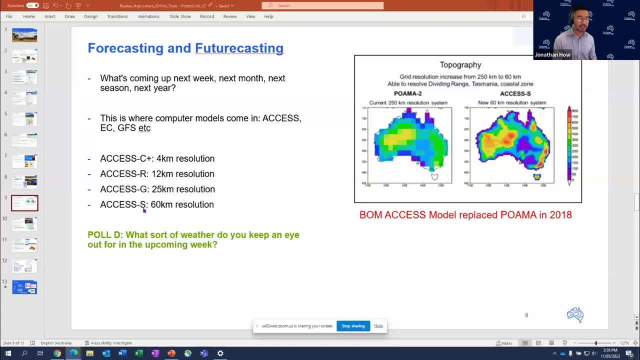 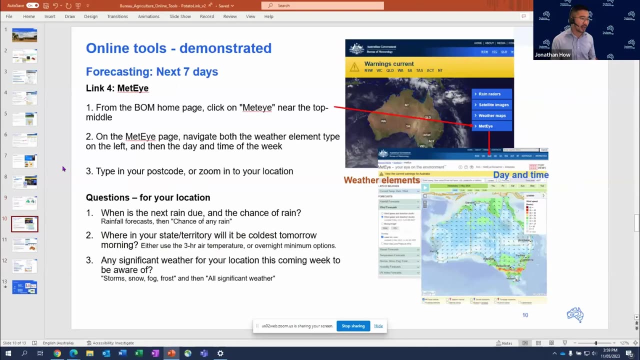 and put that into our software and add kind of that human touch, blending the model and also adding local effects that the model can't quite capture on these large scale resolutions. so on the next slide, starting off first in forecasting. so this is looking at everything in the next seven. 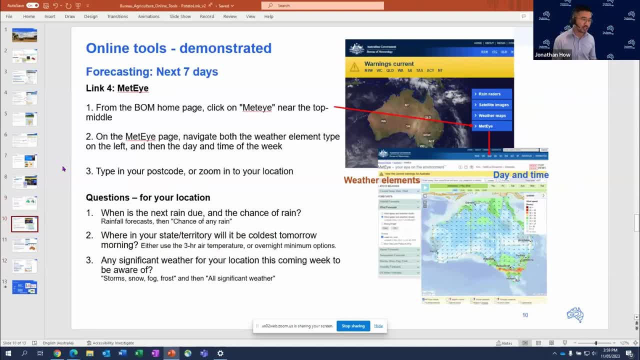 days, and it's quite a few. people have already kind of mentioned medai is a really great tool. so medai is will actually give you what the forecast has produced. so, um, we're talking about that raw data and put it into the software that we have here at the bureau and outputting that um temperature. 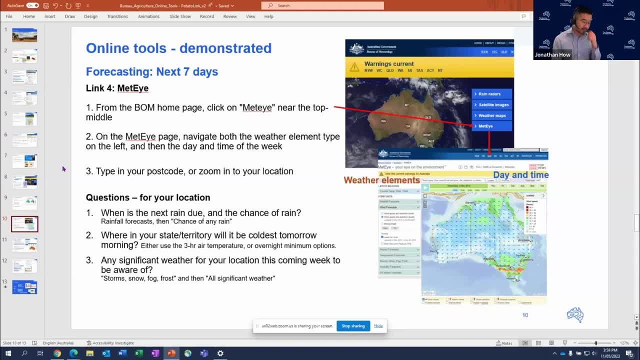 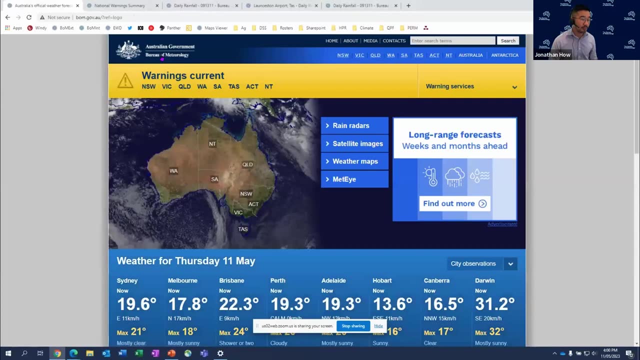 wind, rain data. you're getting that um kind of direct information on mess high. that's exactly what the forecasters here at the bureau are putting out. so, uh, the way to get to mess high. i'll just share my screen. go back to the screen here. so we want to go back to the um, back to the 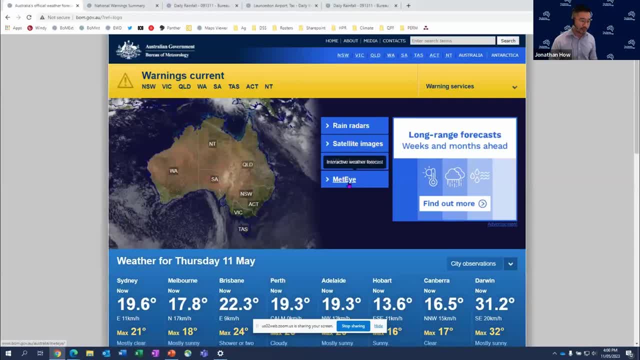 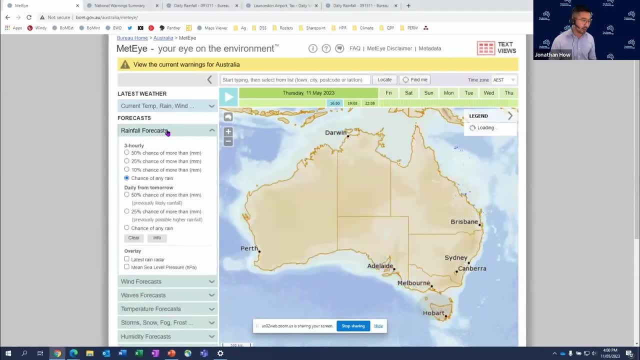 bureau page. it's under meta here, under weather maps. clicking on that will take you to a map of australia. the default is wind, but you can change it to any other weather element that you like. there's two ways to look at what you'd like for your location. you can either zoom in. 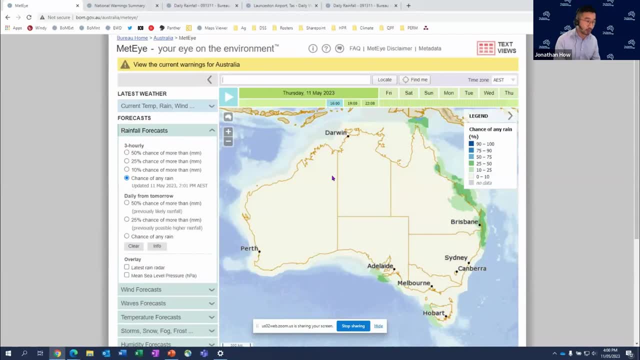 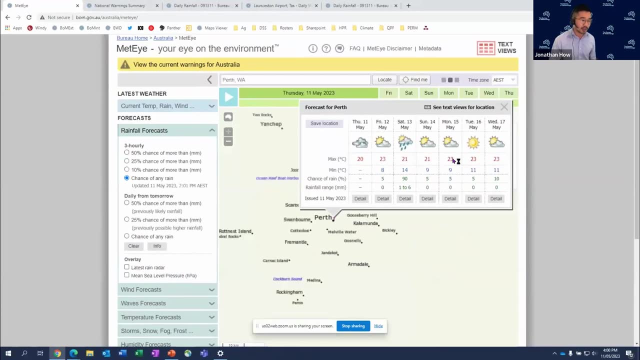 or just type in your postcode. so let's just type in for perth, for example, it'll zoom in, give you the weather forecast for the next seven days. then you actually have the choice as well to explore what's what's coming up for your location. so having a look here at some of 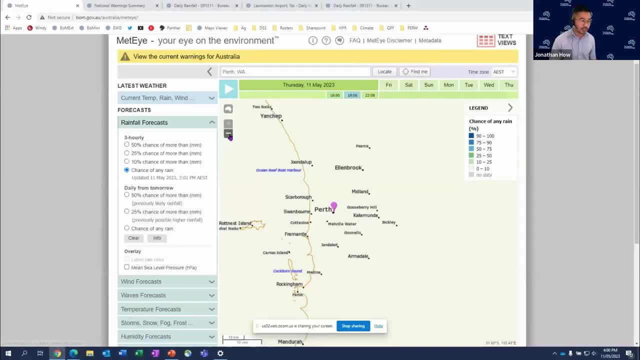 the questions. so questions based on link number four. uh, the question is: oops, zoom back here. when is the next chance? when is the next rain due? when is the next chance of rain? so to do that, uh, click on rainfall forecasts and that will take you to a couple of different. 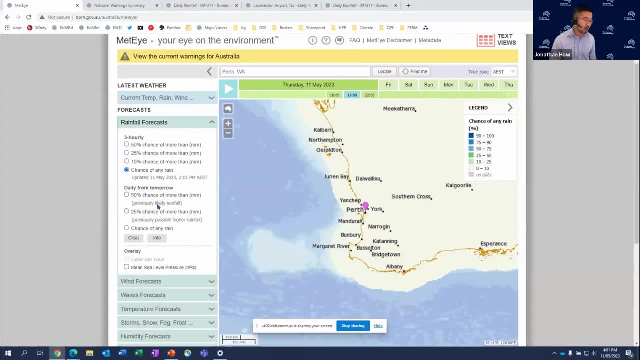 options, so you can. you can filter through by the three hourly data, or you can just want to see, if you want to see how if it's going to reflect on the forecast, and then you can filter through by the three hourly data, or you just want to see, if you want to see how, if it's going to reflect on the. 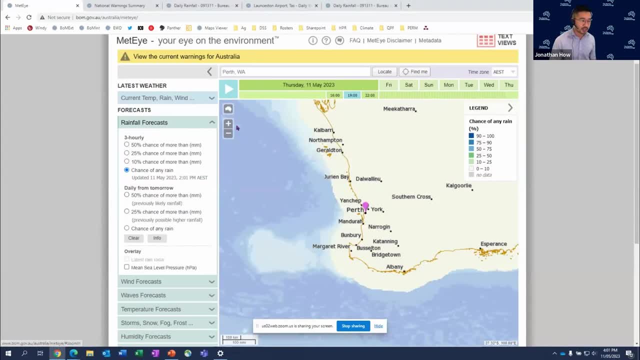 rain tomorrow or not. so what we can do here is just kind of scroll through and look through the next chance of any rainfall. at the top there's a three hourly time period, so just kind of stepping through, clicking through, you can see, tomorrow there is a bit of shower activity, coming first to margaret river and the capes and stepping. 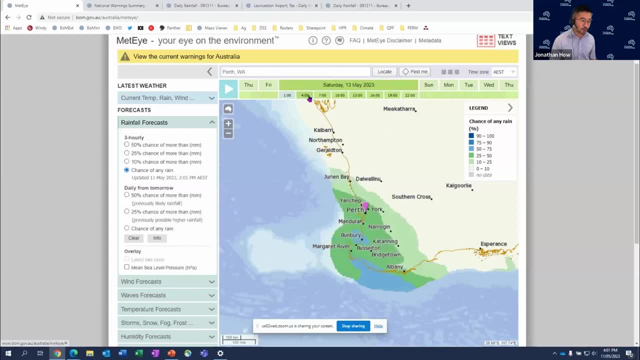 through. it's a great view to kind of see when the chance of rainfall is coming through. so what this map is actually telling you is um, based on all the different models that we have and all the different individual model runs that we have as well. so for the access model, we'll 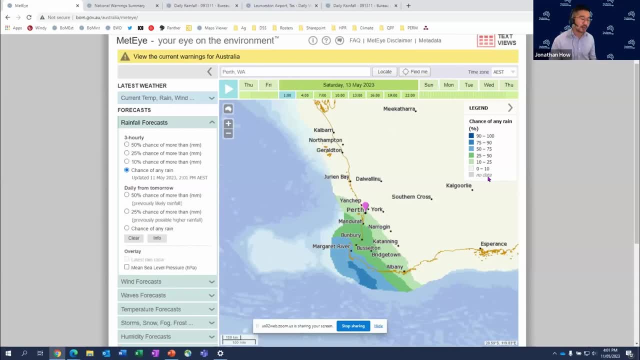 run it many different times through the day to reduce many different outputs. what percentage of models are saying there's going to be a chance of rainfall in that three hour period? so looking at saturday in the three hours to 1am, look, it's looking like 10 of the models are saying saying 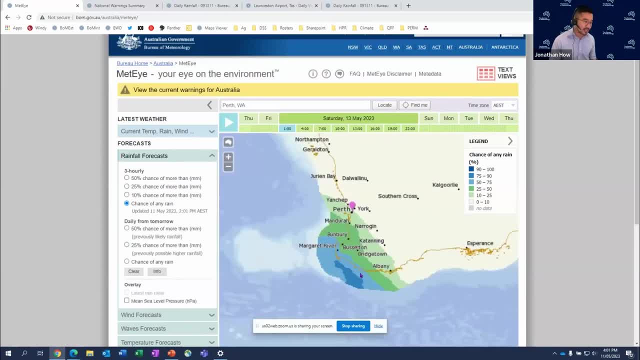 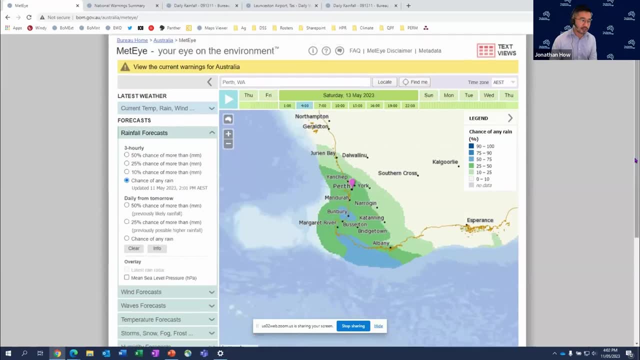 there's going to be showers across perth, but it's looking like more than 75 of the models. and it's going to be showers across the far south person, but it's going to be showers across the far south person, wa and stepping through you can see the chance of rainfall does change depending on how different. 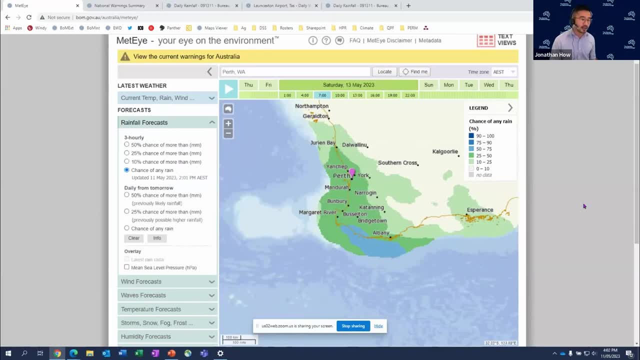 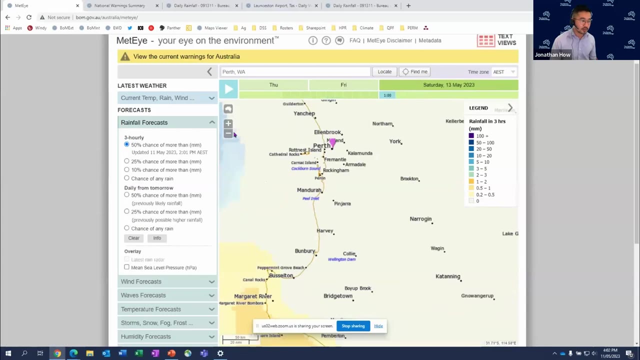 weather systems move through. so it's a really great tool to kind of see: you know what time of day are you expecting the rainfall, what was the highest chance, and also having a look at how much rainfall we can just kind of have a look through here. so if we go back into uh, saturday, saturday- 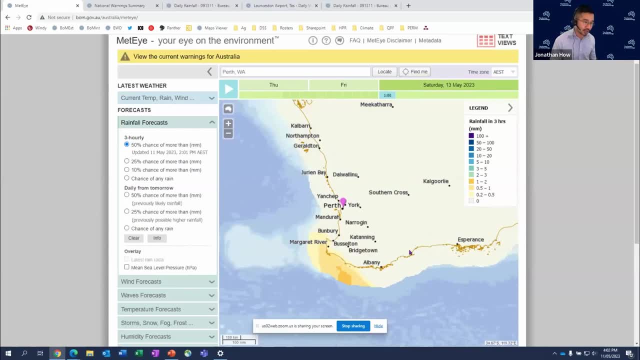 so, um the chance of rainfall um millimeters only goes out through three days. what it's showing is um. what it's basically saying is that 50 of the models are saying that in the three hours we'll get this much rainfall. so, um once you have that in the back of. 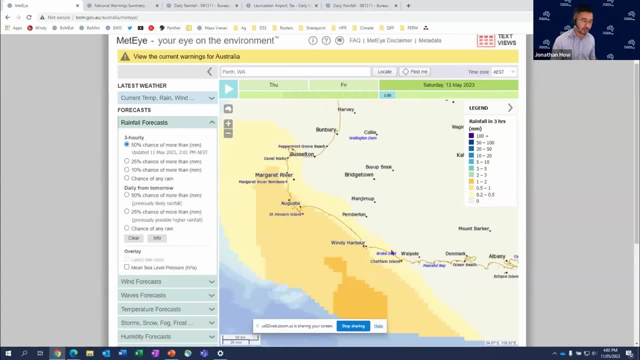 your mind. it's probably easier to kind of um kind of you know, interpret. but what the models say, in this case here, if you're down in augusta in three hours to 1am, saturday, 50 of the models are saying that we're going to be getting at least a millimeter or so. but if you want to change that, 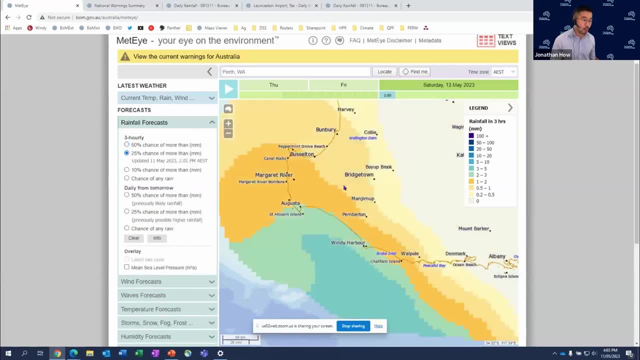 percentage chance you go, you're going to be seeing um more rainfall. so saying that 25 of the models are showing two millimeters and then 10 of the models are showing five millimeters, so it gives you a bit of a range of kind of the worst case scenario, um, you know, of course, during the wet season you'd see, you know. 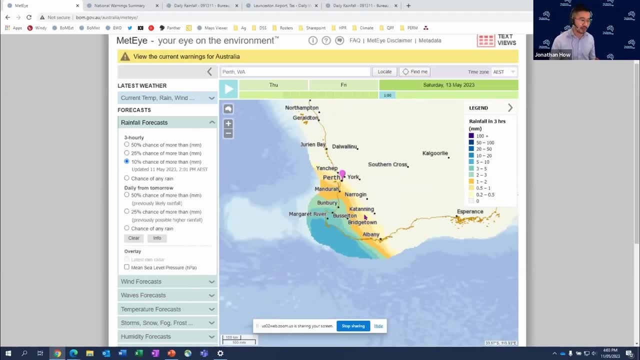 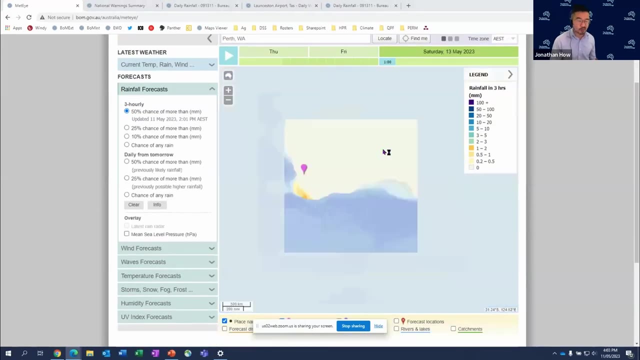 these purples, 100 millimeters, the 10 chance of 100 millimeters or more coming in that time period. so this can be a really great tool to kind of use, um to see this rainfall coming up in your location. so, um, the next kind of question is where we're in your state of territory. will it be coldest tomorrow morning? 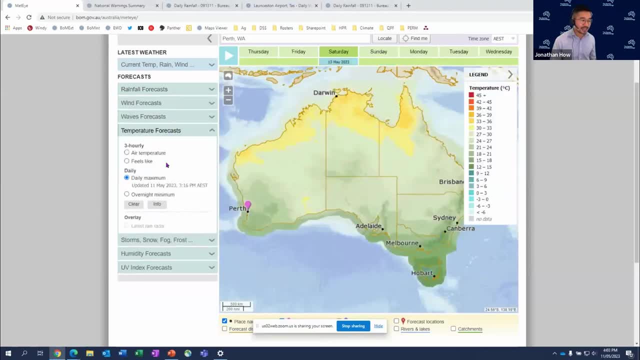 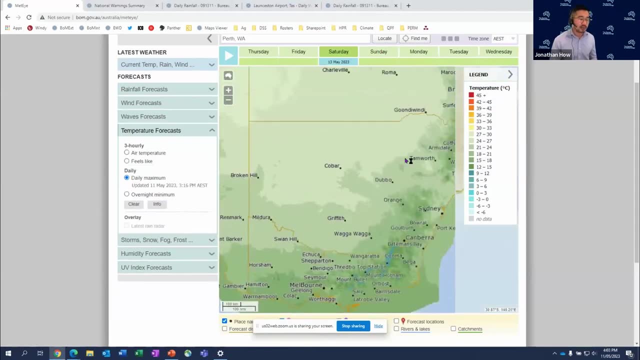 so for this we can either use um, if you go to temperature, the air temperature, or we can look at daily or overnight minimum. so let's just say, for example, we're in new south wales, you know, we just want to know on sunday morning where's the coldest location going to be. 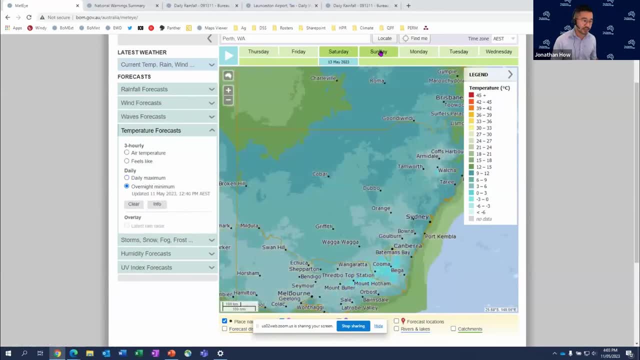 so we'll click through on overnight minimum and click through on sunday. that'll just give you that color range of where we'll see the temperature. so in the northwest of the state looking like this overnight minimum. um, you know, just clicking on there, looking to the overnight minimum of about. 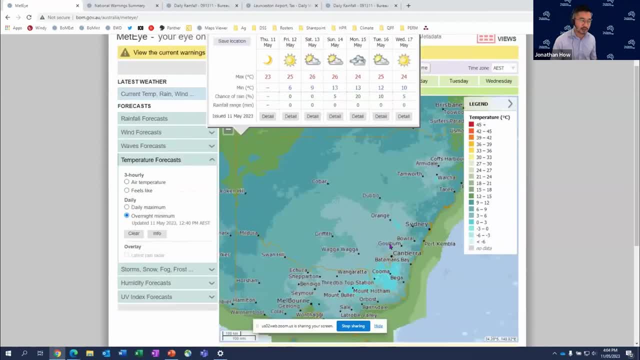 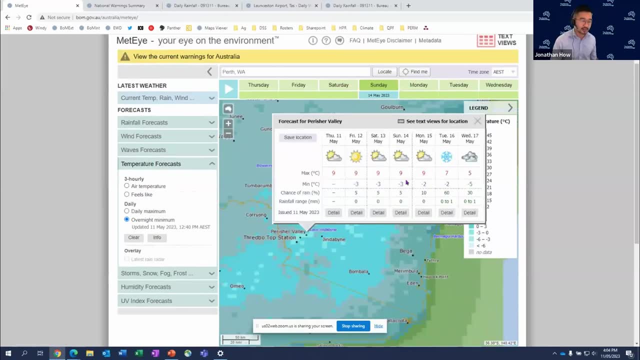 13 degrees. it looks like the cold spot in new south wales on the weekends across the snowy mountains, so it's looking like something like parisia, for example. it's going down to minus three. so maybe i can give you the the ability to act to answer quite a few different questions, you know. 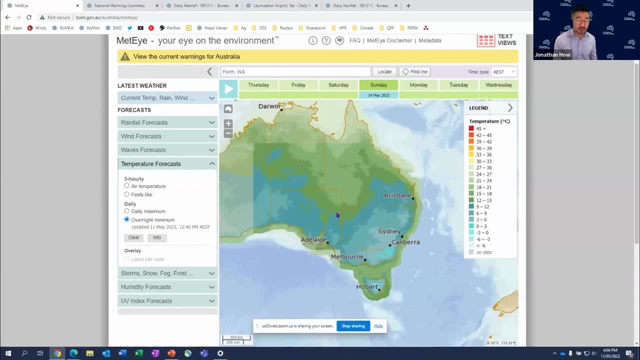 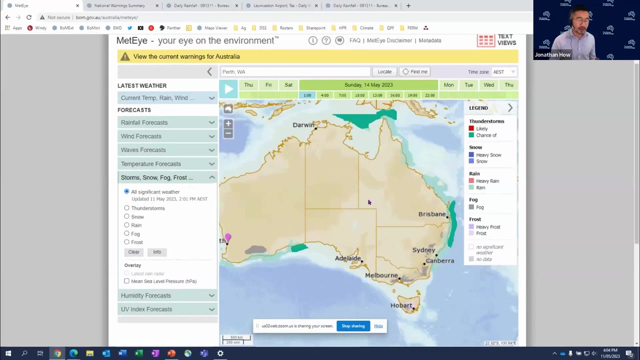 what's the highest temperature in the country tomorrow? who's getting the most rainfall tomorrow? another great one is um significant range of rain weather. So if we go down to the next option- storms, snow, fog and frost- what we have here is the significant weather what's coming up, So you can see what significant weather is there's. 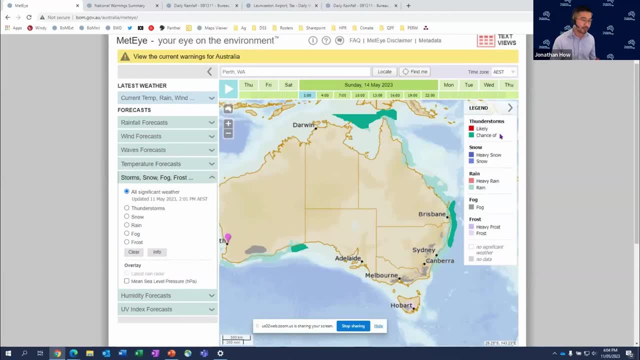 thunderstorms, whether there's a likely chance- that is, more than kind of 50% chance of thunderstorms, or just a lower than 50% chance, whether there'll be snow, whether there'll be rain or even fog as well. So you can see, for tomorrow morning the forecast is predicting. 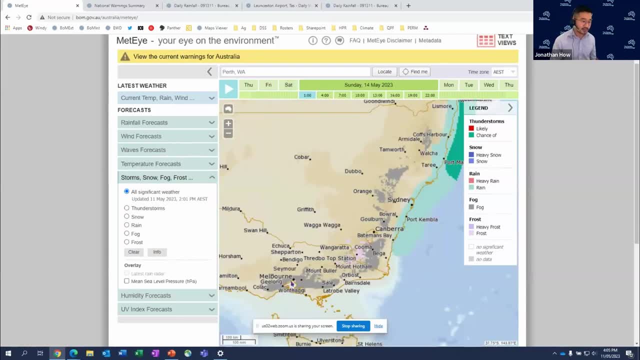 a chance of fog. sorry for Sunday morning, so I should say forecast predicting a chance of fog for these areas in grey across southern Victoria, And also you can see here the chance of frost as well. So it gives you the ability to step through every three hour time step for the next seven. 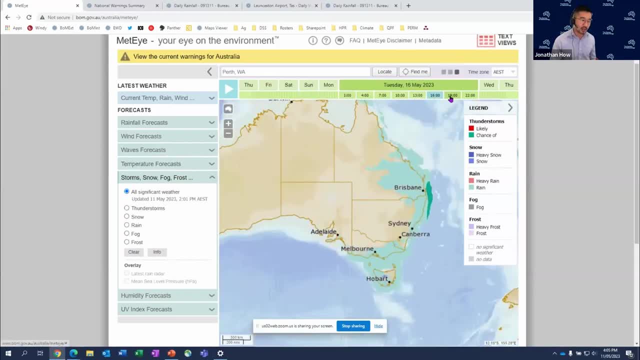 days to kind of see what kind of significant weather. So someone mentions thunderstorms as being an important thing looking out for. this is the way that you kind of have a look at it, to kind of see when in the week you can expect those thunderstorms or, you know, your frost. 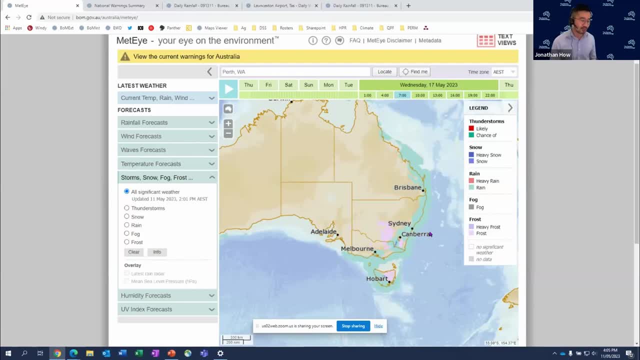 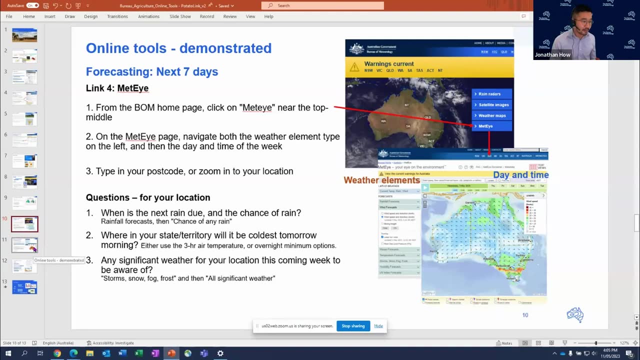 will be giving you your own versions So that might inform decisions to spray and that sort of thing. So that's a bit of an overview of the mess high Before we continue. there was one question that came in through the chat here. The question was: we have fairly detailed forecasts for seven. 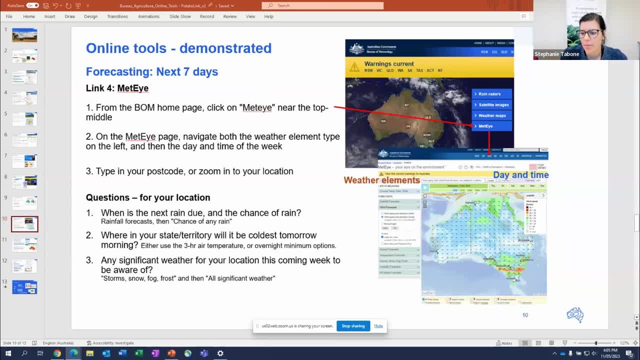 days ahead for the various parameters. Could forecast evapotranspiration be included? So evapotranspiration is not something that's going to be included in the forecast. It's not something that we currently have the ability to forecast. It's not something that the 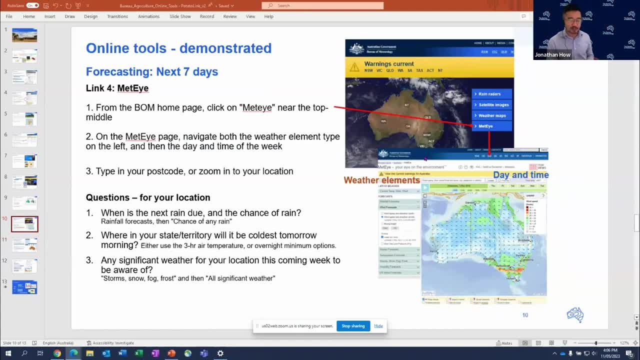 model data outputs. But certainly you know it's probably only a matter of time We do. I think there are some maps which do show average evapotranspiration over the year, which can give you an idea of historical data, you know, in terms of you know how much you expect to evaporate. 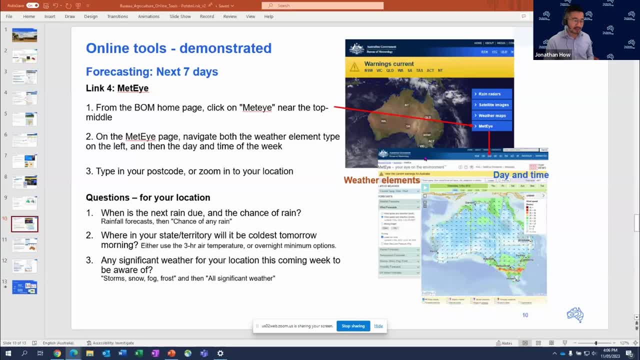 as opposed to fall as rainfall, But in terms of the next seven days, nothing that I'm aware of, unfortunately. So the best way to probably look at that would be probably a combination of humidity forecasts. So of course, you know, lower humidity and more sunshine. you do get more evapotranspiration. 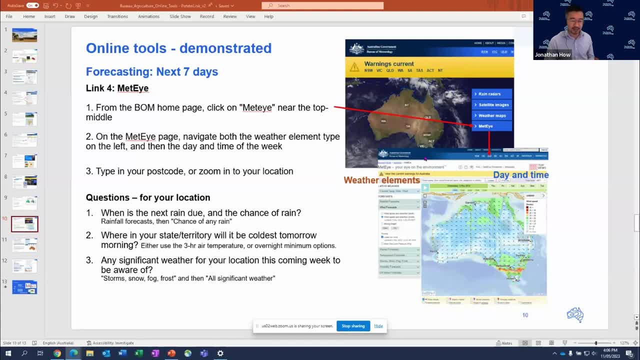 But unfortunately, in terms of direct weather element, nothing available that I know of. I'd probably just add there as well that, yeah, I'd really like to see evapotranspiration forecasted well on our publicly available website. But I have had 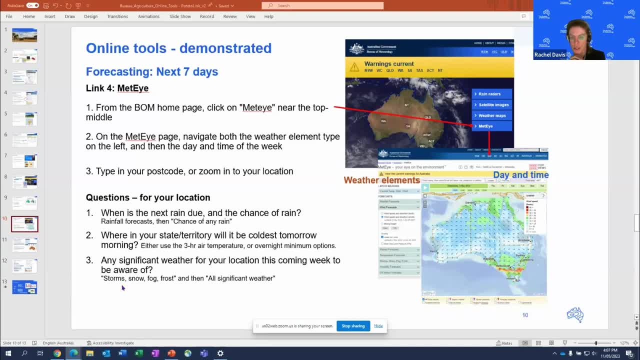 feedback that internally, that because it's a very agriculture-specific product, you know the likelihood of it to appear on, you know, a tool essentially for the public and community. it may not appear somewhere here But that doesn't, you know, necessarily suggest. 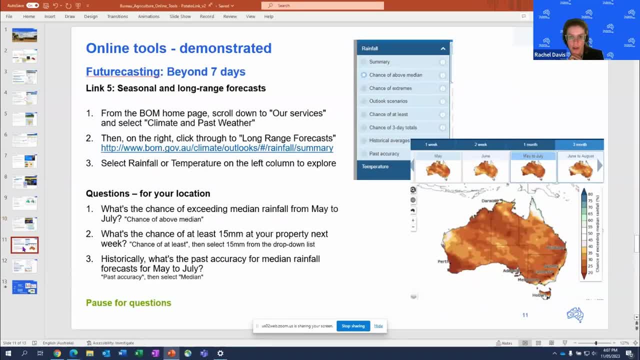 that it's not going to appear somewhere else on another more ag-specific tool or website. So yeah, definitely want to be flagging. since I started the Bureau last January- And I'll feed back Peter Smith's question as well- I keep feeding back to people how important it is for agriculture. 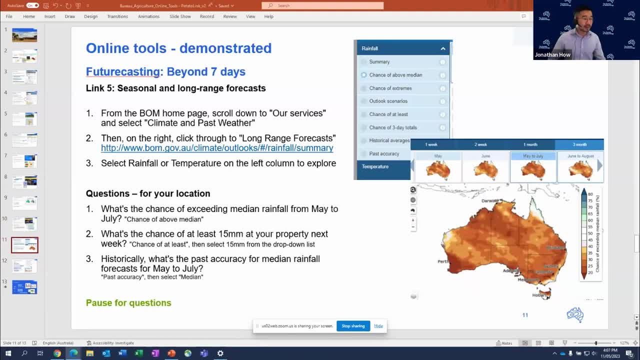 Thanks, Rach, That's really great. So yeah, finally looking at future casting, And at this point in time we're looking at kind of weekly to seasonal and even yearly forecast. So I did note that most people are kind of interested in you know what's coming up. 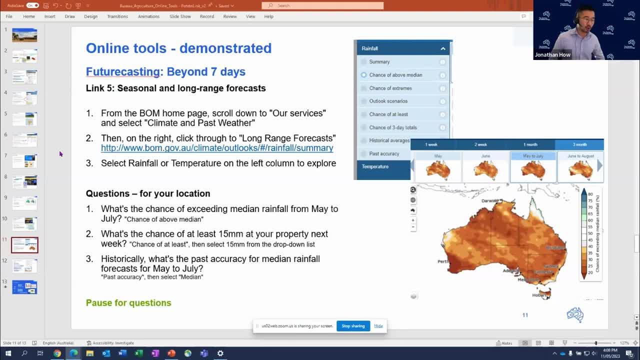 And it flows on nicely for what Rachel was speaking about before. The 4-1 is 4-1 project did produce five different maps based on the Axis S model that you did see, So I'll take you through some of these maps and how you can use them. 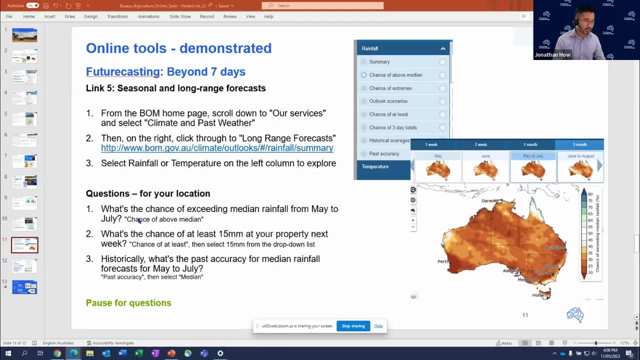 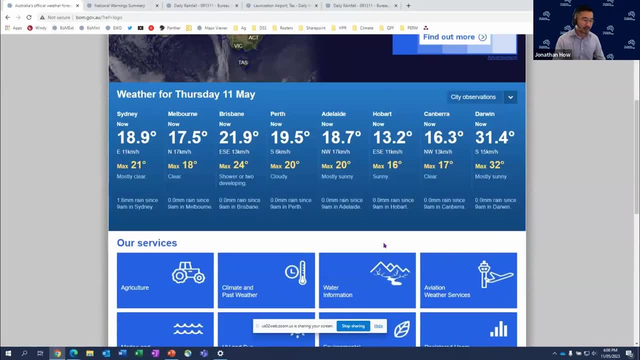 for your location before going through some of these questions. So what we'll do is, again, we'll go back to the Bureau's homepage, And this time we want to go down back to the Bureau's homepage, So we'll go up here. 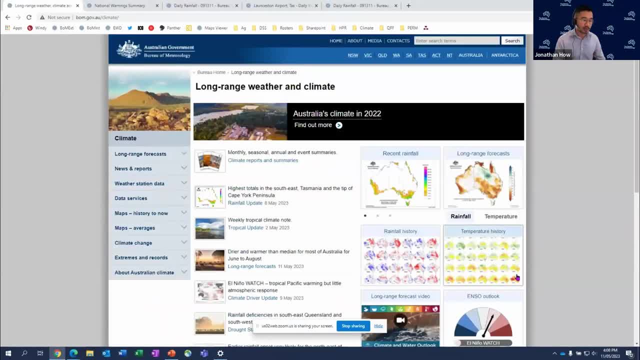 We want to go back into climate and past weather. So click on that here. This is your climate portal again. And then the right hand side: we want to go into long range forecast. So this brown and blue map everyone knows and loves. 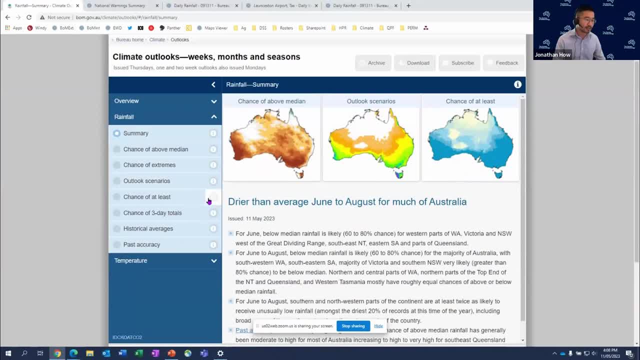 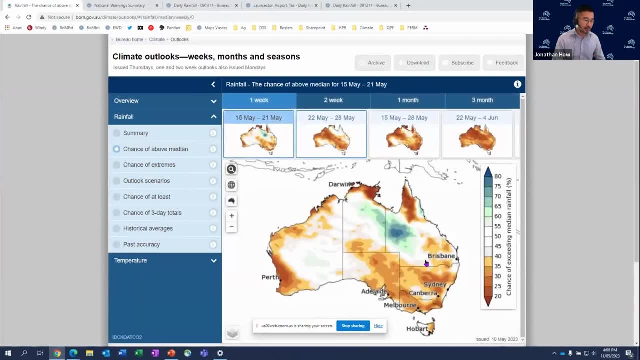 This will take you to our climate outlook page, And the most common one that people probably already know is this: chance of above median rainfall. So this is the map that shows you the chance of exceeding median rainfall on weekly, monthly or even monthly. 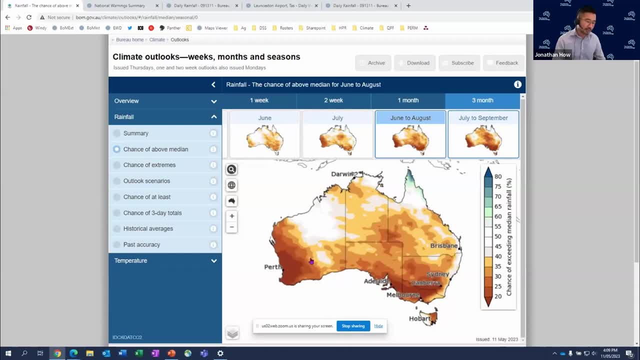 or even seasonal scales. so, as I mentioned before, Australia is going to a very dry period heading into the winter season and that's reflected in these dark brown shades. but some of the other maps that came out of this 4-1-4-1 project basically help farmers and help producers. 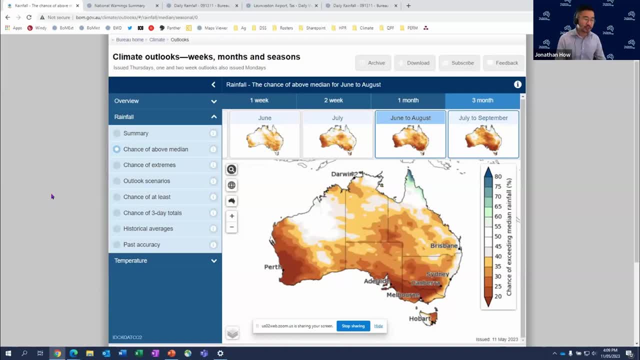 give a bit of a heads up any extreme weather coming up. so Australia is extremely prone to extreme weather and of course the last couple of years have really shown that. but there really hasn't been any sort of maps or tools to help guide decisions amidst kind of changing climate. 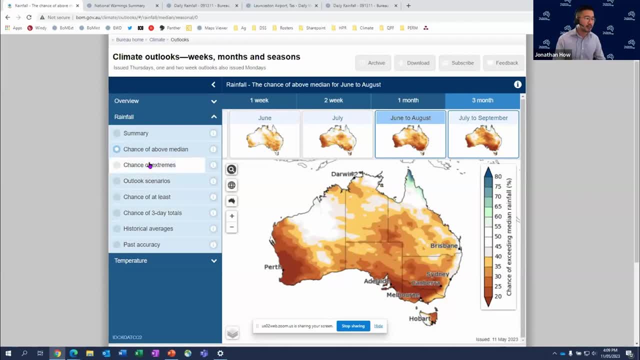 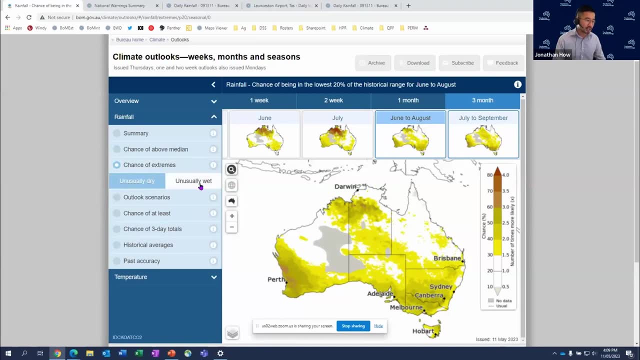 climate change and these extreme conditions coming up. so the the first set of maps that were introduced are these chance of extreme maps, and they're divided into chance of unusually dry and chance of unusually wet for rainfall. what you're seeing here is the chance of seeing rainfall in 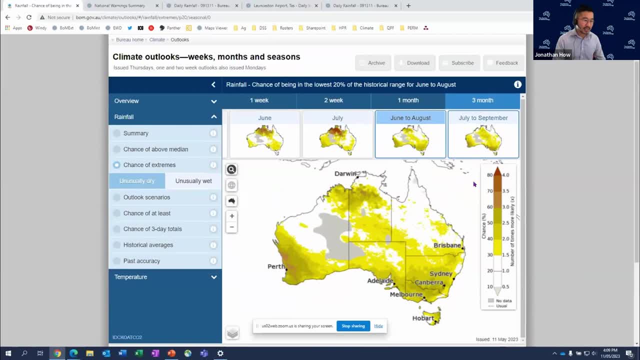 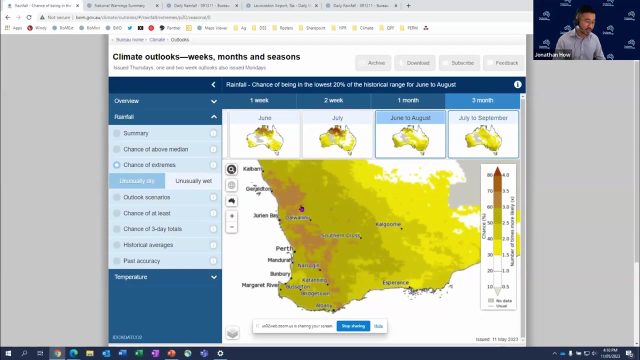 the bottom 20 percent of historical records, as you can see here, for June to August, um, it's not going to be unusually wet and that's that's no surprise there. um, and then the same thing for temperature. if we want to look at temperatures, the chance of seeing um unusually. 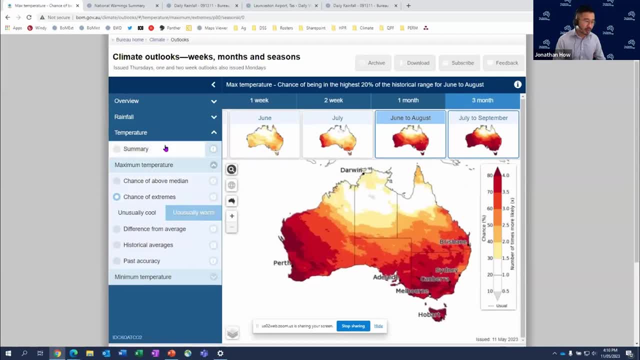 high temperatures, for example. so again, um temperature chance of extreme and chance of being unusually warm. so unusually warm is what is the chance? it's going to be maximum temperatures of the top 20 percent of historical records, as you can see here. so it's going to be um up to four times as likely to be that highest temperature quintile for. 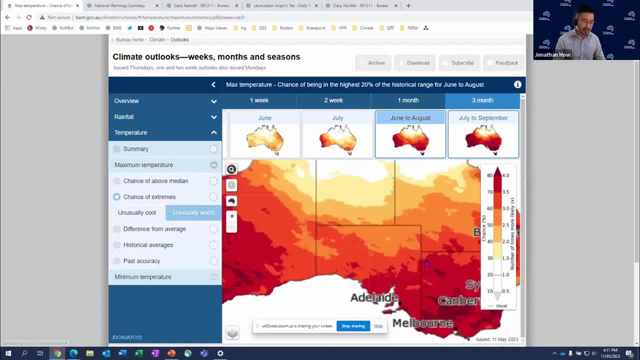 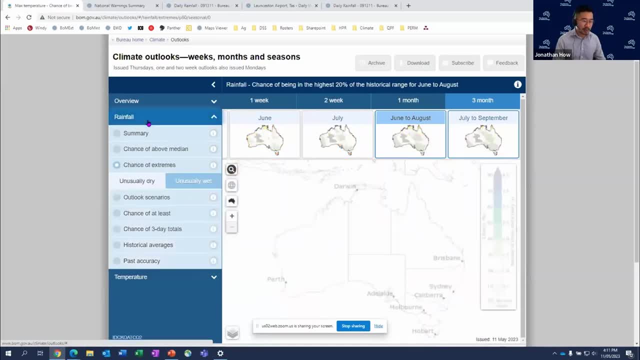 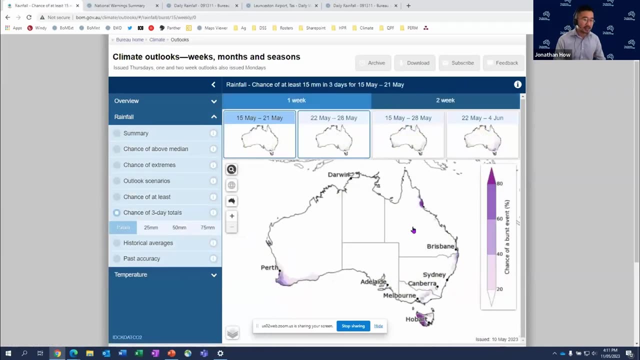 Western WA, as well as for parts you can see here of northern Victoria and into the Riverina in New South Wales. another map that came out of, for one is four arms um is these kind of burst rainfall events. so this is particularly useful, for example, for um kind of growers looking for a certain amount. 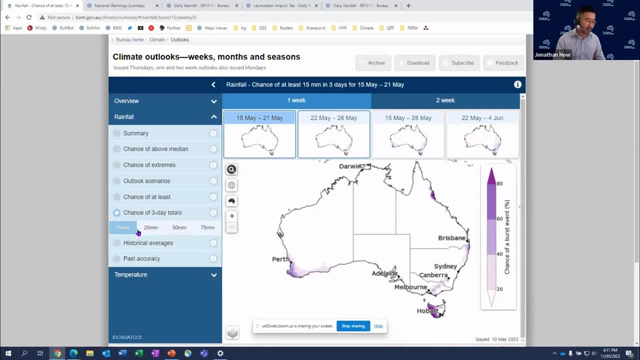 of rain in three in a three-day period, and you can filter on the left. you can um kind of choose the left-hand side, what rainfall you want to show. so, for example, um, in the coming week, I want to know what's the chance of getting 25 millimeters over three days. you know, for purposes of something like: 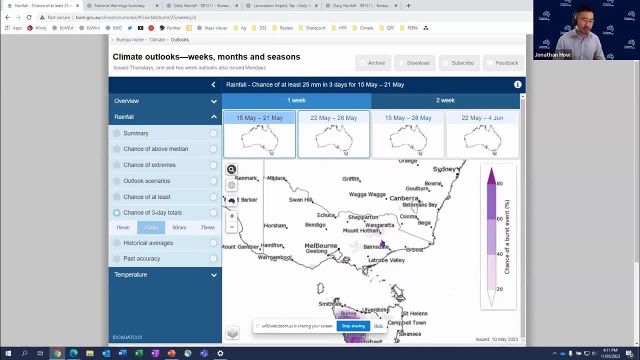 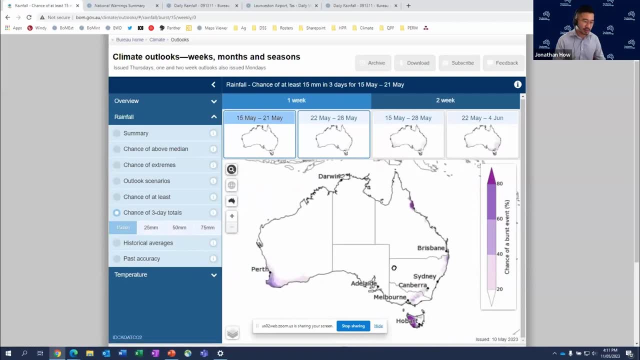 autumn break. you can just choose that and kind of see that you're fairly low chance of seeing that over the next um over the next week. but then changing that to 15 millimeters it's probably um a slightly higher chance of seeing that 15 millimeters over three days. and there are quite a lot of other maps as well. you can. 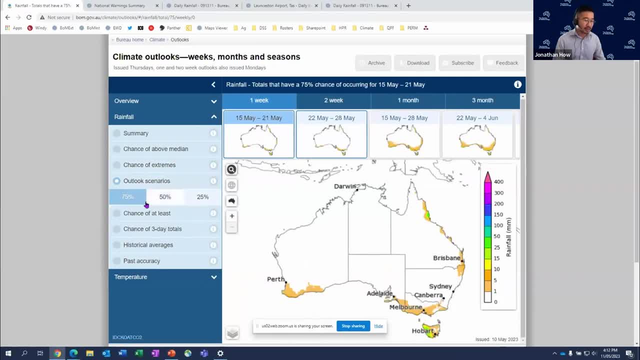 have a look at the outlook scenarios. so again looking at what percentage of the models are saying there's going to be a certain amount of rainfall, and then you can also filter that by the rainfall amount we look at as well as historical averages for that location and 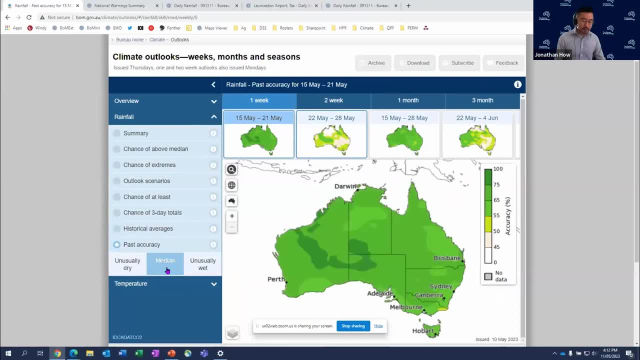 past. accuracy is a really important one as well. so at the moment, we're coming out of this autumn predictability barrier, so typically across the autumn season the models don't do so well just because we're in that transition period, and so it's it's really important when using these maps to have having the back of 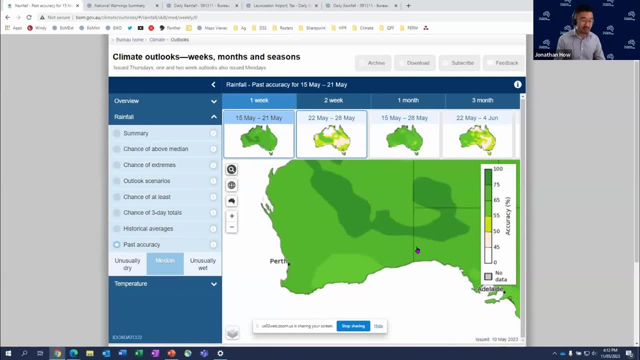 your mind. okay, the model's saying there's going to be, you know, 30 chance of exceeding average rainfall, so it's going to be fairly dry. but how accurate has the model been in the past? so you can kind of have a look through and see, for example, in for the month of June, the model gets it right. 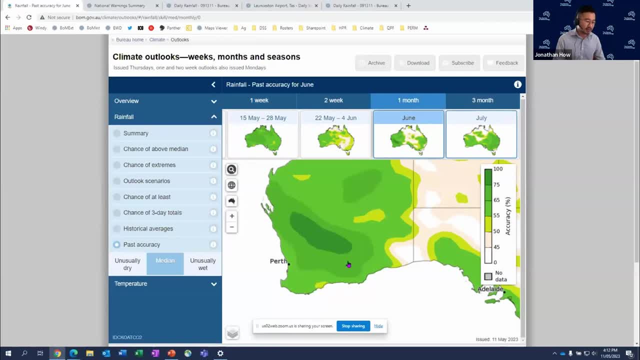 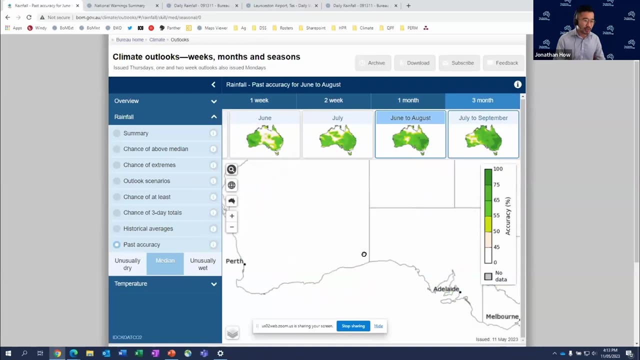 50, 55 to 65 percent of the time across Perth, but then further in Land you go to the Great Southern and central weakbelt, increased up to 75, and we do expect to see an increase in model accuracy through the winter season. so, for example, looking at June to August, this is a little bit times. we. 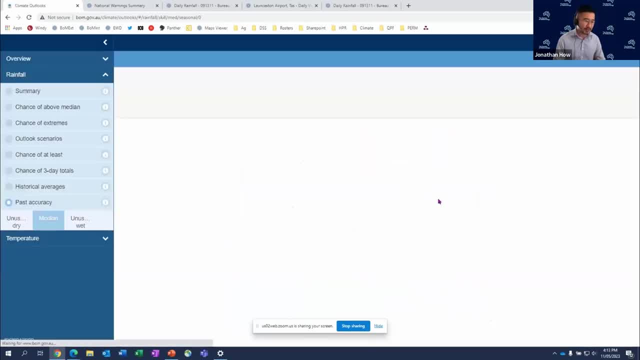 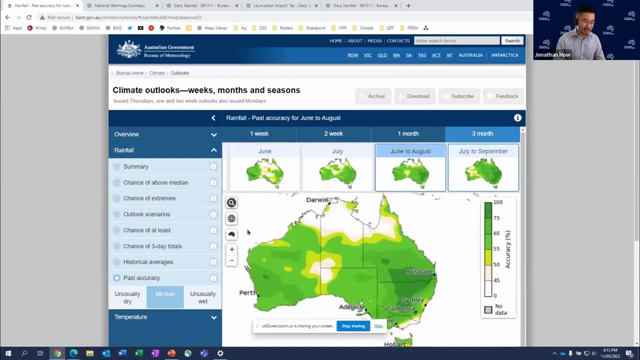 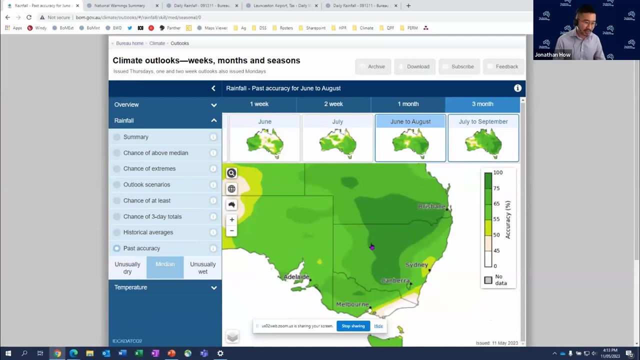 do expect to see increase in model accuracy. I'll just kind of refresh that there. we do expect to see and model accuracy through winter, as you can see here for most of eastern australia. so again, that kind of um you can have, you can, you can have a high level of confidence in what the outlooks. 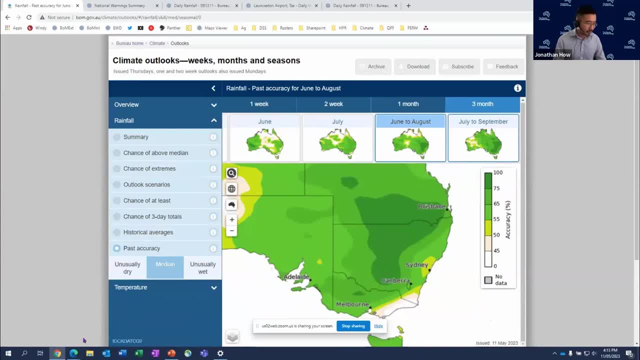 are telling you. so i will go through those um some of those questions there. so, for example, um looking at uh questions based on link number five. so let's just say, for example, i'm going to look at the lockheed valley um in southeast queensland. so question one: what is the chance of exceeding? 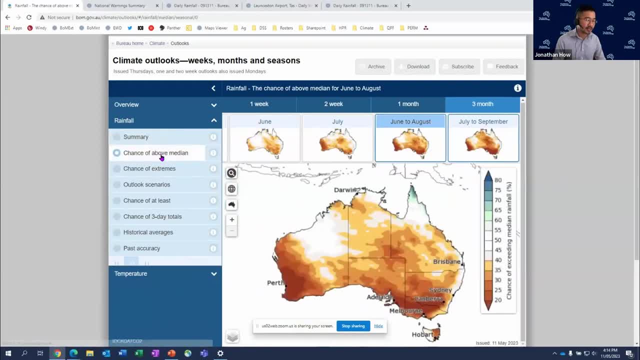 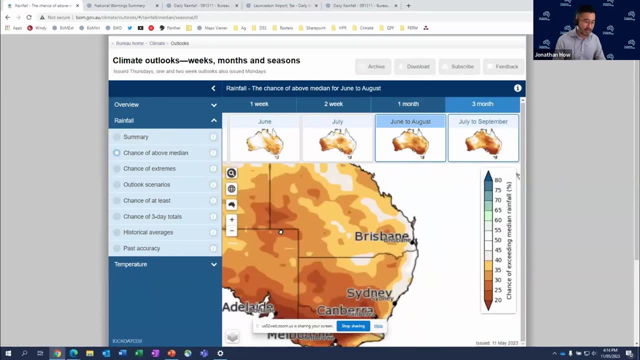 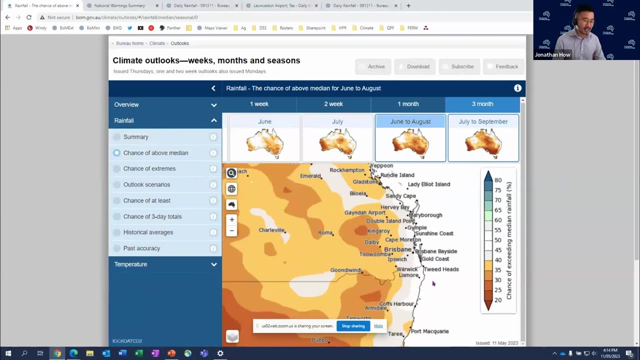 median rainfall from may to july. so what we're going to look at is: um, sorry, i will change that to june to august. we have updated the maps today. so what is the chance of exceeding median rainfall across lockheed valley? uh, through winter it's looking to be less than 40 chance. so what it's? 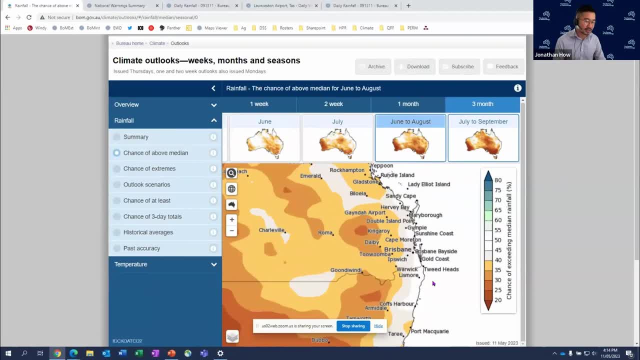 saying is that, uh, 40 percent of the models are saying that, um, it's going to be, we're going to be below, it is going to be below which rate for um 40 chance of that happening. um, if you want to look at what is it? sorry? sorry to interrupt you, jonah. i was just going to ask: um, did you just show? 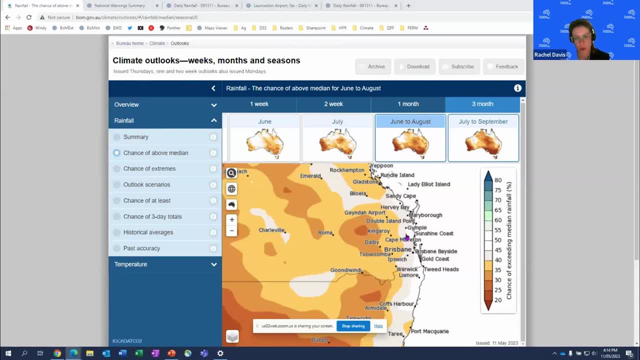 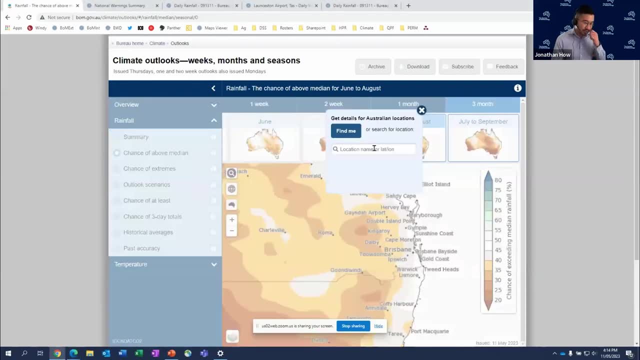 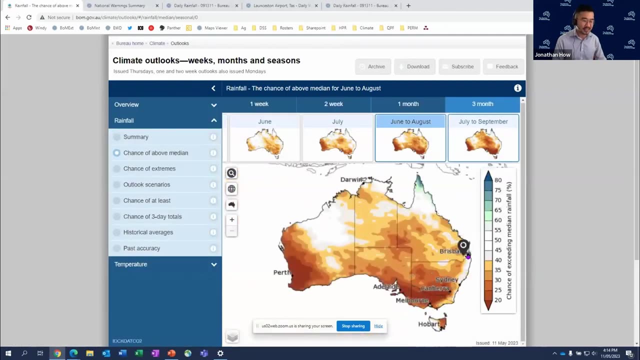 just to check the magnifying glass, or you could actually put your location in as well. yeah, just room to add that. yeah, true, so, yes, you, you can also um, just you know, for example, because you, you um, some statistics and these are some more products which came out of four one, four round. 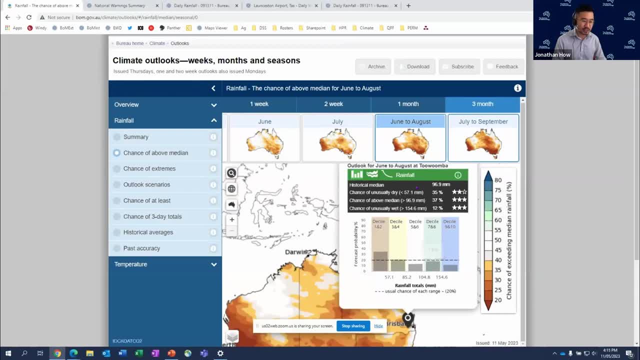 um, as retro shows. so it does take a little bit of time. so what it does is shows you a bit more detail for that location, for example swimmer, june to august, the um historical records show that the median is 97 millimeters and it shows you the chance of being unusually dry, by meaning usually. 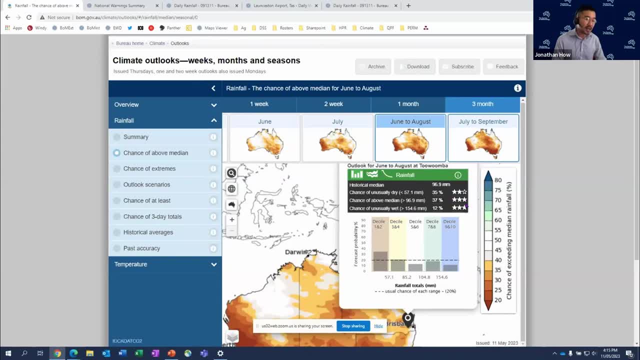 wet and these stars give you um accuracy. so three stars. so yeah, pretty good, two stars saying not so accurate, one star will be. don't rely on this too much. so this is another tool that came out of four. one is four armed to give another kind of um, a little bit more um to give growers even more. 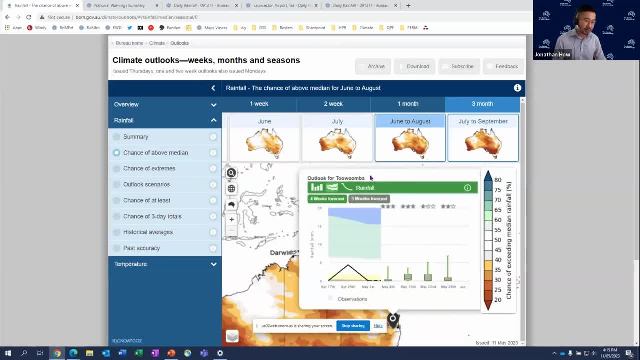 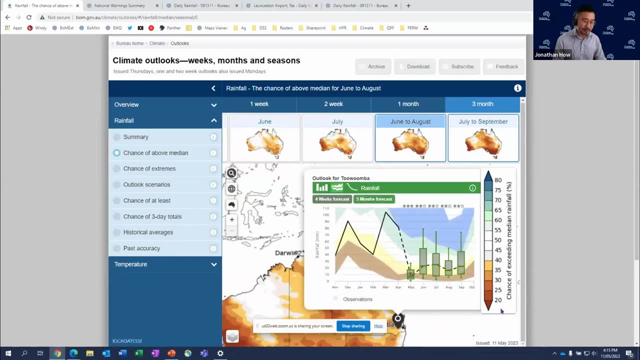 confidence in what they're looking at, the forecast. we also have these climatographs which show a similar, um, similar sort of information, but just showing, for example, um, what is? all these different colors of the different quintiles, the twenty, forty, sixty, eight hundred percent rate for ranges based. 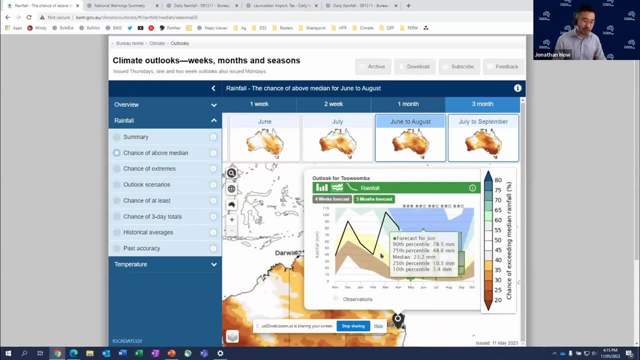 on historical data by month, and then these little plots show you um the range of rainfall expected. so definitely, if you haven't a time, have a look through and if any information, click on this little icon for information. you should have a little bit of a video and a bit of an explainer. 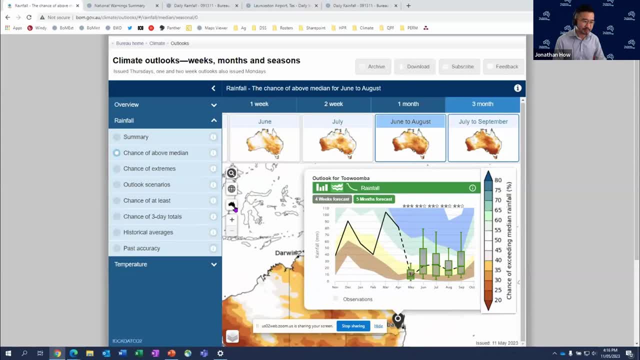 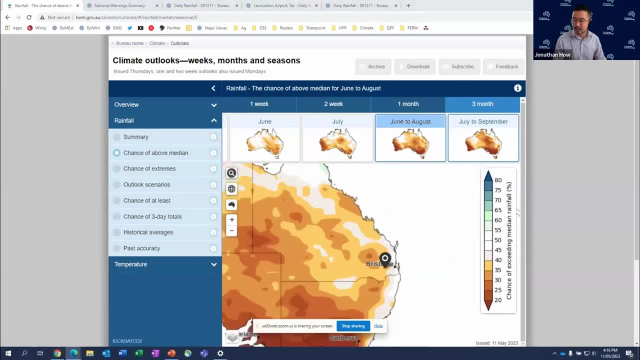 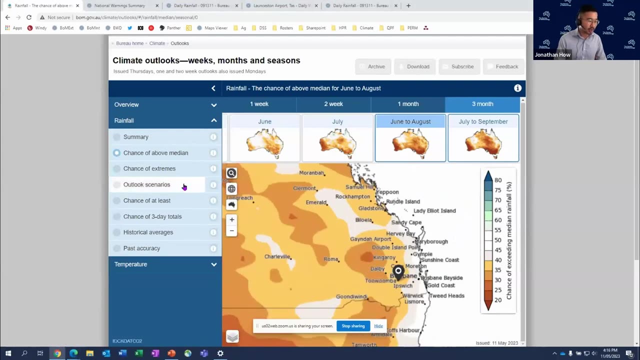 of how to actually use these products and get the most out of it for your location. but, yeah, continuing on with kind of looking at um, looking at, lock your valley. so the question here i have is: um, what, what's the chance of at least 15 millimeters over the next week? so what we can do is go to um chance of the least. 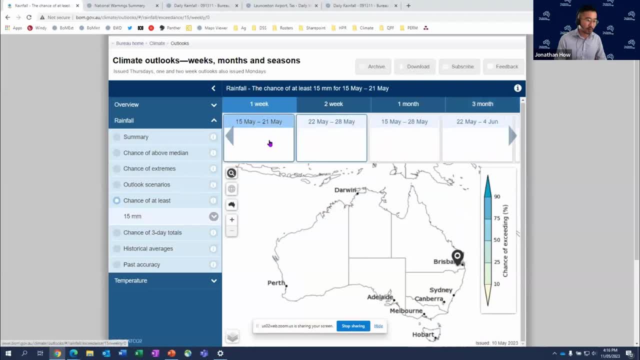 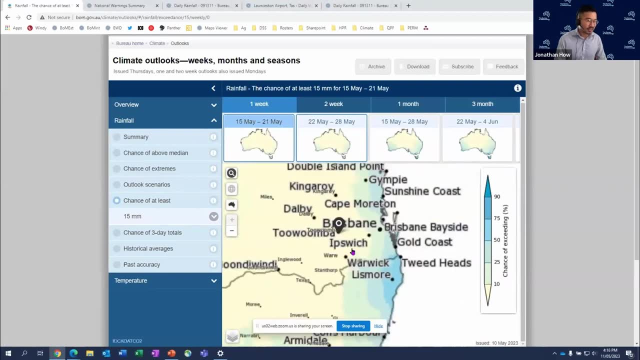 select 15 millimeters and you want to know what's coming up in one week and again we might go to zoom in again. so this is showing that lock your valley. the chance of seeing 15 millimeters next week um is looking pretty low, looking to be less than 25, 10 percent uh up to the west of brisbane and 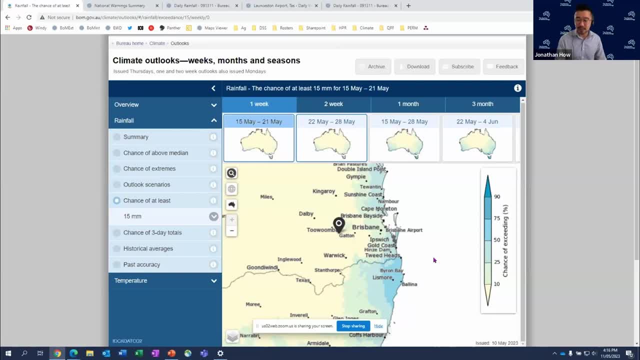 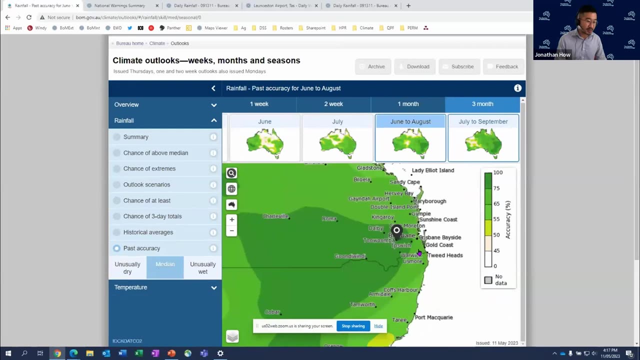 then if you want to know what's happening in the south east queensland, um, i would say, you know, okay, we've seen all that, but what's the historical accuracy, um, for kind of june to august? so again, kind of going through past accuracy and then selecting the period we can zoom in and go, okay, for southeast queensland. 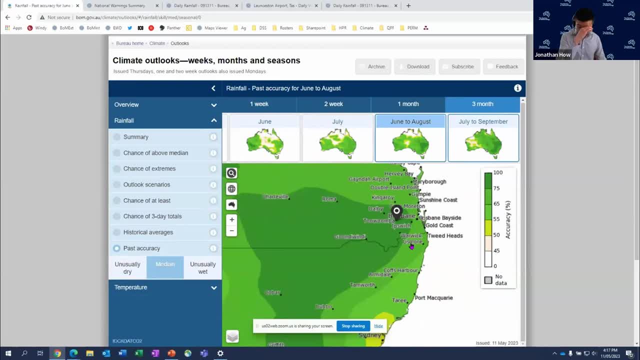 the accuracy is pretty good. you know it's looking to be more than 75 accurate um based on all historical data um. but of course there are limitations with the model itself, particularly resolution. 60 kilometers on land can have huge elevation and vegetation changes, so representing one location is a 60 by 60 kilometer grid point might not always get the job done, so it is. 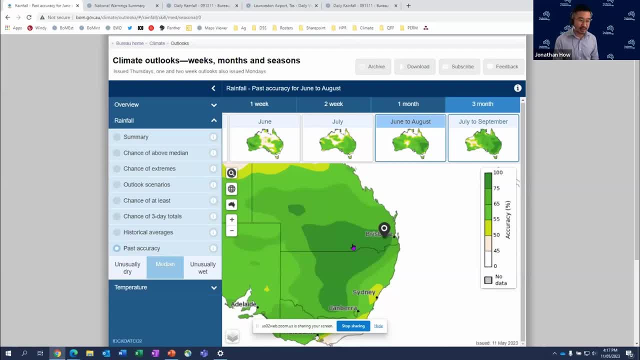 important. that resolution is a key limitation of the access as data and that can also play a part of in terms of what sort of weather events you can and can't pick. so, thinking of thunderstorm events, thunderstorms you know, typically five to ten kilometers wide, but given that they can't be, 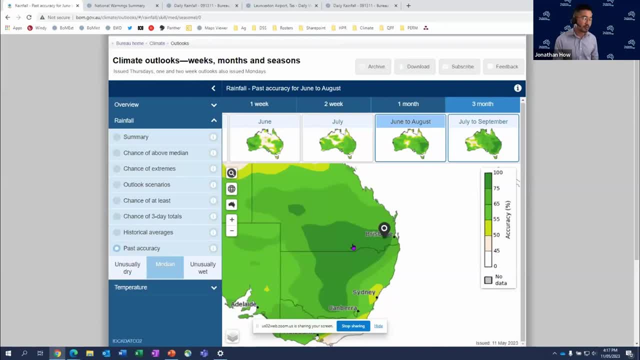 represented by 60 kilometer grid. so that's the climate models, particularly in the week ahead, can't quite pick these big thunderstorm events. so it is really important that you look at your warnings, look at your now cast and look at your net eye to get the more granular detail for your. 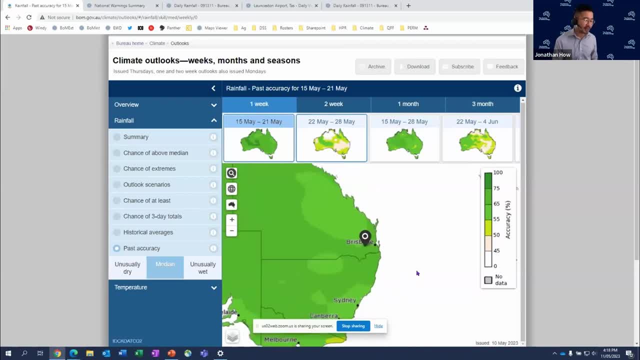 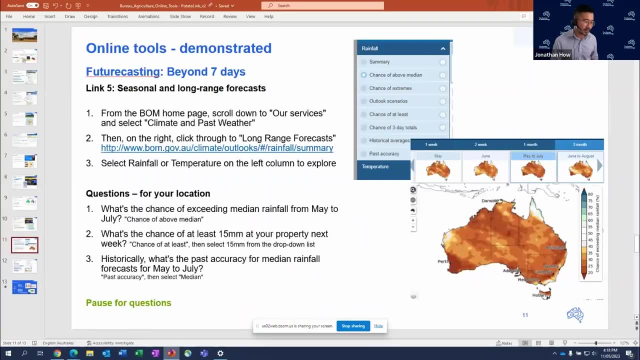 location. so definitely access s having all that in mind when you're looking at the accuracy and limitation of the models as well, but just give you a bit of an idea of what what's coming up over the next kind of months or so, so i'll pause for any questions. a lot to take. 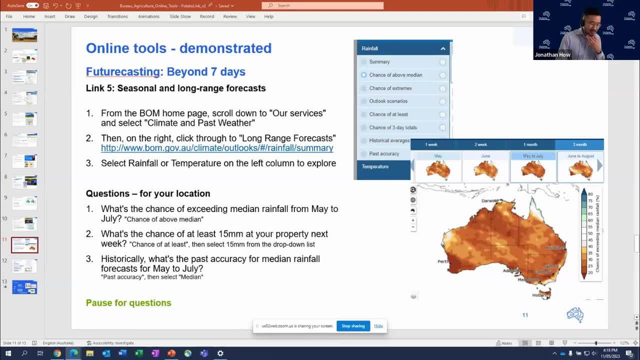 in. so certainly feel free to go back and have a look at some of those slides later on, but any questions at all? currently nothing in the chat there. jonathan, i was just wondering if, peter, you wanted to have or provide a comment on like context from a potato growers perspective, like what are 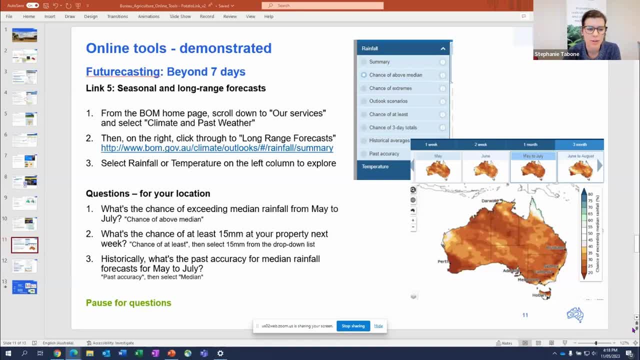 some of the things that they might change in their management and how they might change in their management and how they might change in their management decisions based on the tools that jonathan's just covered around. uh, seven day and and more of the long-term forecasting. uh, thanks, steph. uh, you know, one of the big things around potatoes is harvesting time and being able 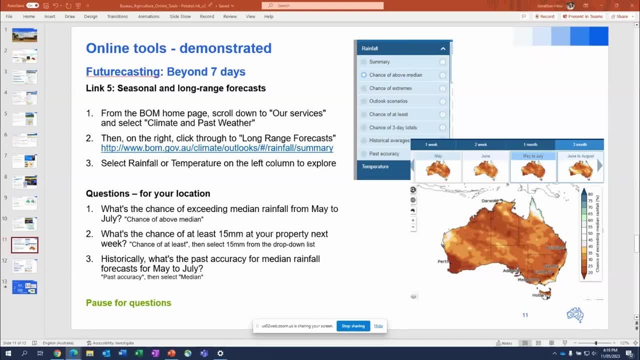 to forecast when you've got rain coming, um, in order to either catch up on your schedule or pause your schedule in in and and wait for conditions to be right. so i think that's going to be a big thing for us to look at. and i think that's going to be a big thing for us to look at. 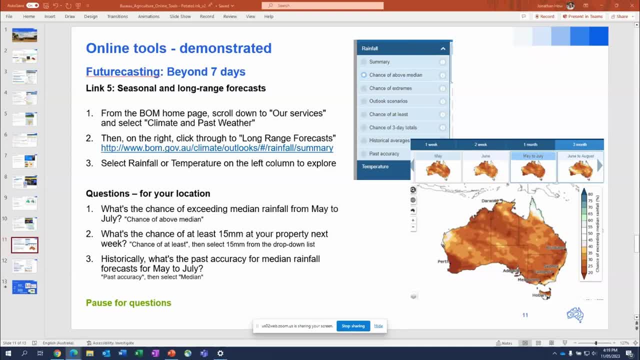 really important um, let alone the issues of spraying um. those kind of things. what, what's it like? what's the best day for me to spray? um. there's a whole lot of things that people would find useful in in this near term and future forecasting um exercise to to really be able to. 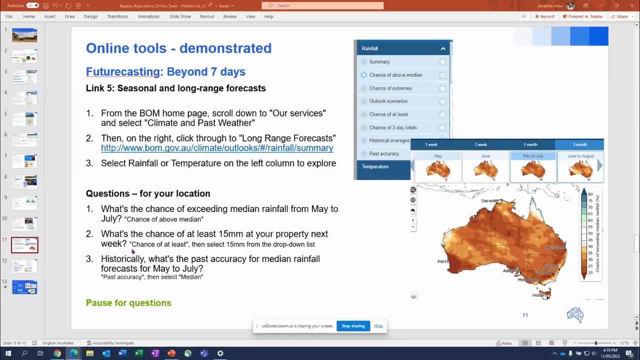 fine-tune their management. um, i agree with the comments around um evapotranspiration. it would be a really good thing to do, and i think that's going to be a really good thing to do, and i think that's going to be a really good thing to do and i think that's going to be a really good thing to. 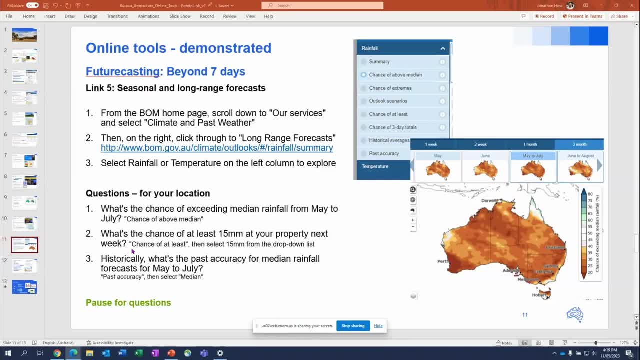 have. there's no doubt about it and most of our potato growers use it in some form in order to forecast their irrigation scheduling. but here's a rough, a rough idea of what's likely. you've got ahead of you and you might be able to guess what um evapotranspiration- your crops likely to face. 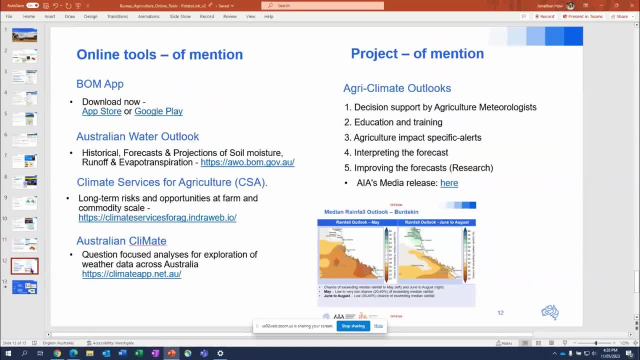 so there are tools within this. yes, it's not a evapotranspiration number, but certainly um will give you a foresight on on those kind of issues that growers could face. i was just going to um add um, i forgot to mention it before. sorry, jono, i didn't want to interrupt you. 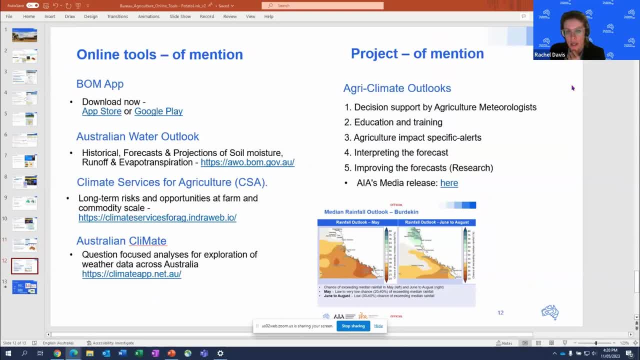 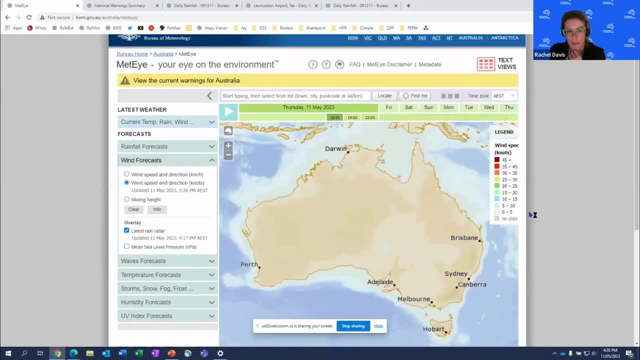 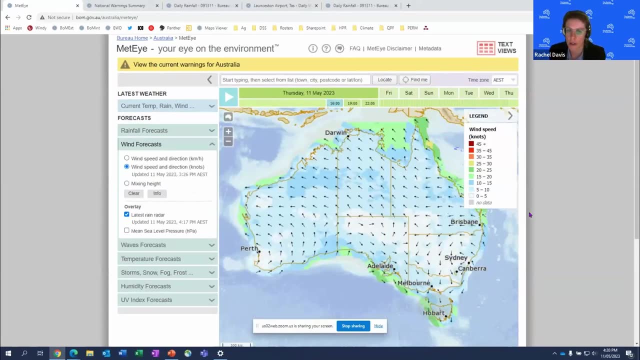 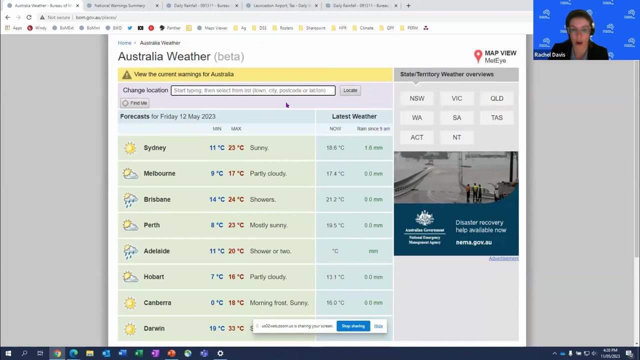 but just back on the metai website, um. there is a lot of data in that site and i know people that um maybe don't have the greatest internet connection or it's struggling to load. you can go into text, view um and get information from there for your location, um and and find people would like to see. 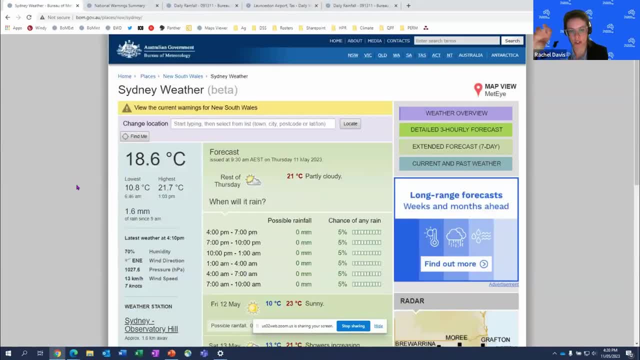 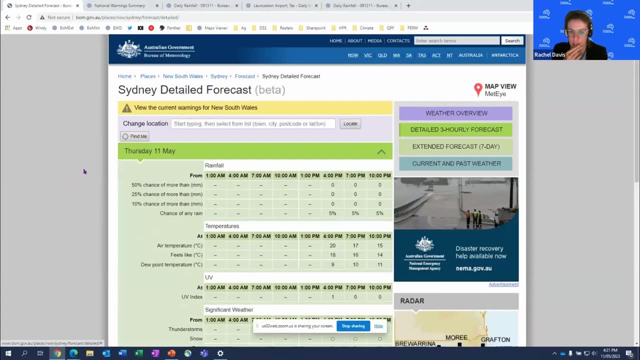 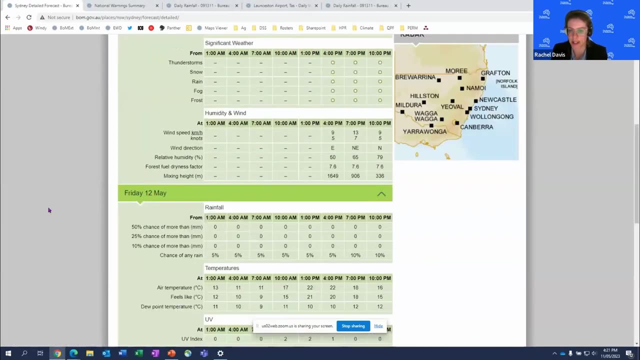 um, like the wind, how it's going to change during the day as well, so you can go to detailed or, um, i think, three at detail, three hourly forecast, yeah, and scroll down and people can see when the wind's likely to pick up and ease. obviously, there's not many hours left in the day, um, the 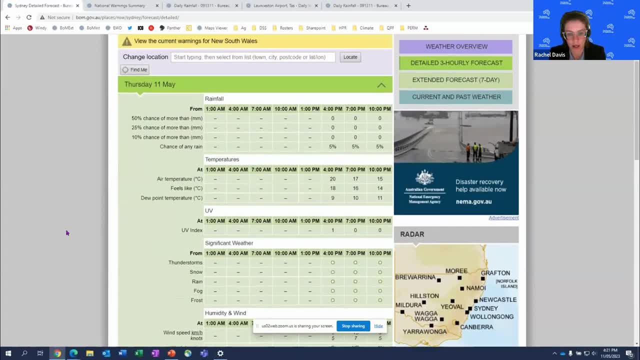 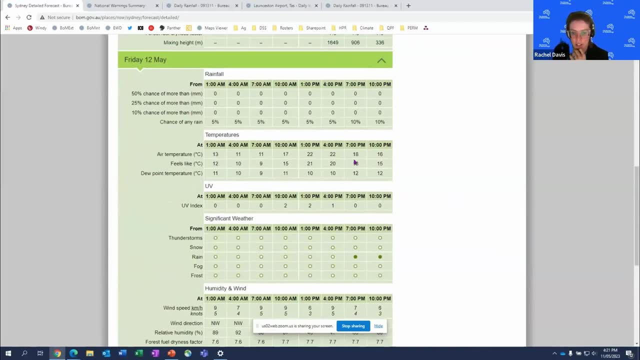 day today but like tomorrow, um, and then you can go to detail three hourly forecast and you can um, you can see that at three in fig in um figures for three hourly and also see you know where their rain dots are for significant weather. so we found people that love the map view and then others that 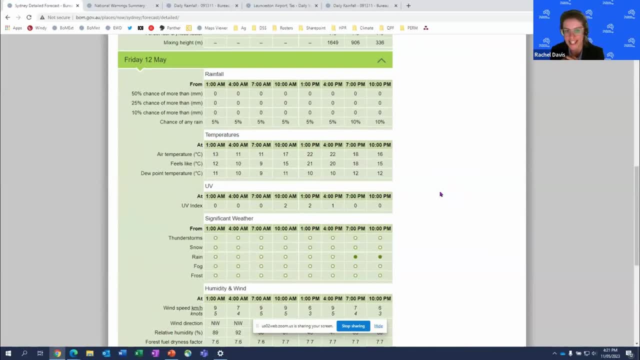 love the text view and then, and also noting potentially internet um issues, just because there is so much um data as you can imagine being loaded and so um, yeah, folk really um get um good value out of the text views as well. i just wanted to add that. 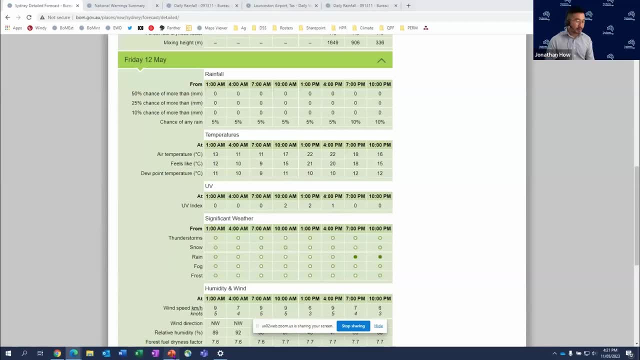 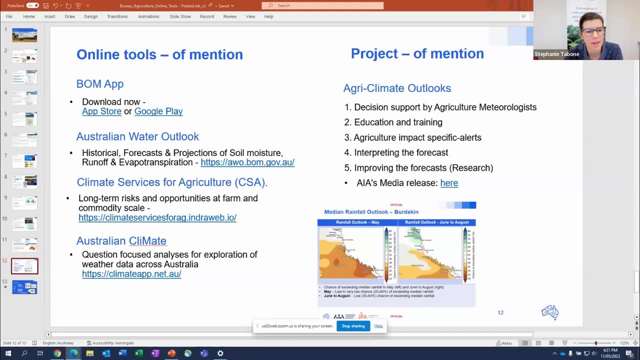 brilliant, it's easy to miss some of the smaller uh functionalities of the tools that you have available. and um, we're almost at time now, but jono is just going to give a brief overview of some other tools that are worth mentioning and we don't have enough time to cover today. 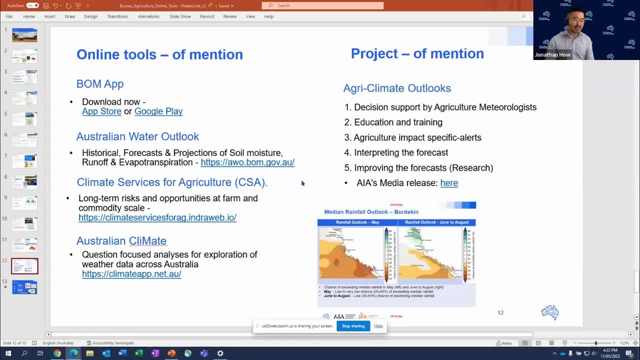 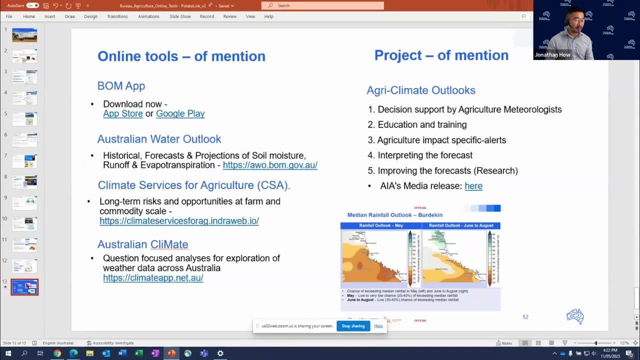 yeah, just some links here, you can feel free. there's a australian water outlook, cs climate services in australian climate, and then we've got just as much information range of mentioning this agri-climate outlooks projects. um so yeah, that's um pretty much it for me. hopefully i managed to get something. 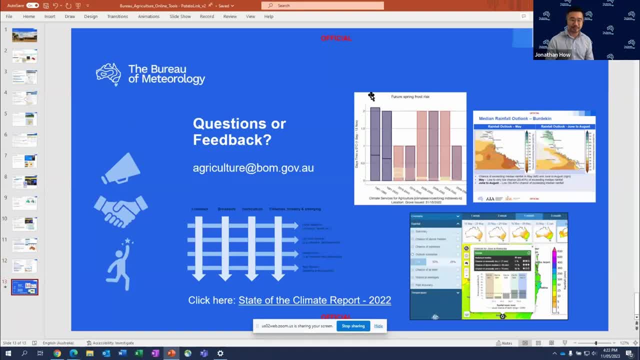 out of it, but you feel free to go back and work through the worksheet again. thanks for that, and we'll also, like i said earlier, we'll upload the slides with the links so you can access it at a later date as well. um, so that concludes the formalities of the training. 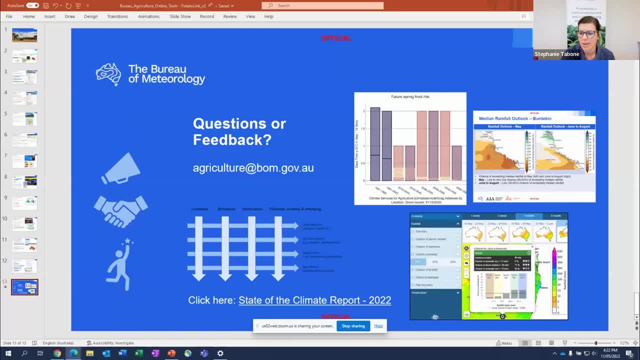 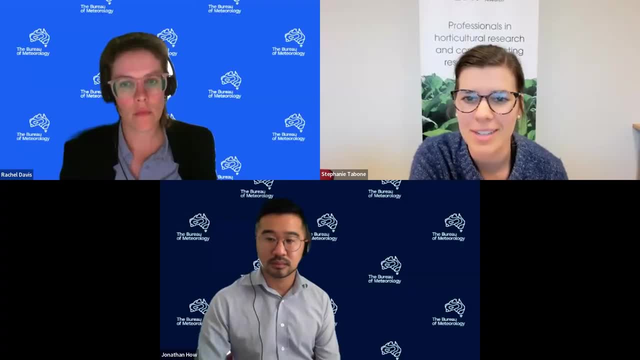 today. i just wanted to open it up, uh, for anybody to come off mute or pop any questions or anything in the chat. it's a really valuable opportunity to have a senior meteorologist on a call with us. that you know. john has explained a lot about how the models work, but if there are any other, 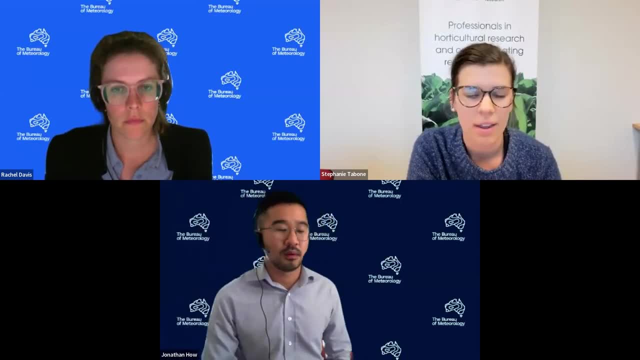 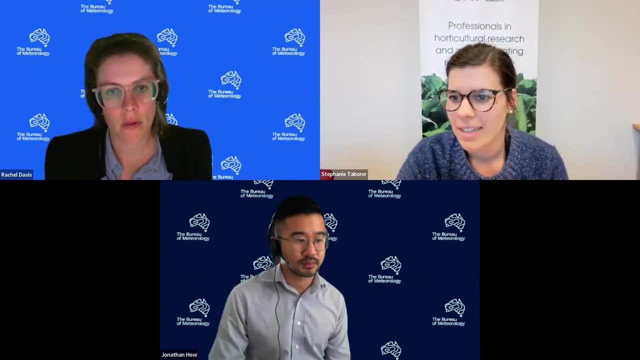 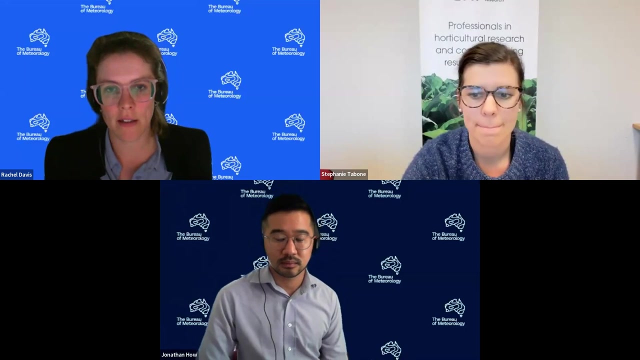 questions about tools that you've used that we either haven't covered today or, potentially, ones that we have that you have any questions about. now is the time. well, people gather their thoughts. um. just going to add that we do have some late mail coming in, that um, potato, potato. 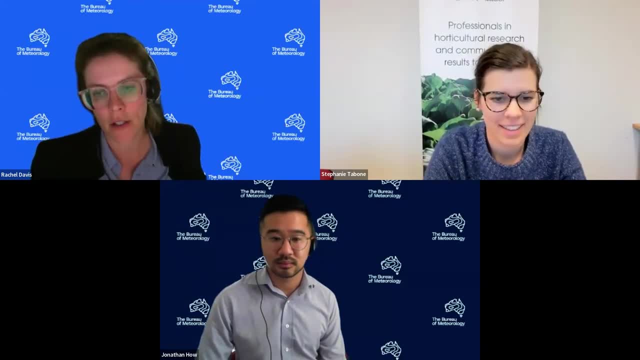 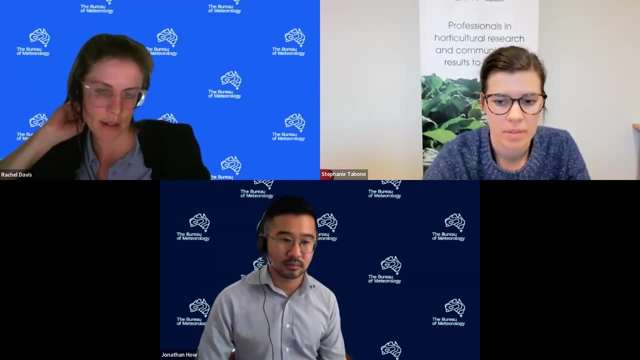 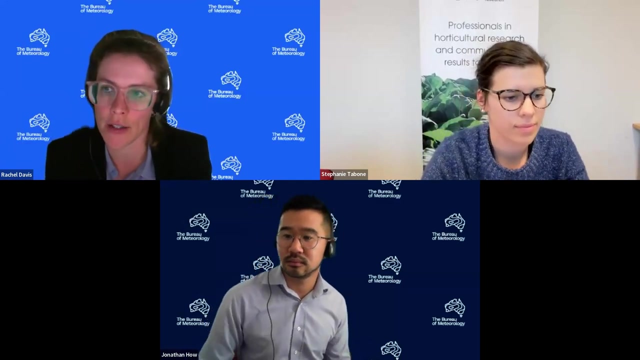 commodity as a commodity is actually available on the climate services for agriculture platform. um, just one. we didn't um display that tool today, but, um, yeah, it was on the of mention um page and so, uh, yeah, it's a great resource and still in development. but, yeah, you can actually 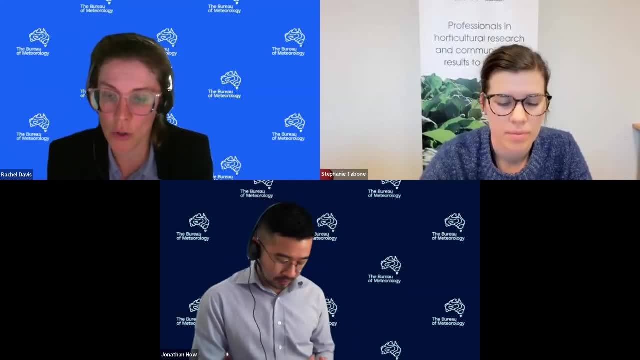 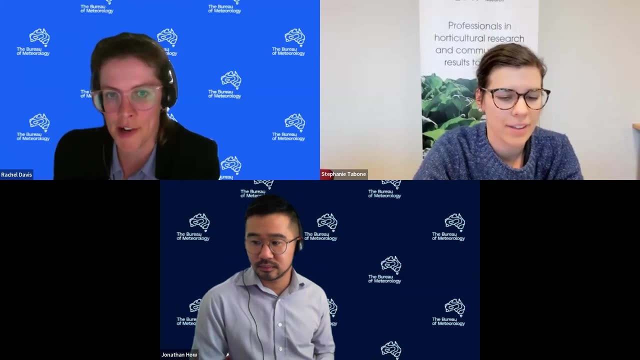 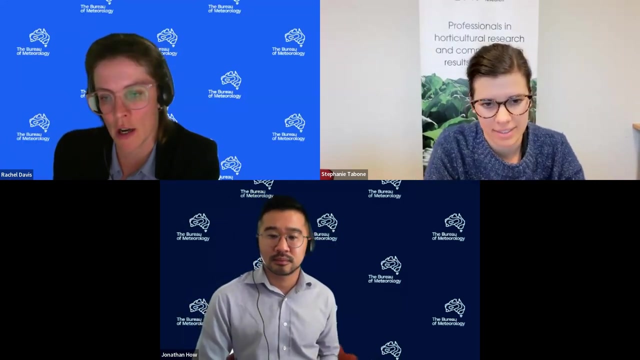 choose um potatoes for um long-term decision making, and then all the historical data is there as well. so, um, we encourage everyone in their spare time to have a look at that, and also, while i've got the microphone just to spruce our agriculture at the omgovau email address, um, we've got a. 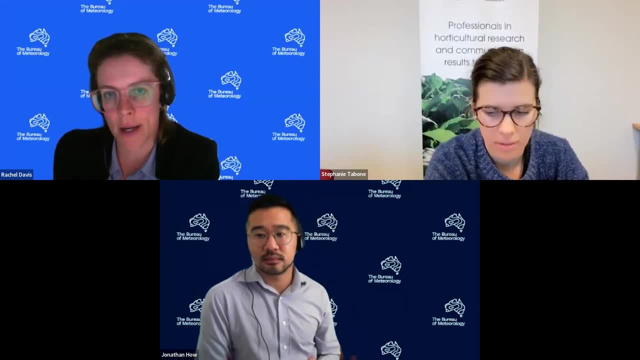 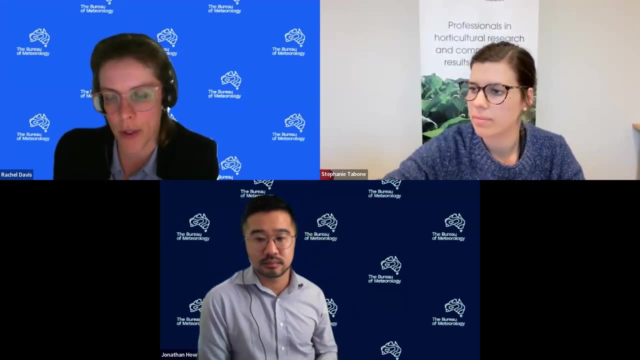 whole team which you've heard about, um behind, um the scenes in agriculture and um customer facing roles as well, that we're keen to hear from people and keen to help um where we can and delve deeper as well into anything that may have been talked about today that you want to know more info about. 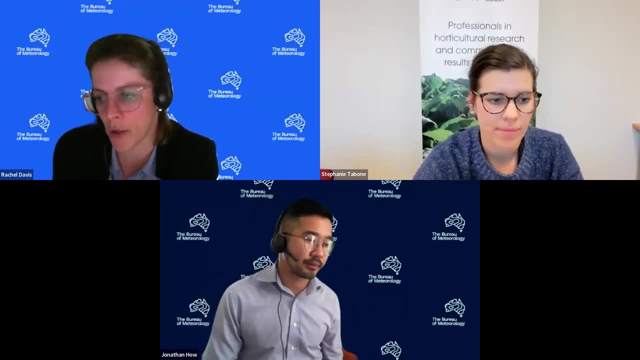 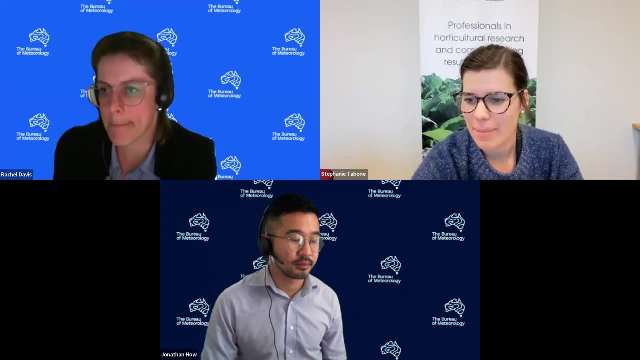 or you need more help with. so, um, yeah, agriculture at bimgovau. and thanks, stephanie, for just dropping that in the chat. no worries, okay, um, maybe just to conclude the session, if you guys wouldn't mind popping in the chat what, what it is that you're going to use moving forward, if there's anything. 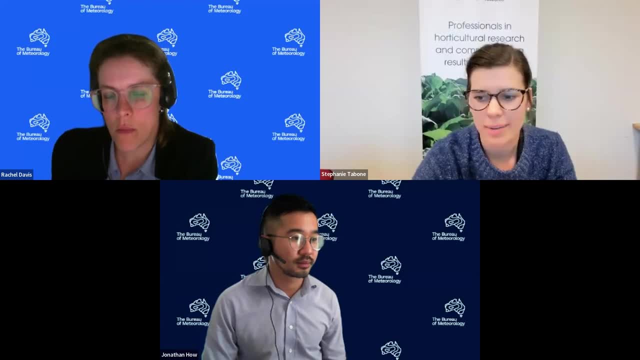 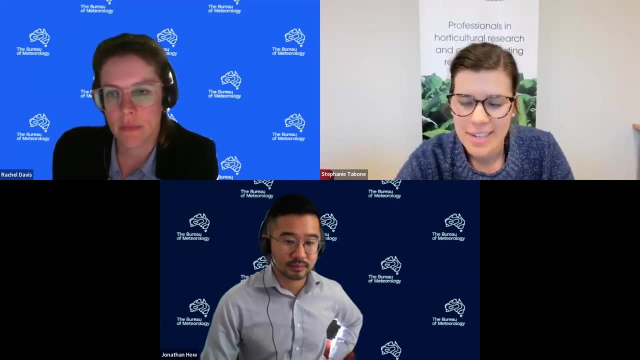 you've learned or how you're going to use it in the future. i'd love to hear from you about that. we're going to apply the tools. um, just any comments on how you're going to use the information that we've gone through today? um, just while folk are doing that, i might just also share my screen on. 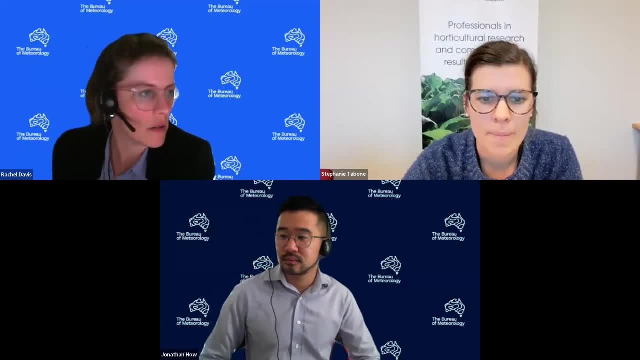 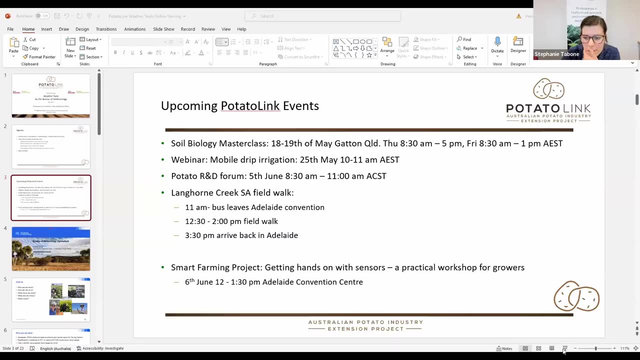 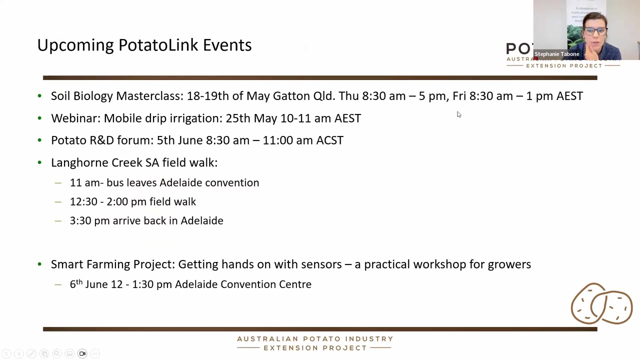 some upcoming events we have for the potato link project. sorry, bear with me. so we've got a soil biology master class coming up in gatton on the 18th and 19th of march, so we're. so. it's a two-day workshop which will be very interactive and involve a field visit and a lab. 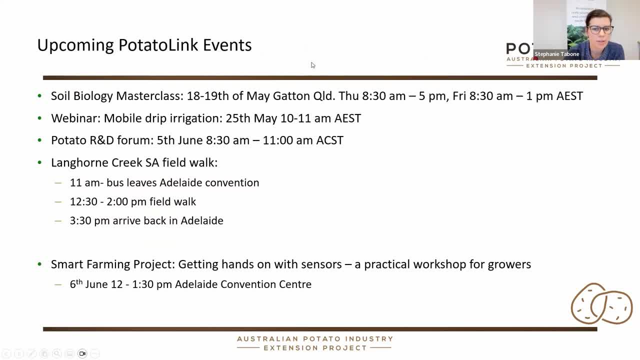 tour of the Medigen lab in Gatton. so if you're interested it's best to register so that we we can accommodate for you there. We have a webinar coming up on the 25th of May on mobile drip irrigation and that will be from 10 till 11am and we've got a potato link R&D. 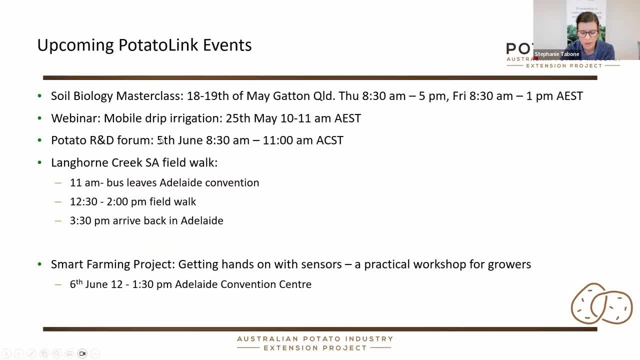 forum where we'll bring to you the latest in research and R&D in the potato industry, but also in other segments, thinking sort of blue sky research that can be applied in potatoes, looking at a range of different topics like precision agriculture, variable rate mapping, what viruses? 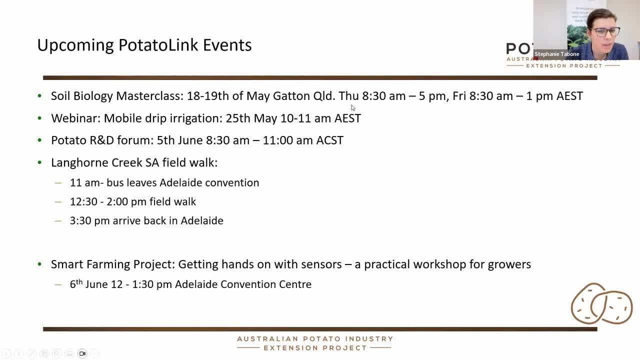 are on the horizon or being experienced at the moment in Australia and we've got, in association with that, a Langhorne Creek field walk straight after the R&D forum, based obviously in South Australia, and we, because this, both of these events, will be sort of linked with Hort Connections as we have a lot of people traveling. 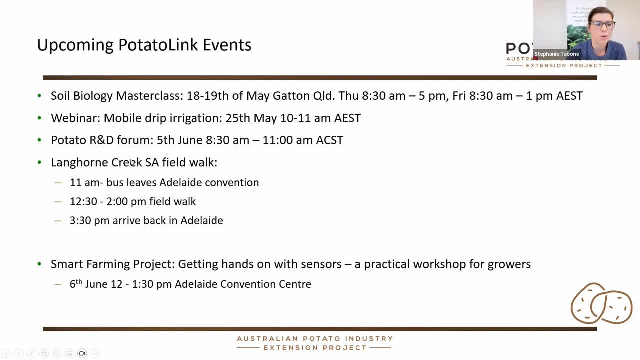 down for the event. we have arranged a bus from the R&D forum straight to the field walk for anyone who would be interested in attending both, which will arrive back in Adelaide in time for the launch of Hort Connections. And then, lastly, this is not a potato link event, but the Smart Farming. 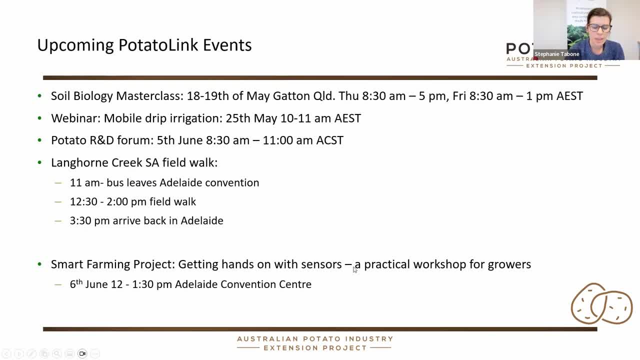 Project are doing a workshop following the R&D forum, based on sensors and practicalities around using sensors, and this is predominantly aimed towards growers, so one of the representatives from the project will be talking at the R&D forum and it's an opportunity if you are interested in hearing more. 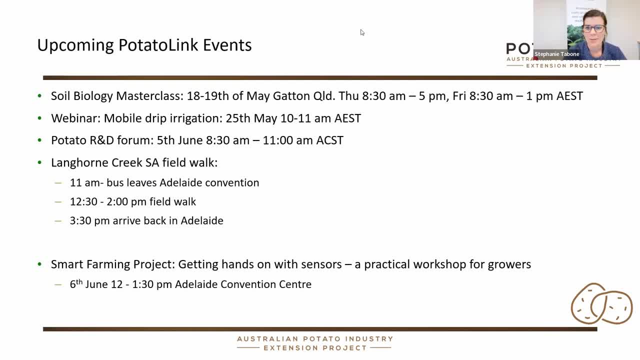 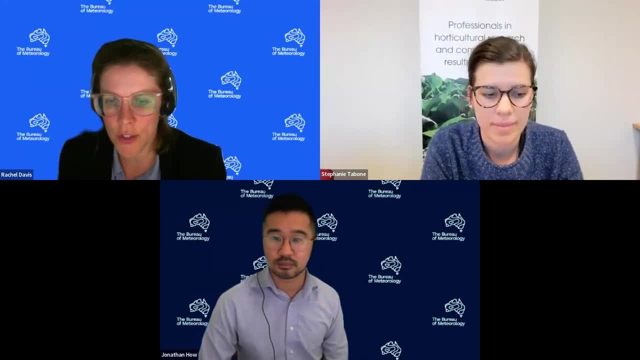 to tune into the workshop. So yeah, that was all I was going to add. And, Steph, do you, does AHR have a stand at Hort Connections? Correct? yes, So we do have a stand. a few of us from the potato link project will be at Hort Connections over the